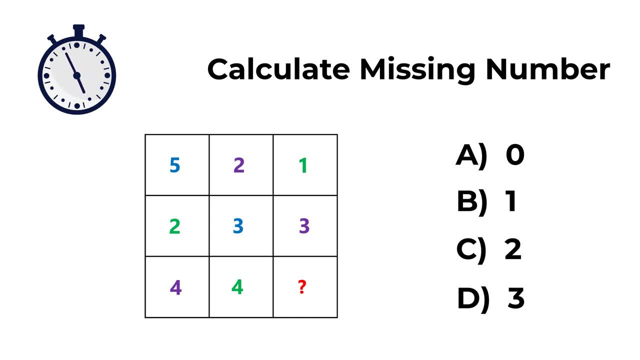 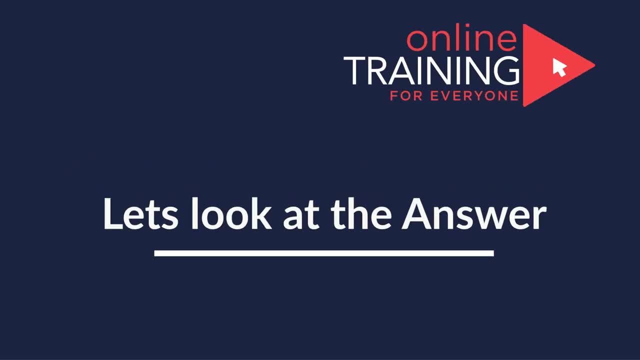 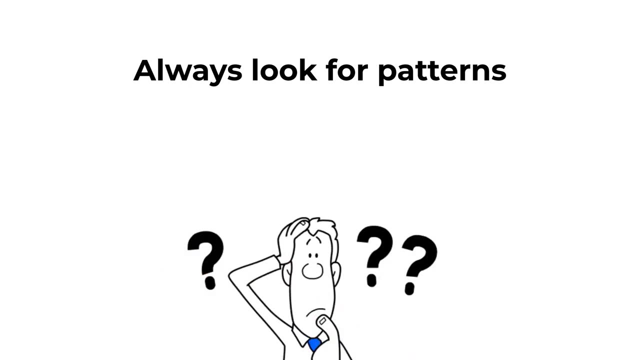 solution. Do you see the answer? Let's continue to see how we can solve this challenge and get to the correct solution together. As usual. my advice to you: always: look for patterns. In this particular case, we need to look at the patterns inside the rows and then inside the columns. Let's look at the first two. 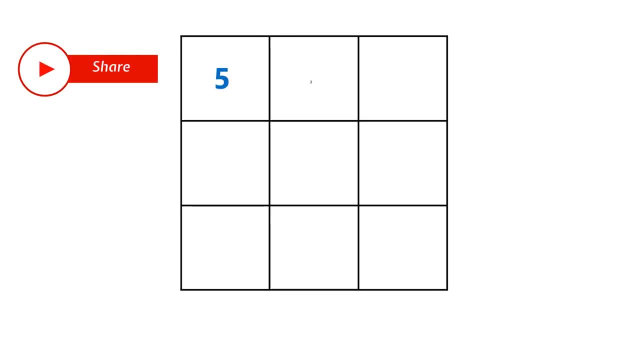 rows to see if we can get the pattern. The sum of 5 plus 2 plus 1 equals to 8.. The sum of 2 plus 3 plus 3 also equals to 8.. So there might be a pattern. Let's look if there is a pattern for. 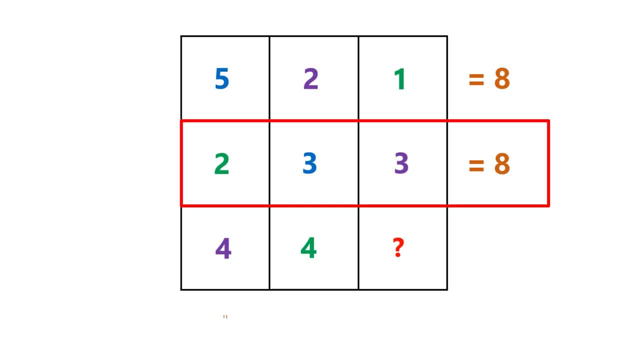 the columns that have full sets of numbers. 5 plus 2 plus 4 equals 11.. 2 plus 3 plus 4 equals 9.. So there is no pattern. In this case we can relatively simply use the pattern from the rows. This would allow us to calculate the third. 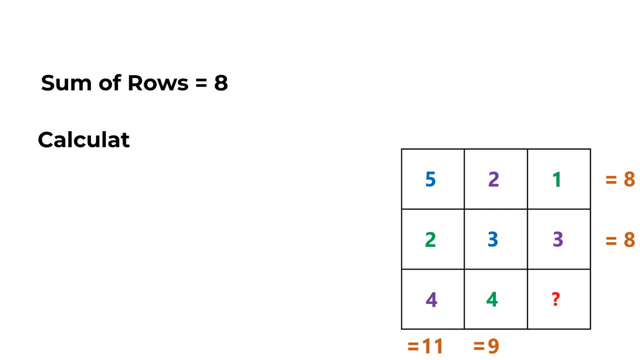 row. If we know that the sum should be 8, we can assume that the 4 plus 4 plus question mark, which would be representing the missing number, would be equal to 8.. So the missing number would be equal to 0.. The correct choice here is choice A, 0.. Hopefully you've nailed it. 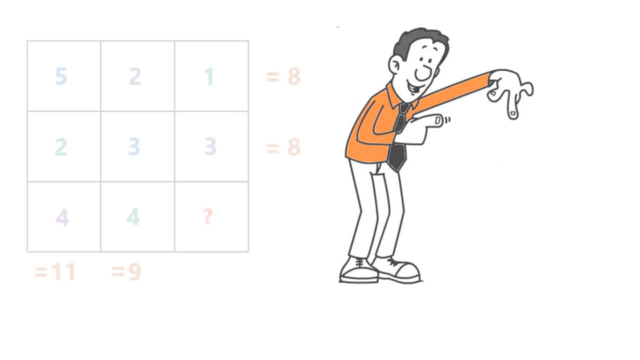 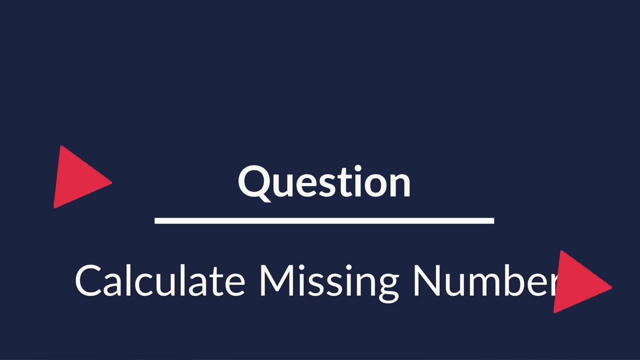 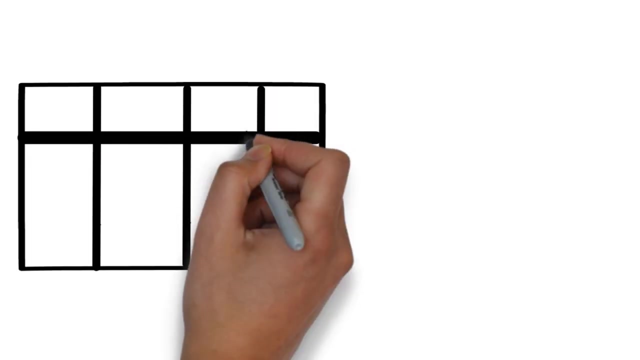 Take this question on your own and now know how to answer similar problems on the test. Here's one of my favorite questions because it is very frequently used on the test. You're presented with the matrix 4 by 3 matrix. Each cell in the matrix has numbers. For example: 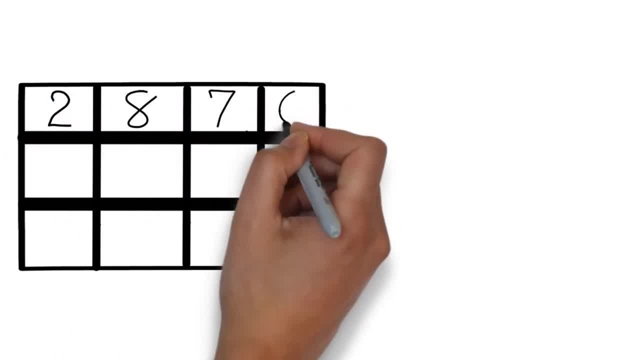 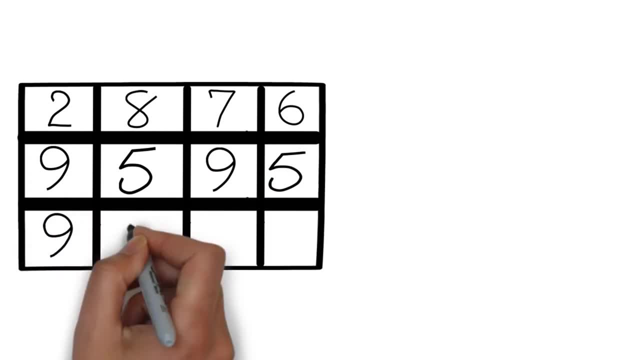 first row in the matrix has numbers 2,, 8,, 7, and 6.. Second row has numbers 9,, 5,, 9, 5.. And the third row has numbers 9,, 7,, 4.. And one number in the bottom right corner is missing, And this is: 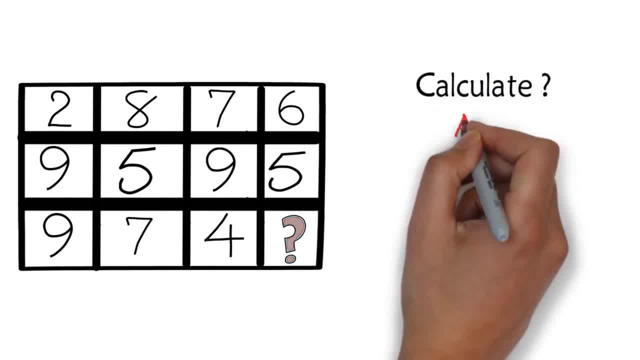 exactly what you need to calculate. You can choose from one of four different choices: Choice A: 5.. Choice B: 7.. Choice C: 9. And then choice D: 11.. Do you think you can come up with the answer? 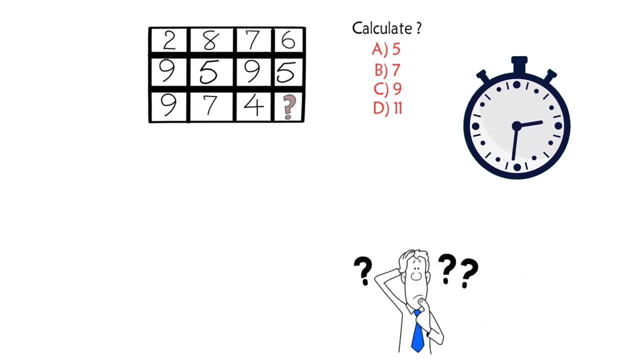 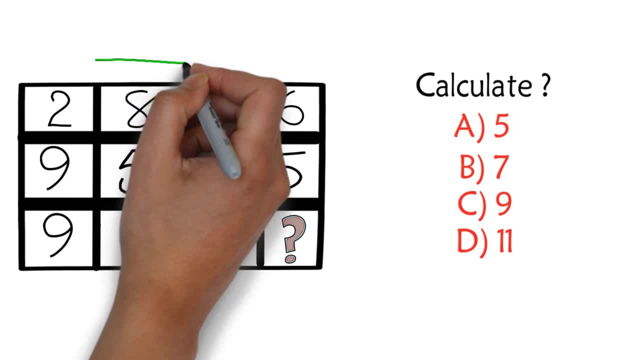 Give yourself 5 to 10 seconds. This is about as much time as you will get on the test. Let's continue to see how we can get to the correct answer together. The key to solve this problem is to determine the pattern, And the pattern either can be in the rows. 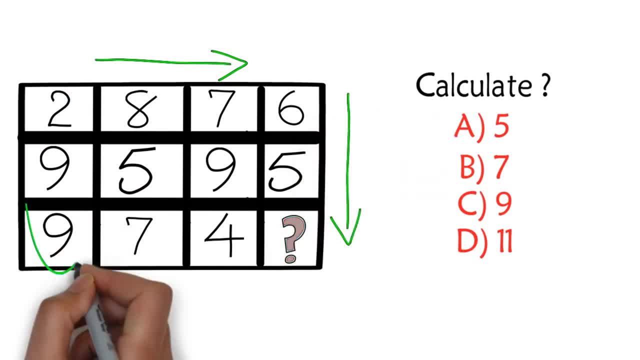 or in columns. In this particular case. let's check the columns first, And then what you see is that each column adds up to the value of 20.. For example, 2 plus 9 plus 9 is 20.. 8 plus 5 plus. 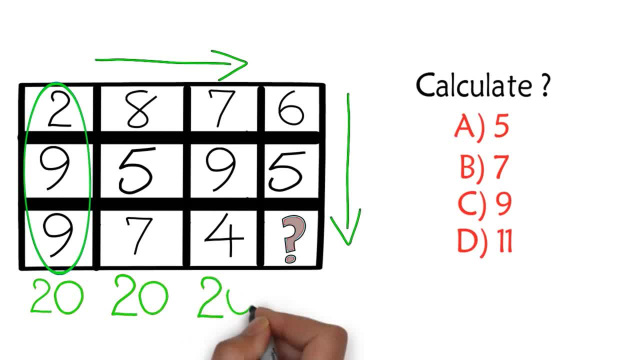 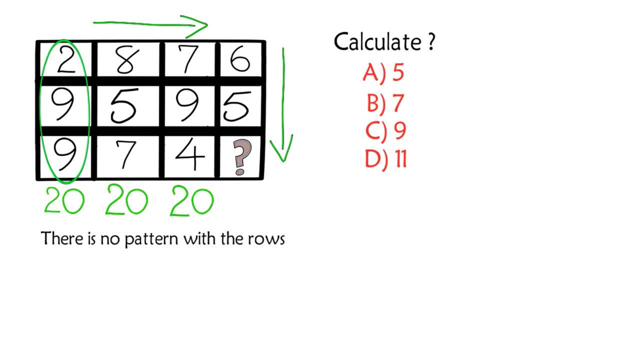 7 is 20.. 7 plus 9 plus 4 is 20 as well. We also want to check if there is a pattern with the rows. And there is no problem, Because the first row adds up to 23.. 2 plus 8 plus 7 plus 6 equals 23.. And the second row? 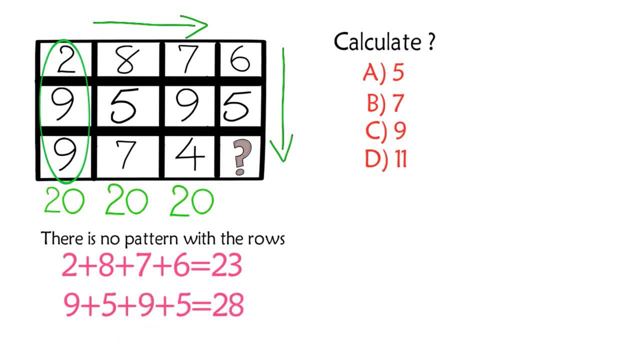 adds up to 28.. 9 plus 5 plus 9 plus 5 equals 28.. So there is no pattern. Based on this information, you can calculate the missing value in the fourth column: 6 plus 5 plus question mark equals 20.. So the answer is C 9.. This is the missing value. 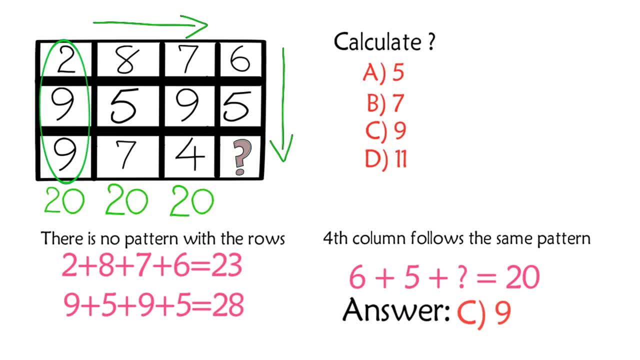 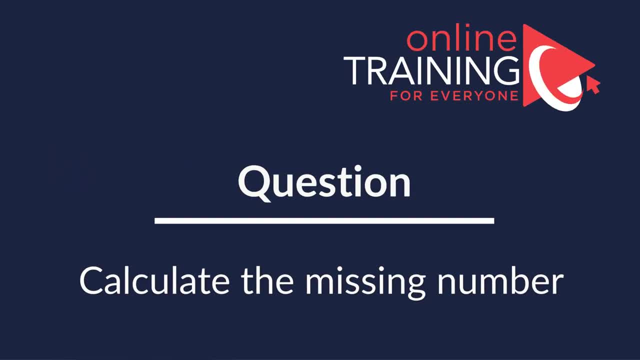 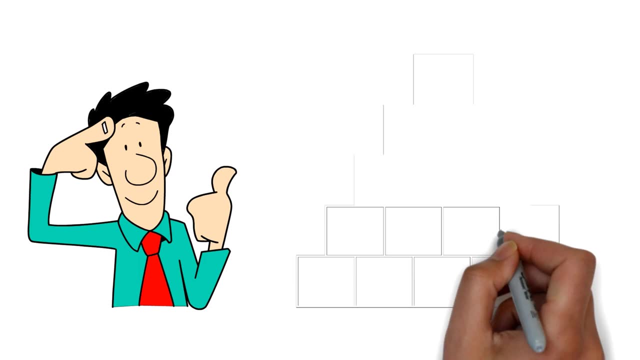 Hopefully you figured it out and now know how to answer similar problems on the test. Here's one of my favorite questions, And it is my favorite because it is so unusual. You are presented with the pyramid. Pyramid contains five different layers. If we go from 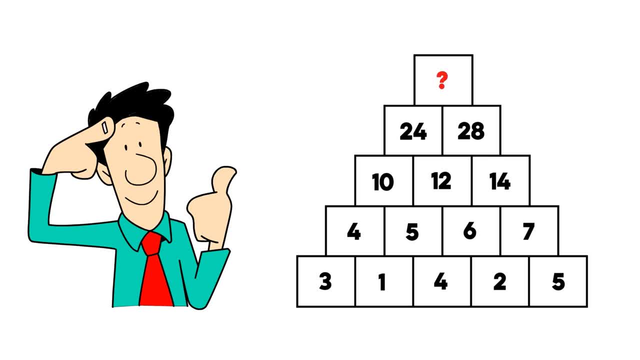 the top to bottom, you have a question mark. This is the number that you need to uncover. The next layer contains numbers 24 and 28.. Layer below this contains numbers 10,, 12 and 14.. Next layer has 4,, 5,, 6 and 7.. And the last layer has numbers 3,, 1,, 4,, 2 and 5.. 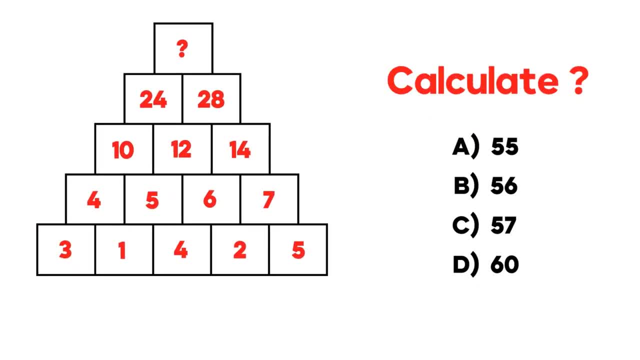 You are presented with four different choices for the missing number: Choice A: 55.. Choice B: 56.. Choice C: 57. And choice D: 60.. Do you see the answer? You will be surprised how easy it is to answer. You will be surprised how easy it is to answer. 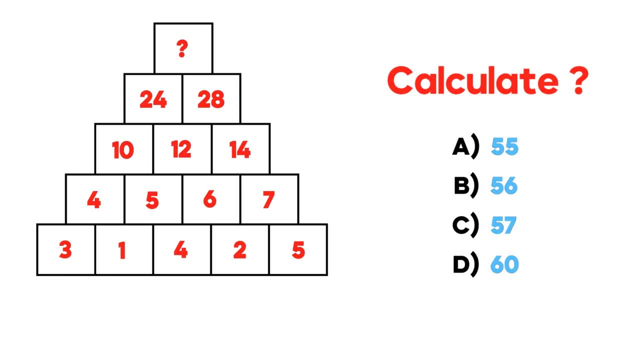 You will be surprised how simple it is to answer. You will be surprised how simple it is to answer. get to the answer. when we go to the next step. give yourself 5, 10, maybe 15 seconds to see if you can calculate and get to the correct answer. did you figure it out? let's continue and see how. 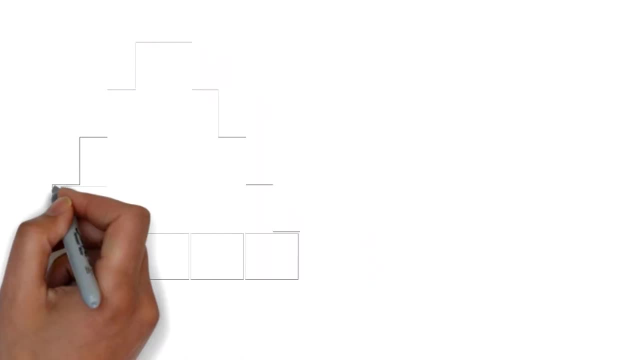 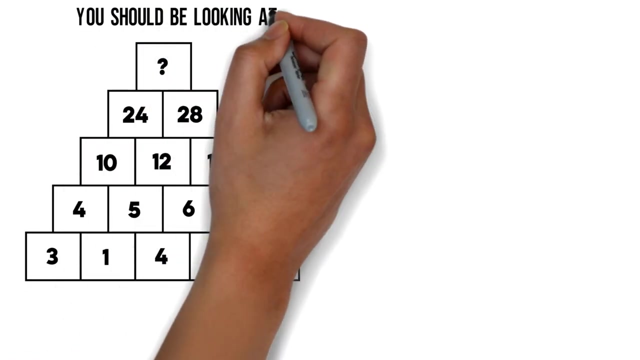 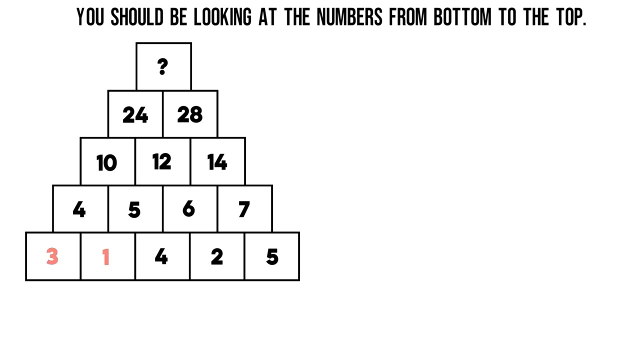 we can get to the correct solution together. well, here, to be honest, i try to trick you. i went in describing numbers from top to bottom, but in reality you should be looking at the numbers from bottom to the top. if we start from the bottom row, for example with numbers three and one, you see. 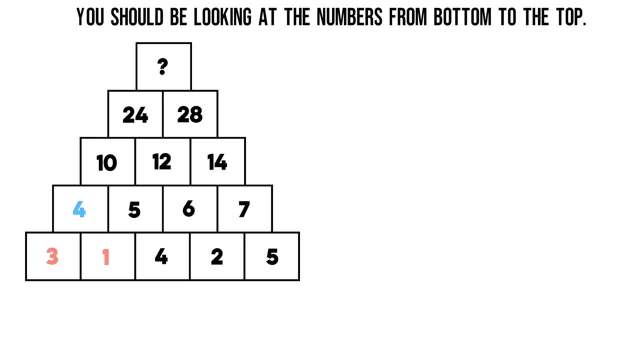 that the sum of three and one will add up to four. but then it gets trickier. if we go from the second row to the third row, you see that the four and five does not necessarily add up in ten. four and five adds up in nine, and then you need to increment it by one. if you go to the next layer, you need to. 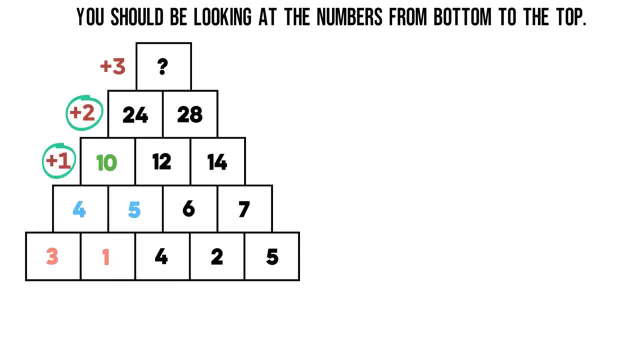 increment it by two and then in the final row you need to increment it by three. so the correct answer here is choice 55.. let's recap, starting with the bottom row, you see that the sum of three and one in the bottom row, the sum of two squares, results in the number in the next row. for example, two plus. 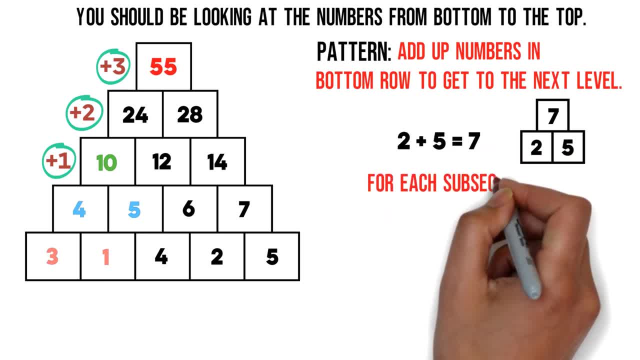 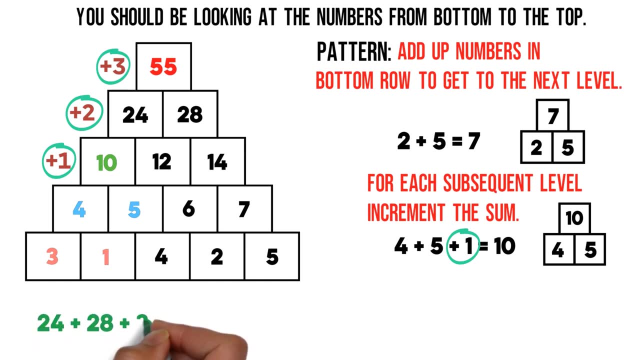 five equals seven. however, as each level continues, the sum increases by one. for example, four plus five. we need to increment and add one to get to ten. so the answer is calculated by adding up 24 plus 28 plus 3, which would be equal to 52 plus 3 and would be equal to 55.. 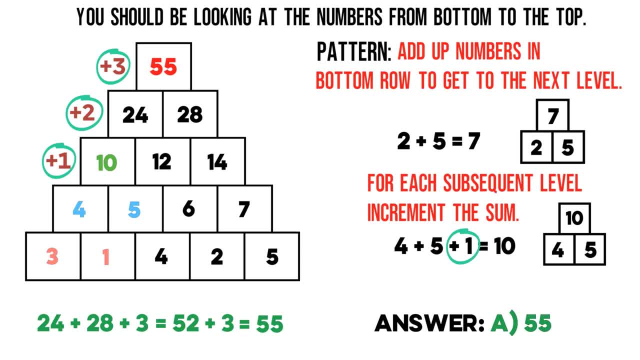 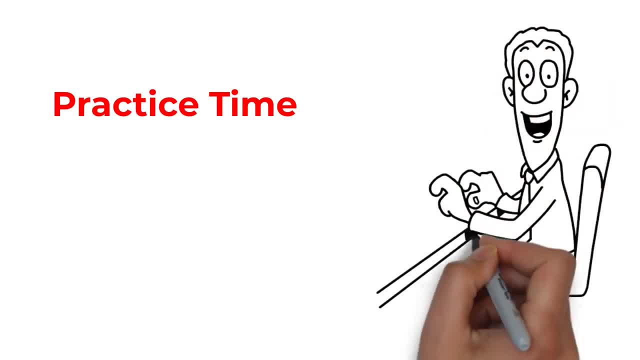 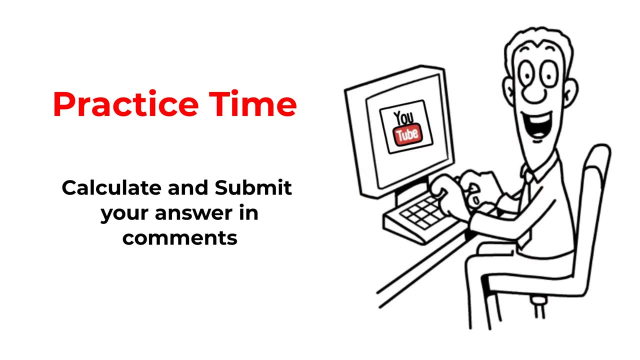 the correct answer here is choice a 55.. hopefully you've nailed this question and now know how to answer similar problems on the test. and now here's the question for you to try. if you can calculate the answer, please post it in the comments section of this video so i can give you the grade. we have two projects and to complete. 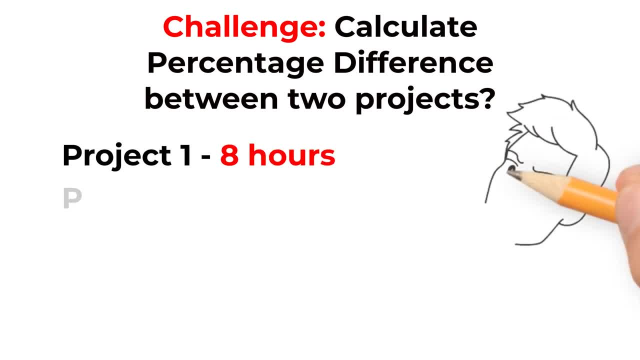 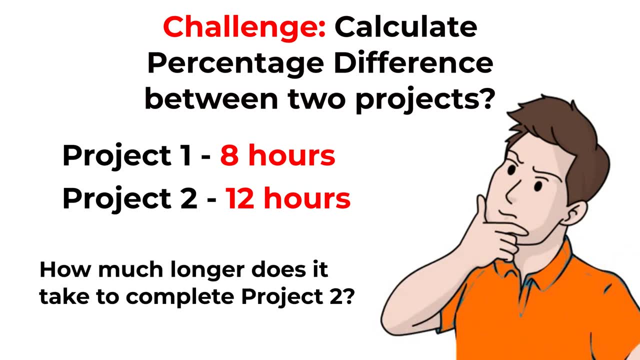 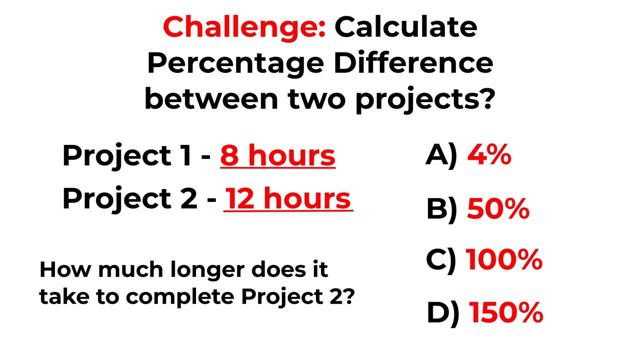 project one it takes eight hours and to complete project two it takes 12 hours. so how much longer in percentages it takes to complete project one versus project two? you have four different choices: choice a- four percent, choice b- 50, choice c- 100 and choice d- 150. can you calculate the answer? 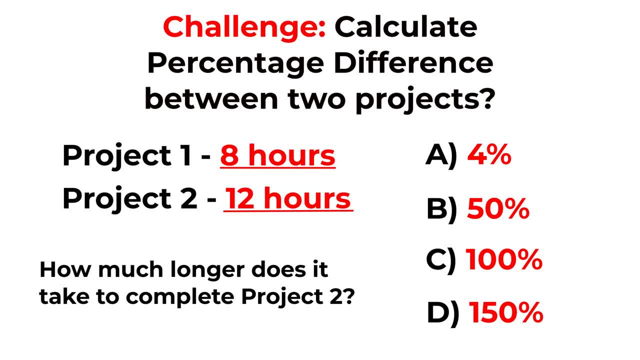 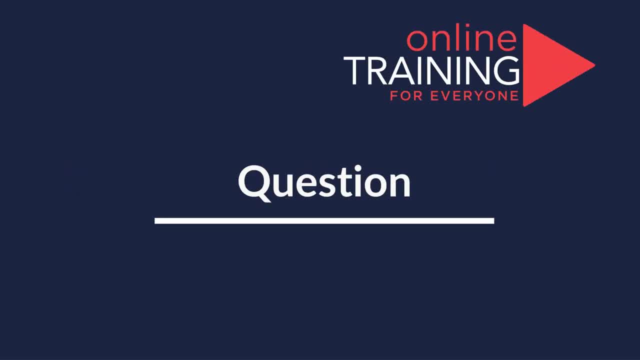 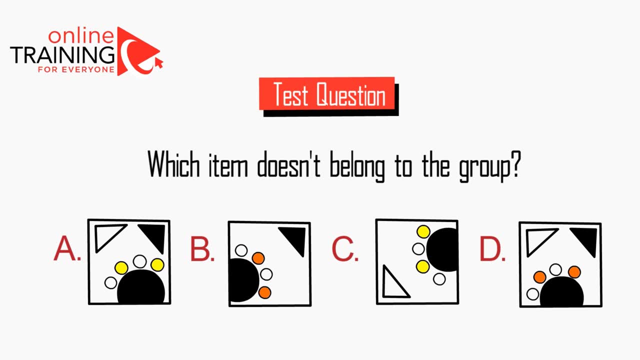 please make sure to post it in the comment section of this video so i can give you the grade. thanks for participating and good luck. the types of questions you are looking at is very frequently used on the test. Typically, you are being asked to determine the item which does not. 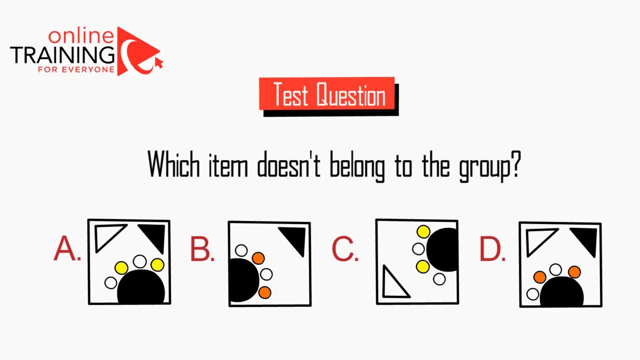 belong to the group and you are presented with multiple items. In our choice, we have choices A, B, C and D. Each item is represented as a square which contains multiple different items inside, and you need to determine the item which does not belong to this particular pattern or sequence. 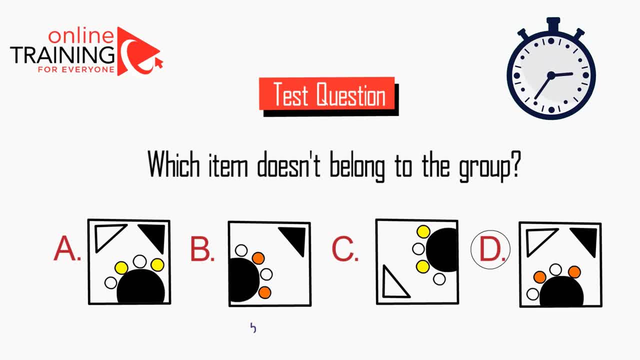 Do you see the answer? Please take a look to see if you can come up with the solution. Give yourself 5 to 10 seconds, maybe 10 to 20 seconds, to see if you can come up with the answer. Did you? 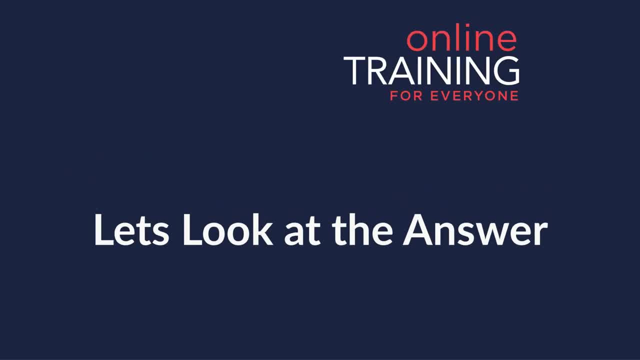 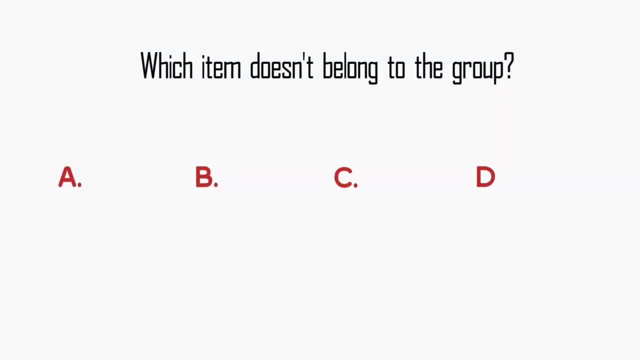 figure it out. Let's continue to see how we can go and get to the correct solution together. As you might have figured out by now, there is always a pattern that you need to detect to answer these types of questions correctly, And a lot of times there are items that are designed to. 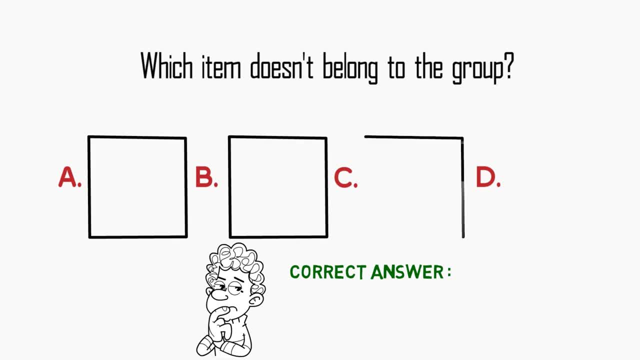 confuse you. So let me first walk you through the items that are designed to confuse you. You have small circles, and there are four small circles in each of the squares, And these small circles do not have any patterns. We also have triangles. Some squares have two triangles. 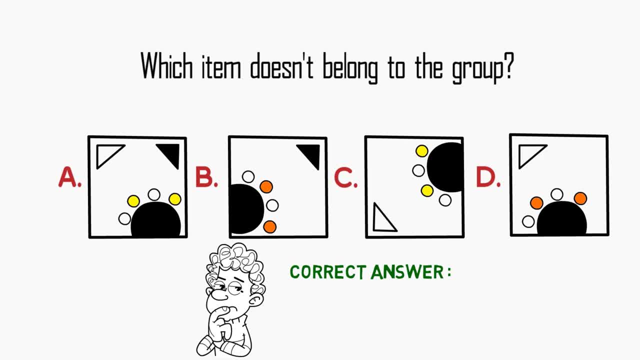 and some squares only have one. But there is no pattern here. The pattern is actually defined by the half-circle And, as you can see, all half-circles are attached to the corners of the square. You see this in the shapes A, B and C, But in shape D- half-circle. 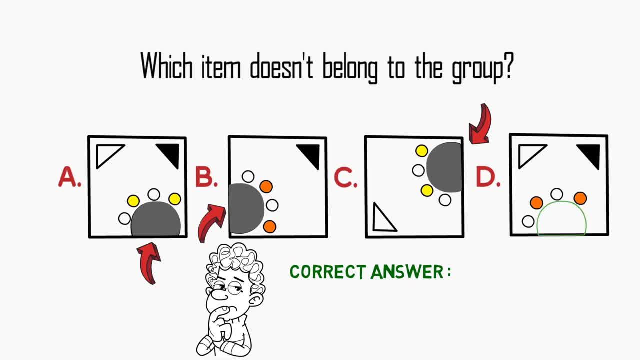 is placed in a different location. It is in the bottom middle of the square. This is why the item that doesn't belong to the group is the choice D, So the correct answer here is choice D. Let's recap: The pattern here is that all half-circles. 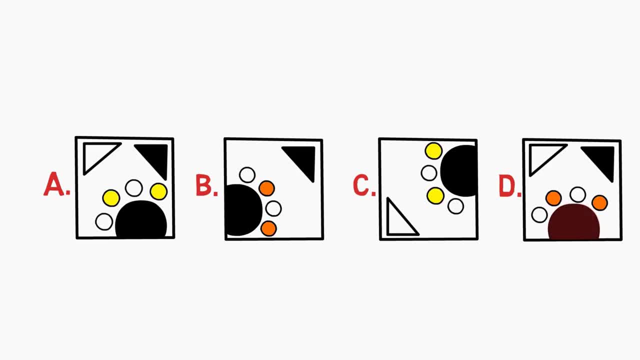 are attached to the corners of the square, But the half-circle in shape D is placed in a different place than the others. The half circle there is in the lower part of the square. This is why the correct answer here is choice D. Hopefully you've nailed this question. 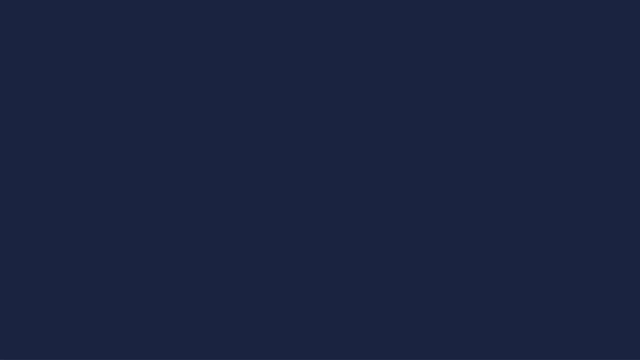 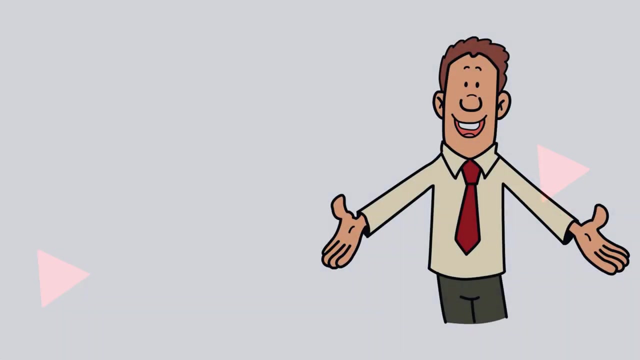 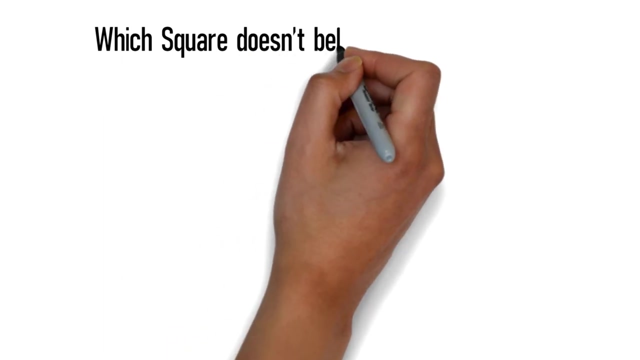 and now know how to answer similar problems on the test. I'm excited to take advantage of the opportunity and share with you how to solve these types of problems on the test. Typically, when you get a problem, you need to determine which object does not belong to the group. In this particular case, you need to determine which square doesn't. 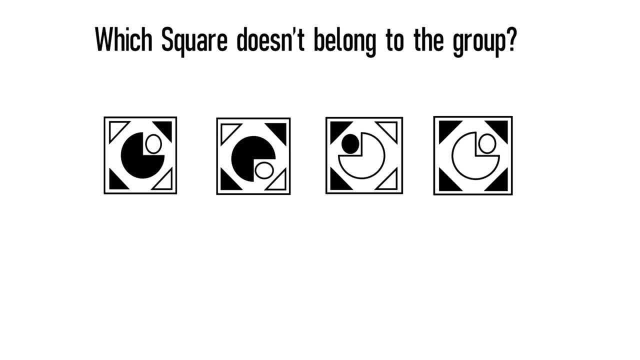 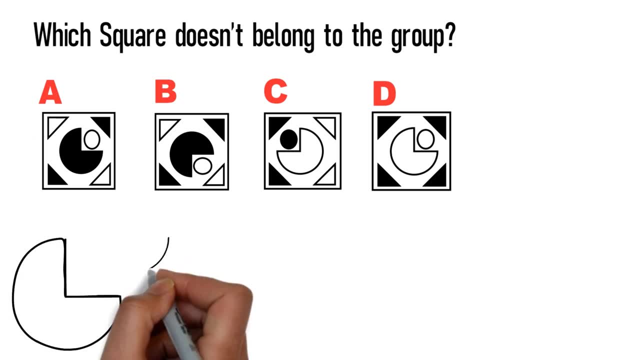 belong to the group. You're presented with four different squares, Choices A, B, C and D. Each square contains two circles inside. In the large circle, quarter of each circle is missing and instead replaced with the small circle. All squares also have triangles in the corner. 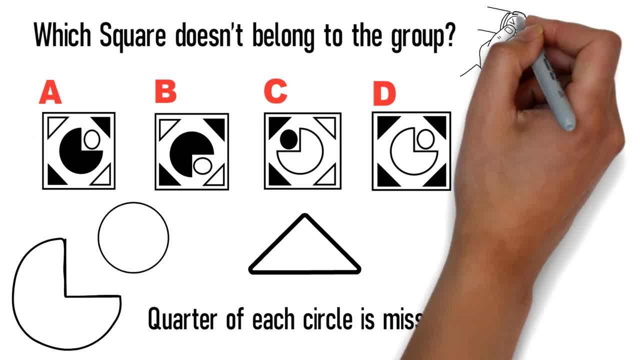 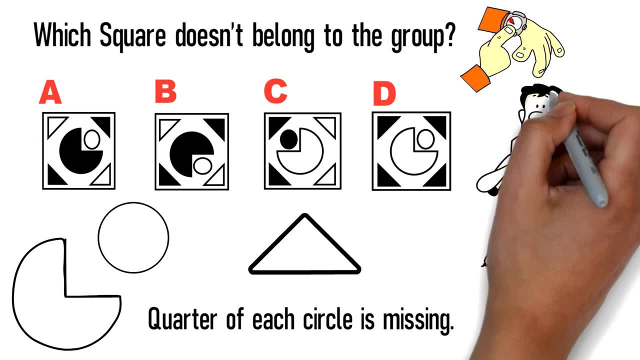 Give yourself a chance to solve this problem. Give yourself 5 to 10 seconds to see if you can come up with the answer. Do you see the answer? Let's continue to see how we can solve this challenge and get to the correct solution. 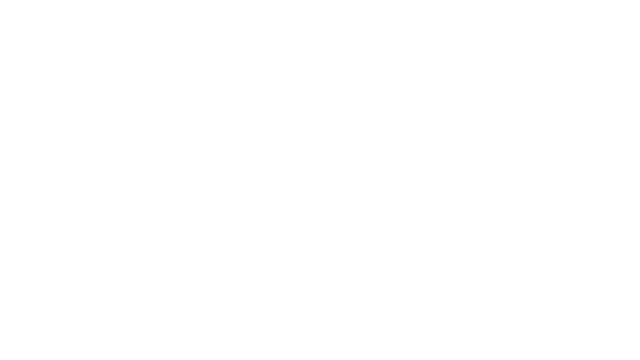 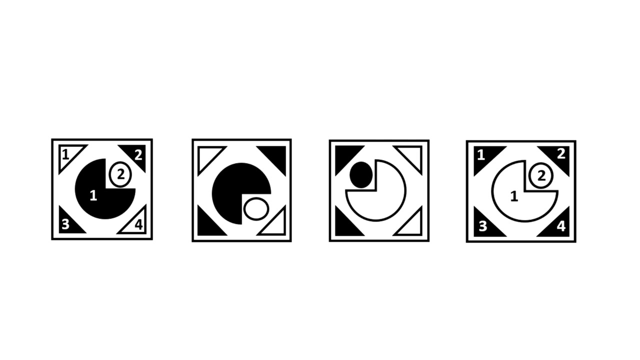 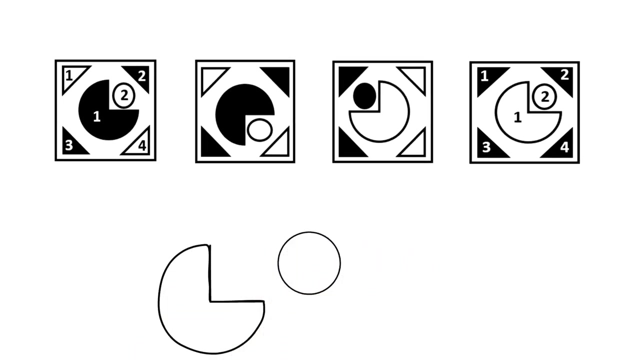 together. The key to solving this challenge is to detect the pattern. This is the skill that you need to develop to be successful in the test, Because there are two shapes here present in this question: triangles and circles. you should try to detect the pattern among triangles and 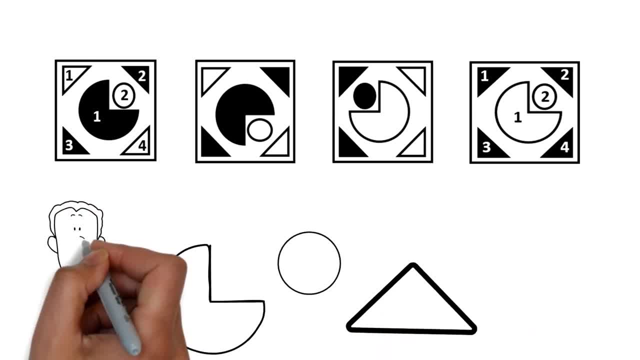 then among circles You should try to detect the pattern among triangles and then among circles You have to detect whether there are triangles. In this particular question there is only one pattern – pattern of the triangles. but there are some sophisticated questions in the test which might include patterns for both shapes In this particular 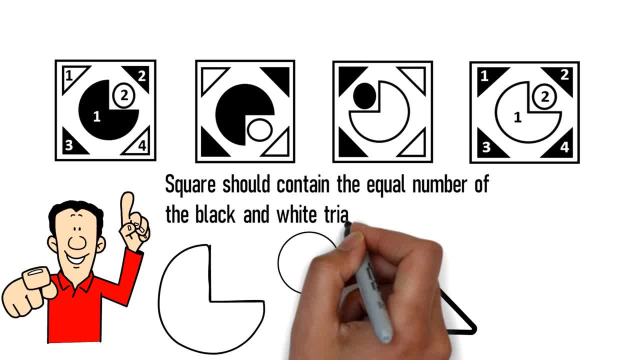 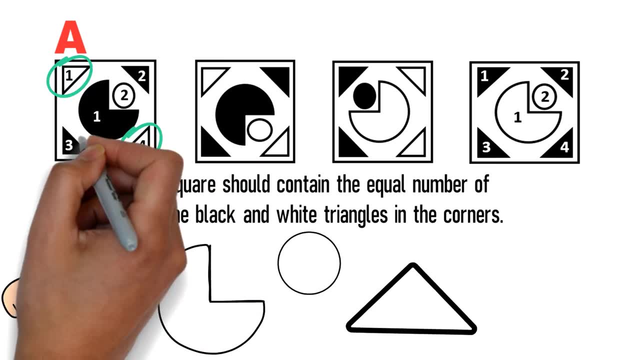 case, the pattern is that a square should contain the equal number of black and white triangles in the corners, Triangles in the square, A position diagonally across each other, located in the upper left corner and in the bottom right corner, And black triangles are located in 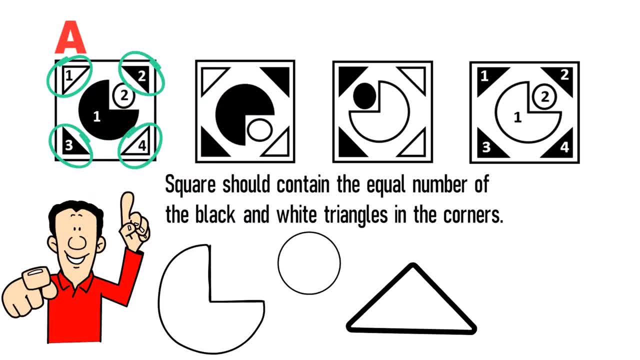 the bottom left corner and in the upper right corner. You can see that the same pattern exists in the shape B, two white triangles and then two black triangles, And in the shape C, two black triangles on the left and two white triangles on the right. But if we look at the choice D, 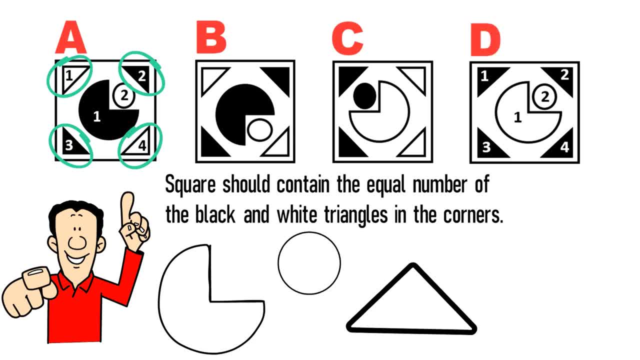 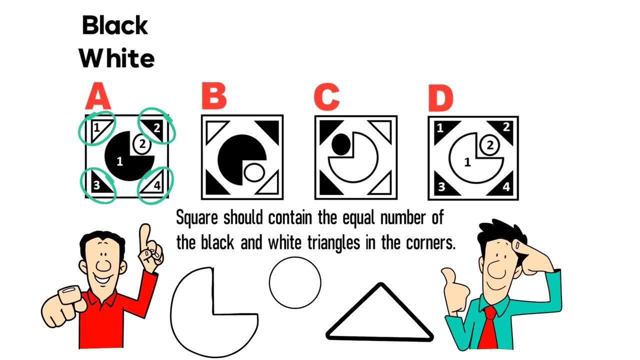 you see that there are four black triangles in the corners. Circles in this picture do not have a pattern and their primary goal is to confuse you. If you look at the circles closely, you see that the large, small circle pattern doesn't exist. We have black white. shape B: black white. 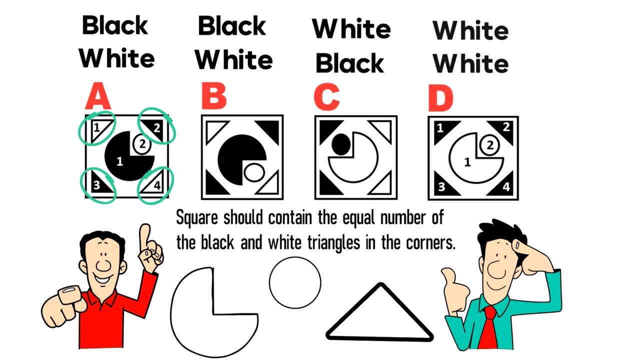 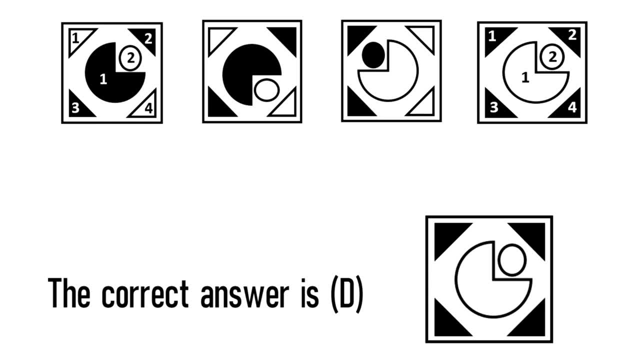 shape C- white- black and then shape D- white- white. Based on this information about the circles, we should ignore them and focus on the triangles inside the squares. This is why the odd shape, the shape that doesn't belong to the group, is the one that does not have equal distributions of all colors in the corners. So the correct 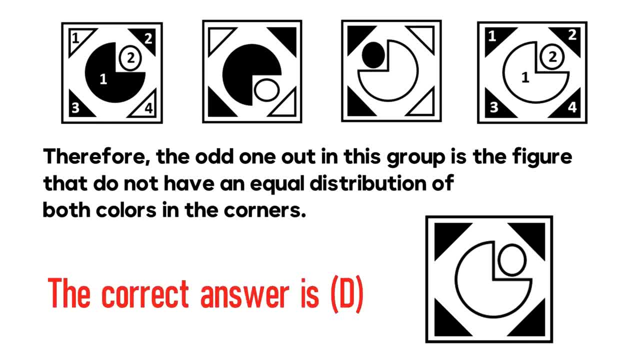 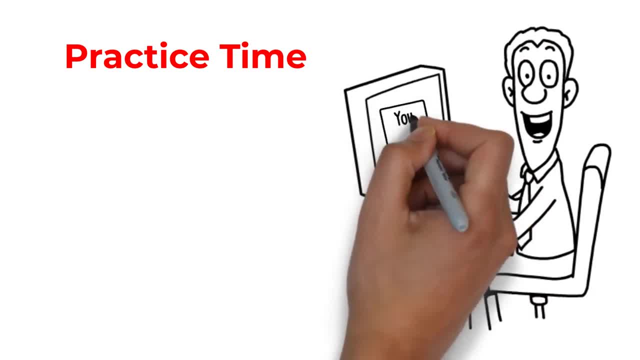 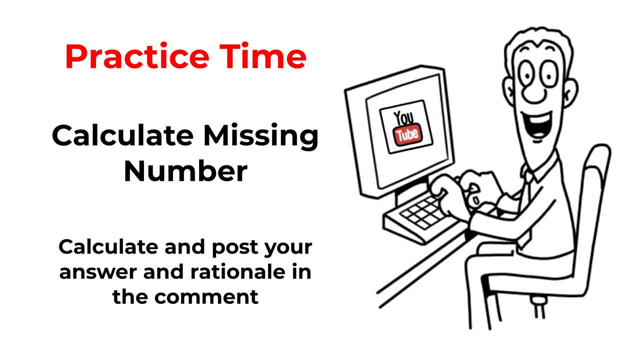 answer here is choice D. Hopefully, you've nailed this question and now know how to answer similar problems on the test, And now it's your turn. I would like you to practice and try to answer this question on your own. Please analyze the question and post your answer as well as your. 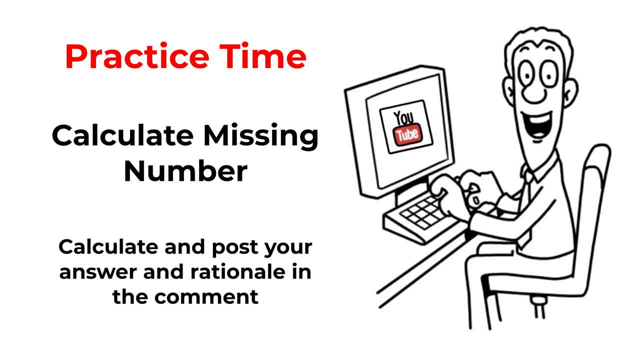 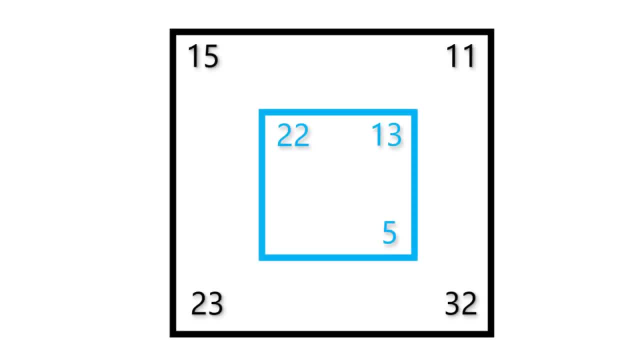 rational answer. If you have any questions, please write them in the comments. And if you have any questions, please write them down in the comments. You are presented with two squares. Smaller square is inside the larger square. Both squares have numbers in the corners. 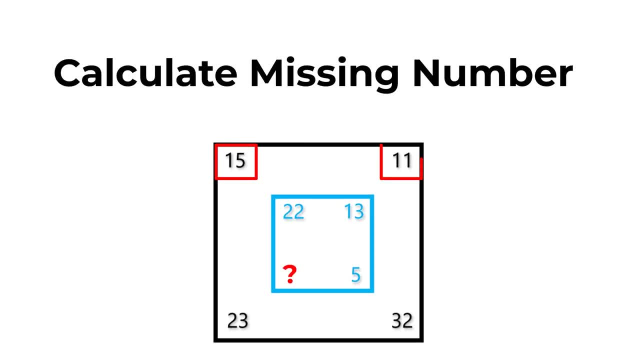 The larger square has numbers 15,, 11,, 32 and 23.. The smaller square has numbers 22,, 13,, 5 and 1 number is missing And this is the number you need to calculate. You have four different choices. 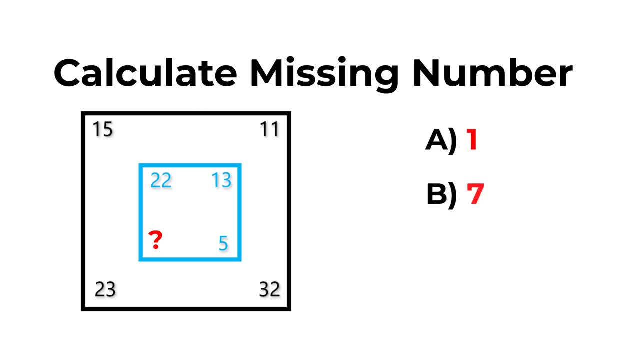 choices: Choice A – 1,, choice B – 7,, choice C – 12, and choice D – 17.. Do you see the pattern? Can you calculate the correct number? Please post your answer in the comment section of this video. 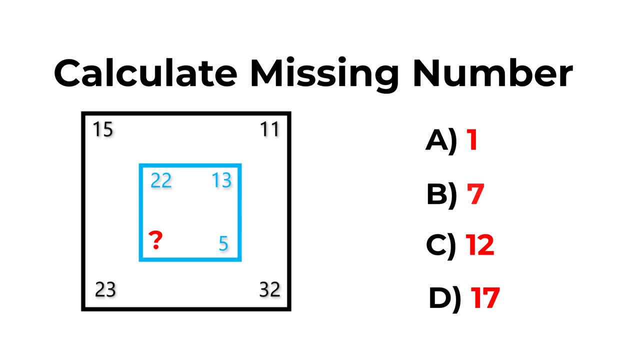 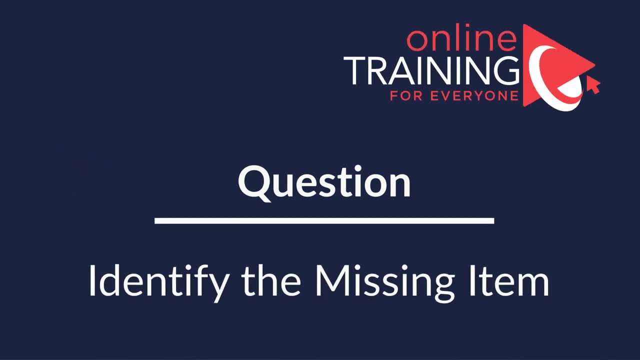 so I can give you my feedback. Thank you for participating and good luck. I'm excited to share with you a cool question which is easy to understand but which doesn't have an obvious answer. You are presented with the 2x3 matrix. 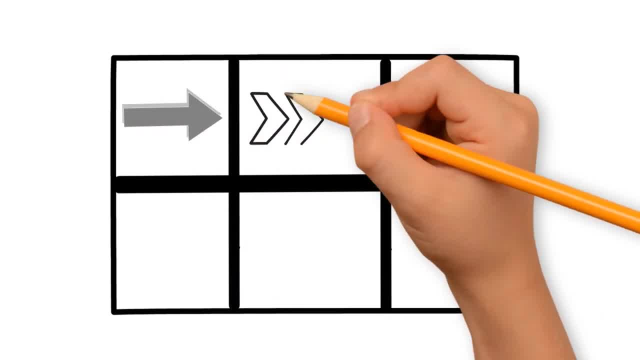 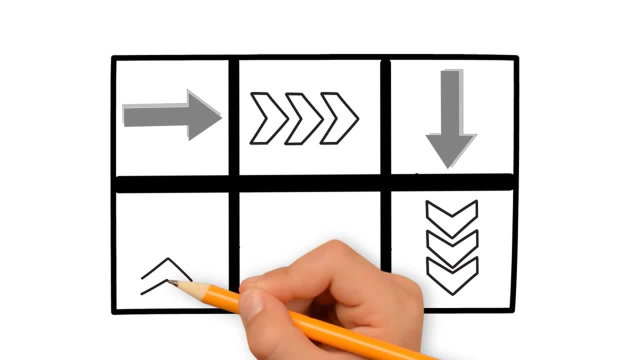 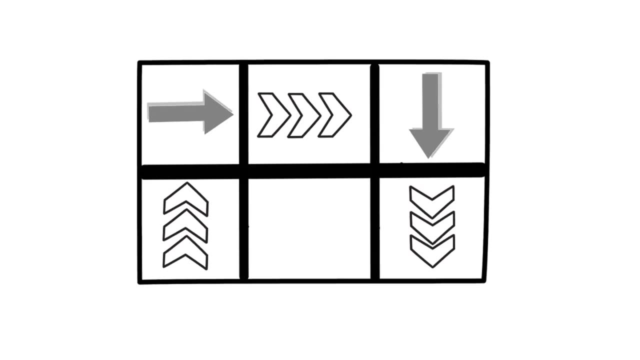 This matrix has arrows inside. There are two types of arrows – solid arrows, and then there are arrows that consist of three different shapes. There are six possible spaces in the 2x3 matrix. Five shapes are present and one shape is missing. You are presented with four different choices. 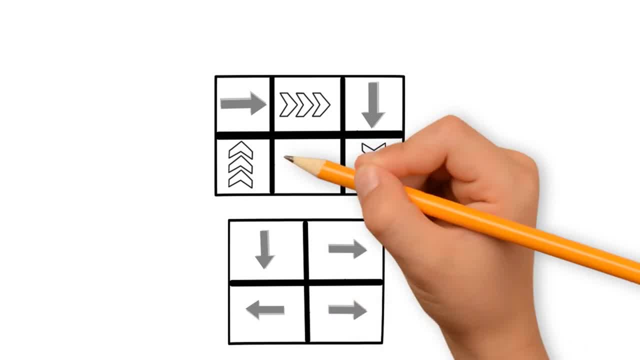 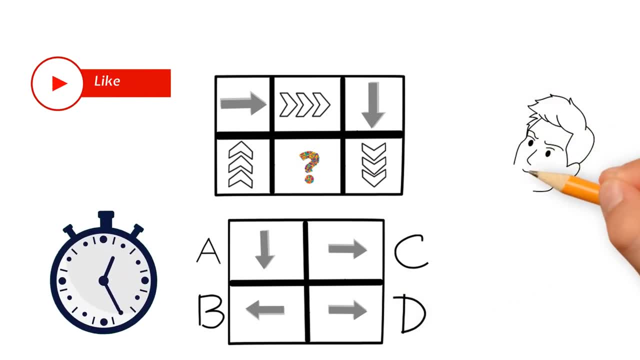 to identify the missing shape which is highlighted by the question mark. You have chosen the 2x3 matrix. You have chosen the 2x3 matrix. You have chosen the 2x3 matrix A, B, C and D. Give yourself 10-15 seconds to see if you can identify the right answer. 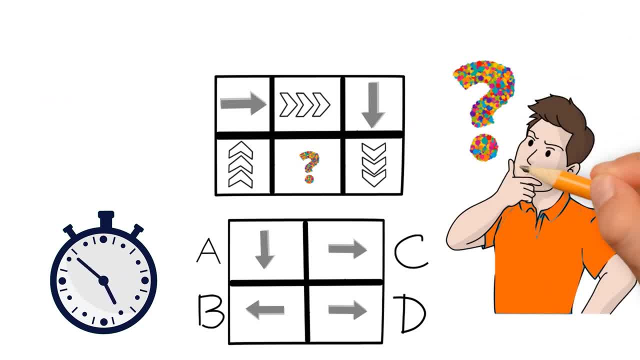 Did you figure out the correct answer? Let's continue to see if we can get to the correct solution together. To solve these types of challenges, you always need to look for patterns, And there are three different patterns present in this sequence. Let's look at the pattern 1.. 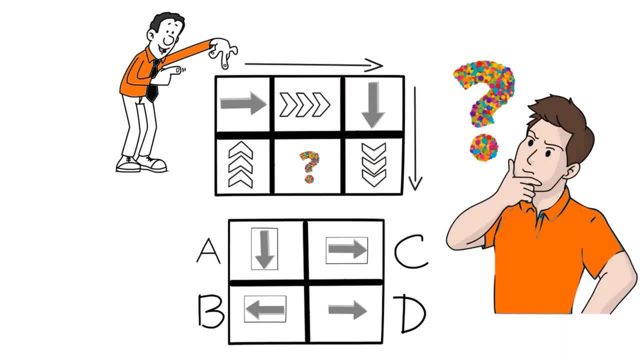 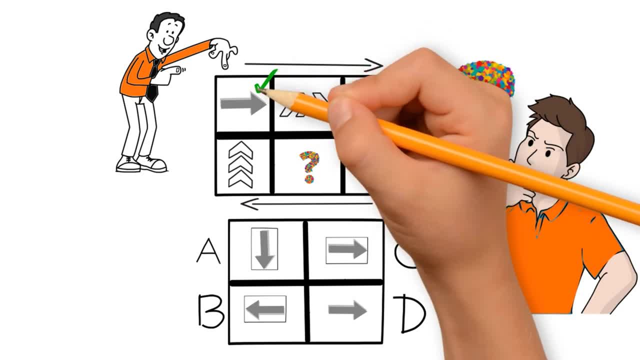 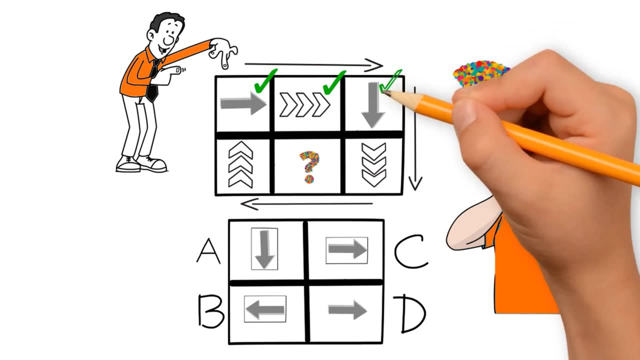 If we start from the upper left corner and go clockwise, you see that the arrows change alternatively in each subsequent box. Second pattern is that inside the box, solid arrows rotate clockwise. And then the third pattern, which is a little harder to identify, is that the previous arrow 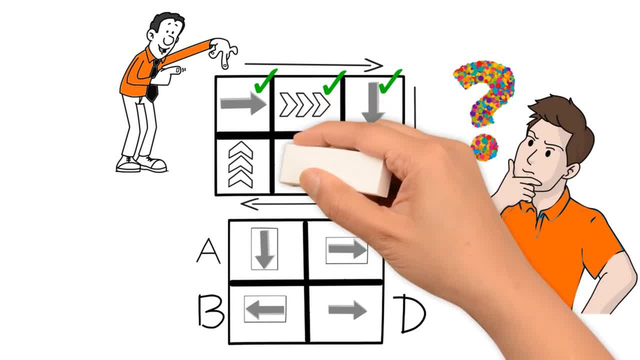 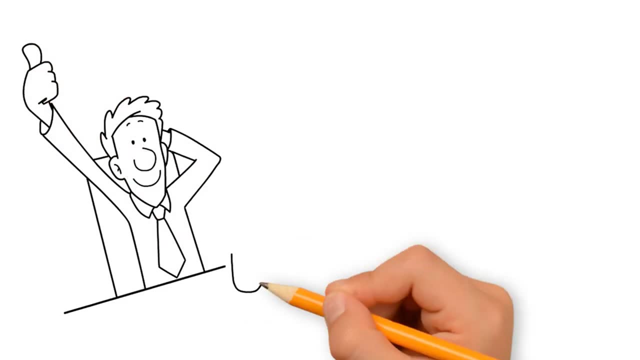 points to the next arrow's start. This is why the missing part- the part that you would need to identify- contains an arrow placed in the right corner pointing to the left. So the correct answer is choice B. Hopefully you've nailed this question and now know how to answer similar problems in the test. 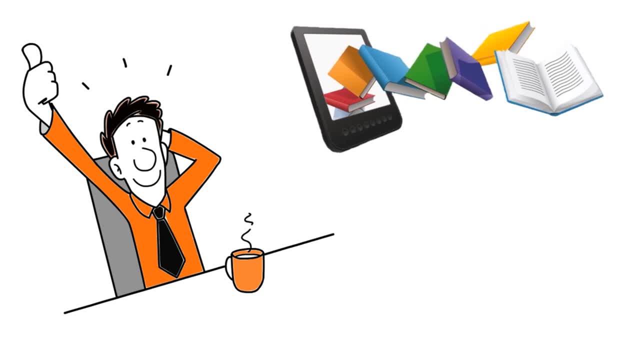 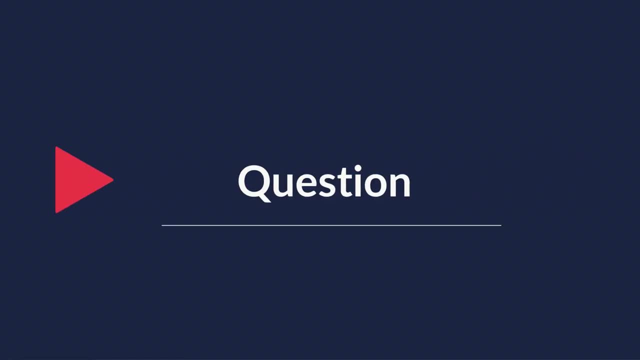 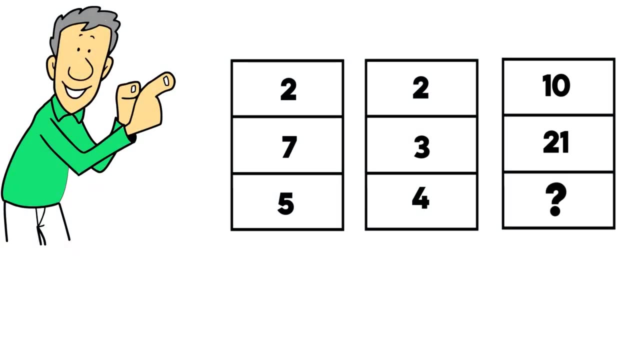 But in case you need more problems and solutions, please make sure to check out my ebook in the description section of this video. I'm extremely excited to share with you the question that tests your pattern recognition skills. You're presented with three columns. Each column has three numbers. In the first column, 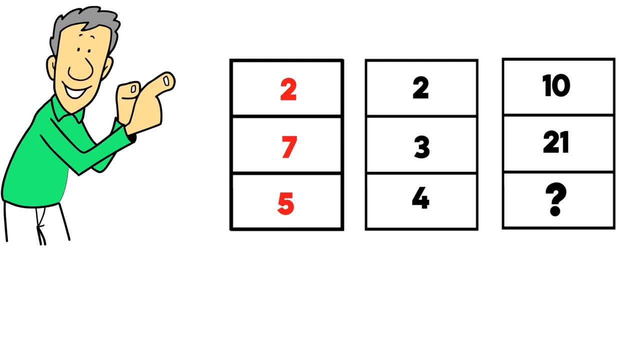 we see numbers 2,, 7, 5.. In the second middle column we see numbers 2,, 3 and 4.. And in the last rightmost column- column number 3, we see numbers 10,, 21 and then one number missing. 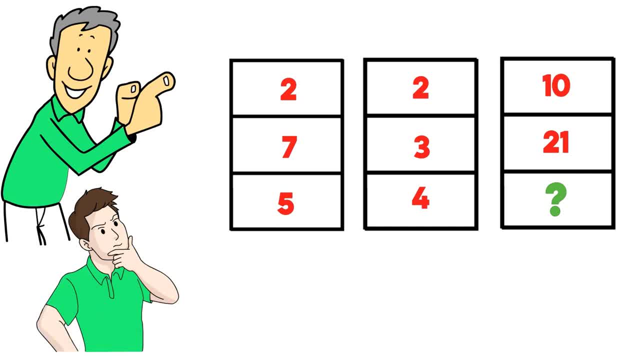 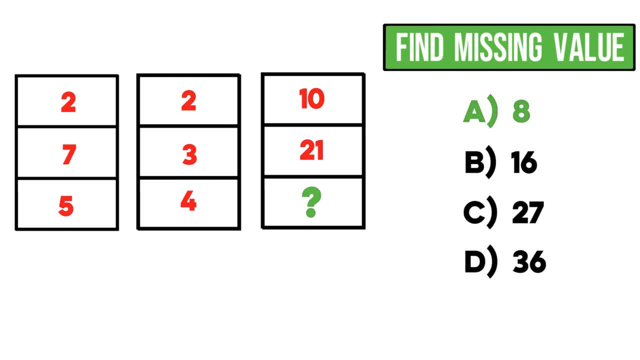 You need to find the missing value, which is highlighted by question mark. You need to find the missing value and you have four choices to choose from: Choice A: 8.. Choice B: 16.. Choice C: 27. And Choice D: 38.. 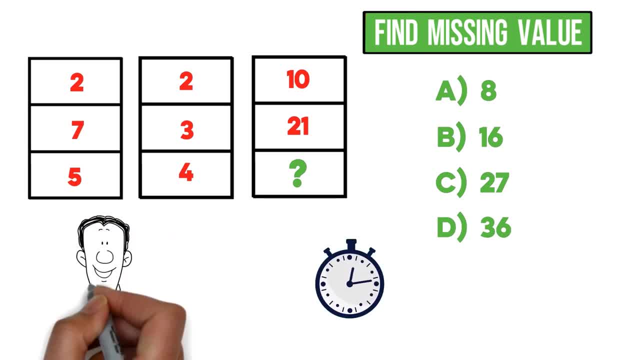 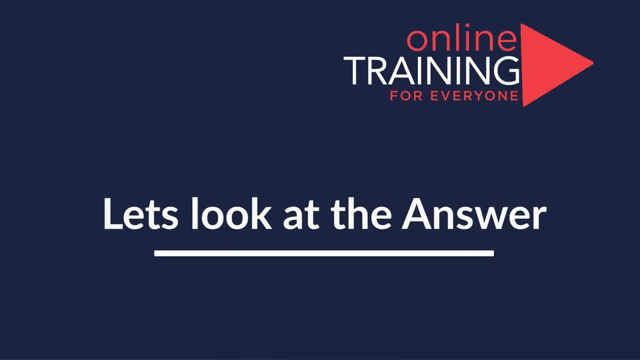 36.. Do you think you can recognize missing value? Give yourself 5 to 10 seconds to see if you can come up with the answer. Did you figure out the solution? Let's continue to see how we can get to the correct solution together. 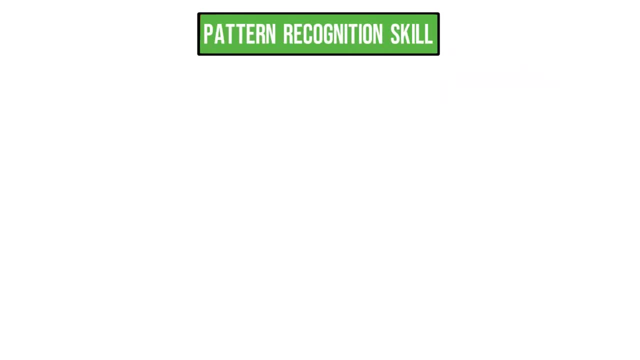 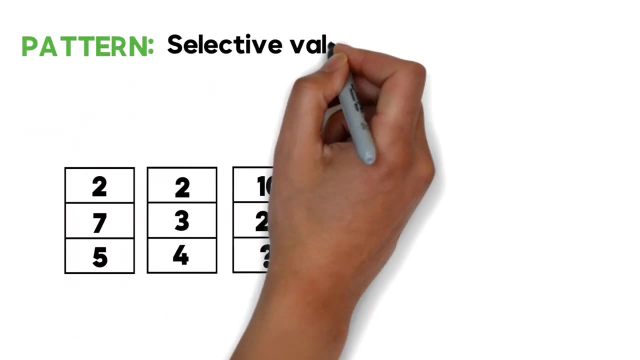 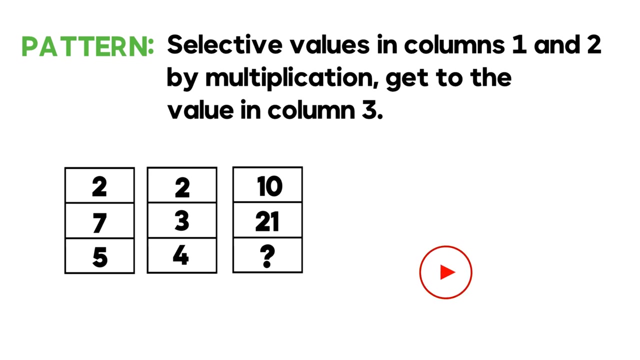 The most important skill to solve these types of problems is pattern recognition skill. To recognize the pattern you need to look closely into each column. Selective values in columns 1 and 2 by multiplication get to the value in column 3.. And this is our pattern. 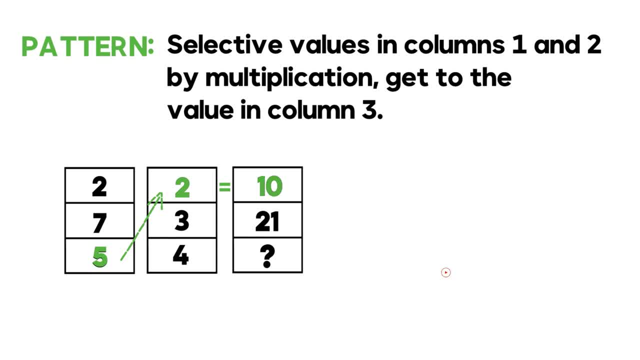 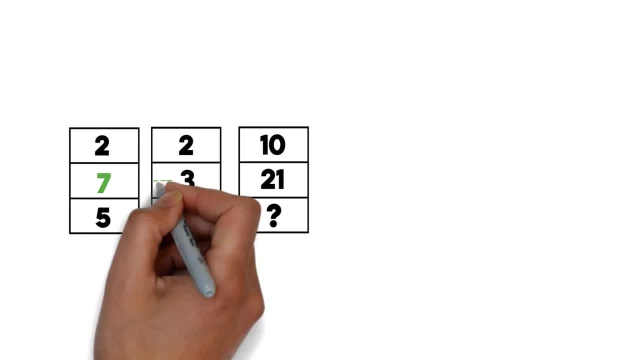 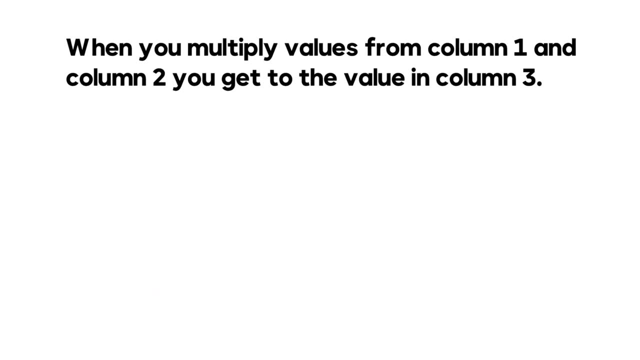 Let's take a closer look for the values that are already present. If we multiply 5 by 2,, we get to the value of 10.. Second set of values, represented by the middle row: 7, multiplied by 3 equals 21.. So the missing values here can be calculated by multiplying 2 by 4, and. 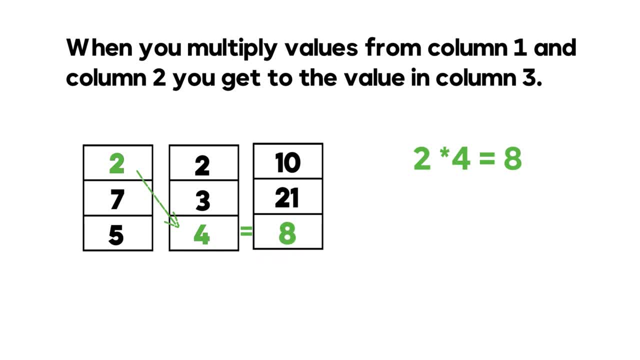 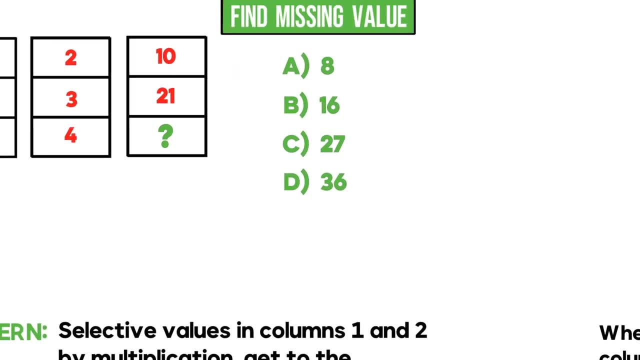 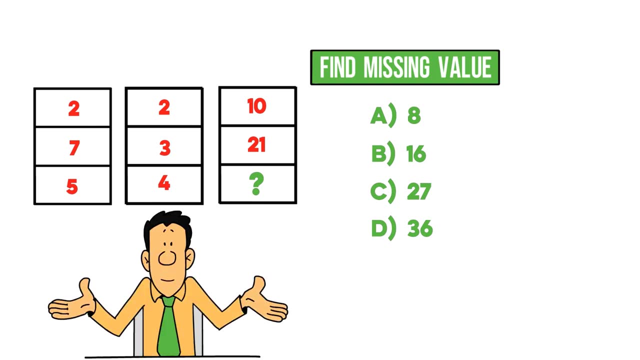 the end result is 10.. So the correct answer to this problem is choice A 8.. I also wanted to share with you one of the typical mistakes people make as part of answering these types of questions. People start looking at the columns themselves, But unfortunately, 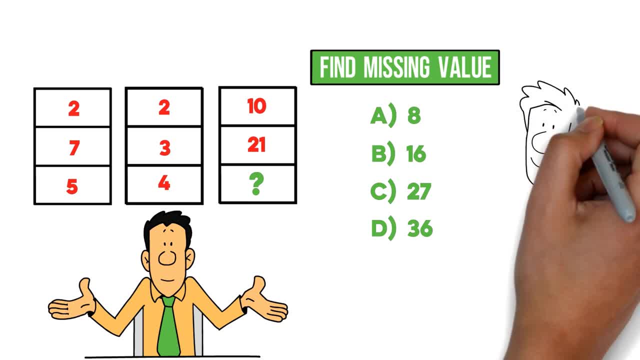 there is no pattern just by looking in the values in column 1,, since pattern just doesn't exist. If you look only at the values in column 1, or only at the values in column 2, or only at the values in column 3,, you will not be able to come up with the answer You have. 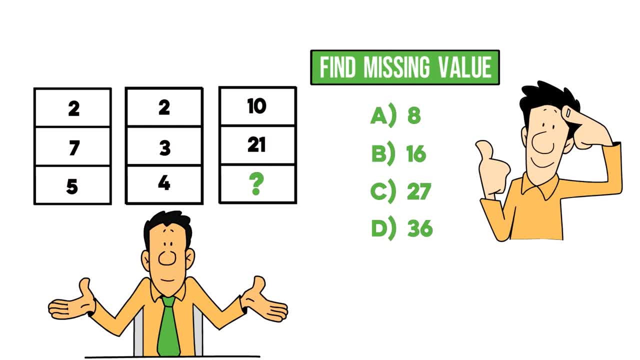 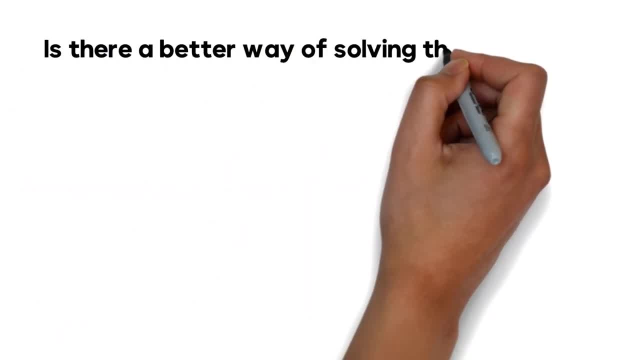 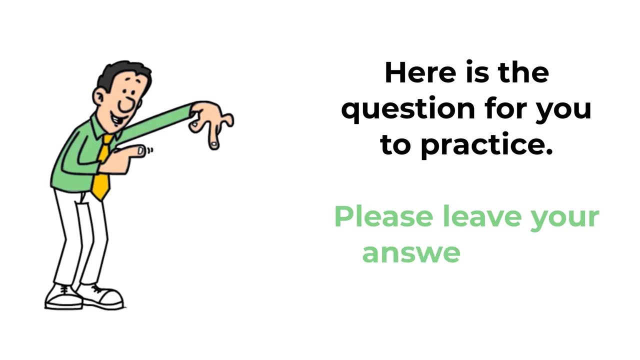 to look across and take a global view across multiple columns to get to the correct solution. Can you do me a favor? If you have a better way of solving this challenge, please share your thought process in the comment section of this video. And now here is the question for you to try. If you can calculate the answer, please leave. 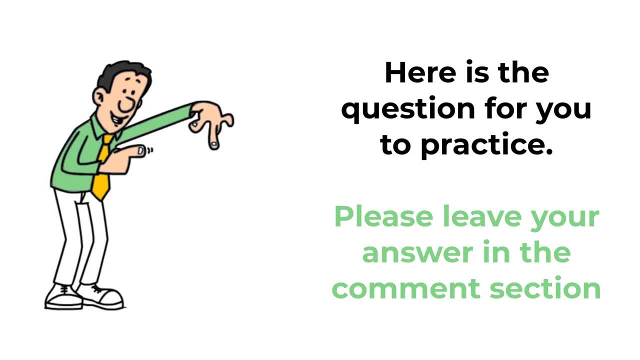 it in the comment section of this video so I can validate it and give you my feedback. Now here is the question: How can we get rid of difference between values of 2 and 3?? Here is the question: How can we get rid of difference between values of 2 and 3?? Can we get rid of the difference between values of the values of 2 and 3?? 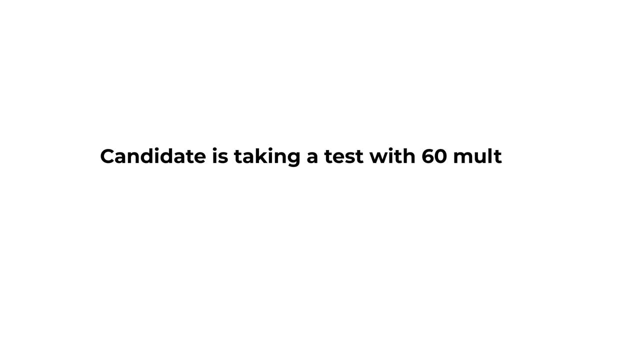 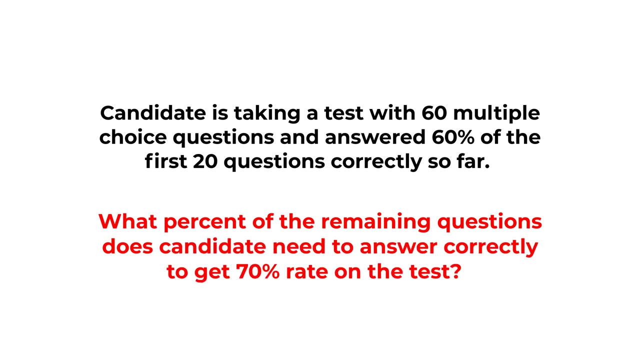 candidate- imagine yourself- is taking a test with 60 multiple choice questions and so far answered 60% of the first 20 questions correctly. What percent of the remaining questions does candidate need to answer correctly to get 70% rate on the test? You're presented with four. 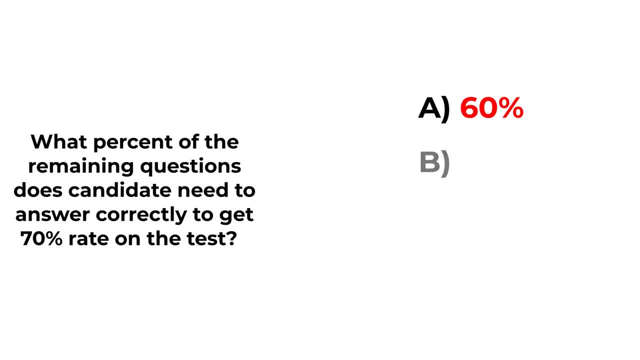 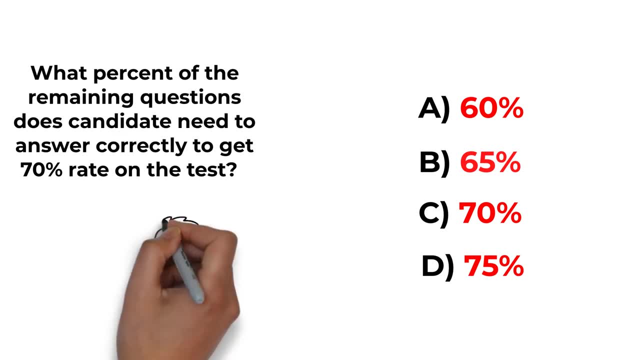 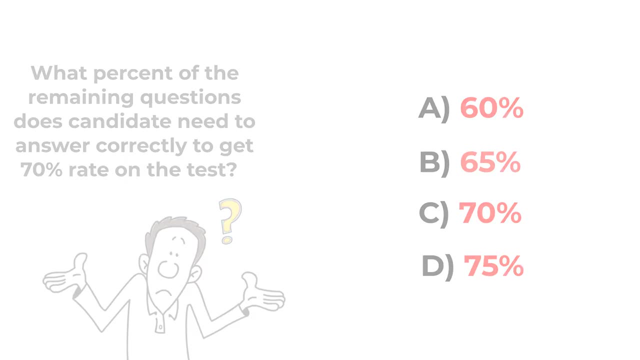 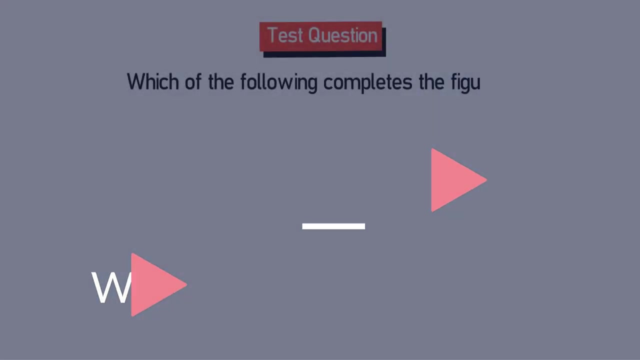 different choices: Choice A- 60%, Choice B- 65%, Choice C- 70% And choice D- 75%. Can you calculate the answer? Please make sure to leave the calculated answer in the comment section of this video. Thanks for participating and good luck. I wanted to share with you a cool question. 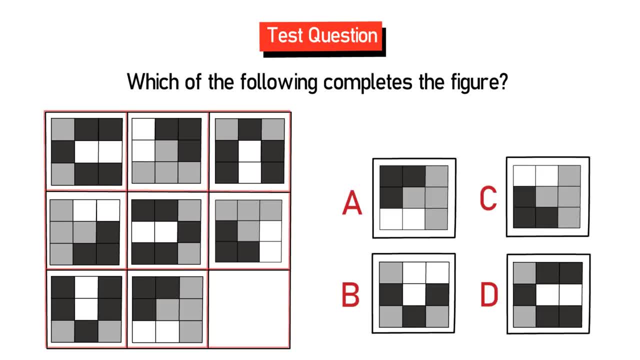 which started showing up on the tests very recently. You're presented with the 3x3 matrix. Each square of the matrix contains another matrix inside. with the 3x3 small squares, There are different colors inside 3x3 small squares. 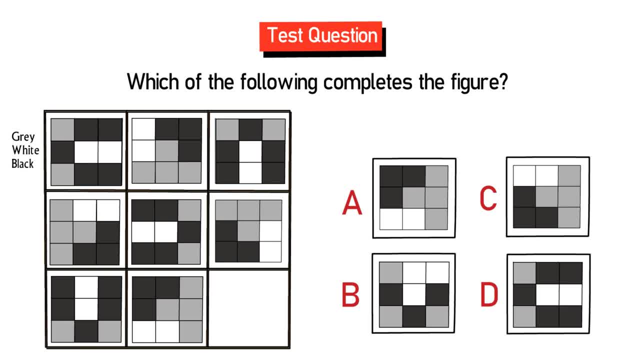 In this case, we see gray, white and black. One 3x3 square is missing and you need to select out of the four possible choices- Choices A, B, C and D- And your goal is to determine which of 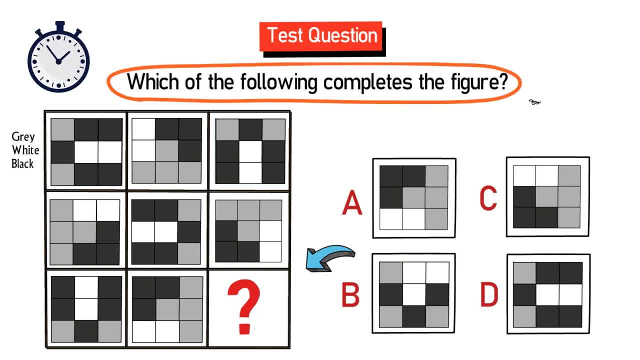 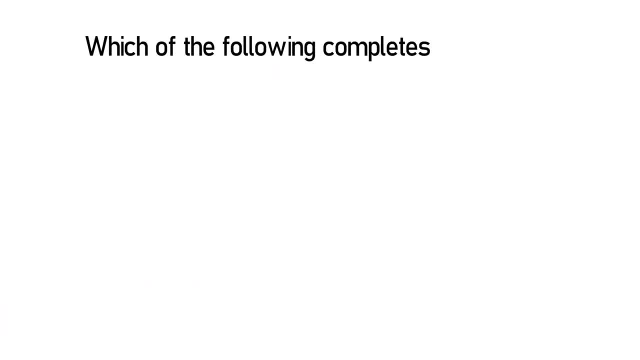 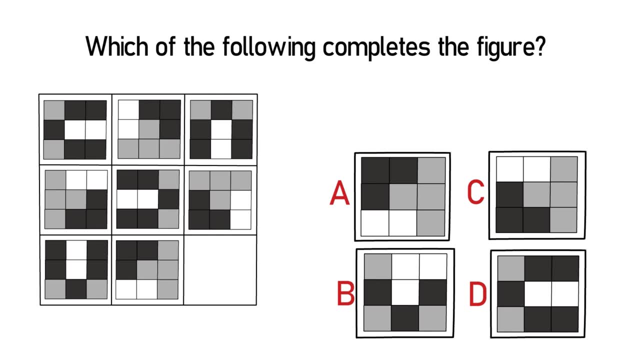 the following shapes completes the figure. Take a close look and see if you can identify the missing item. Do you think you know the answer? Let's continue to see how we can get to the correct solution together. First time you might be intimidated by this matrix, But the answer actually is very simple. 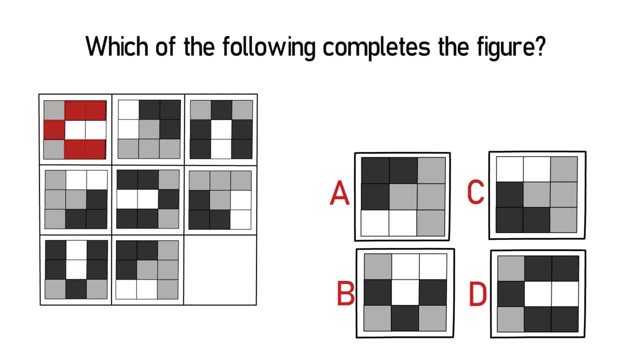 If we look closely at the smaller matrices, you see that the letters are being formed. You see that in the upper left corner black boxes form a letter V. And if we look at the upper right corner, you see that the letter V also shows up. but now it's turned clockwise. 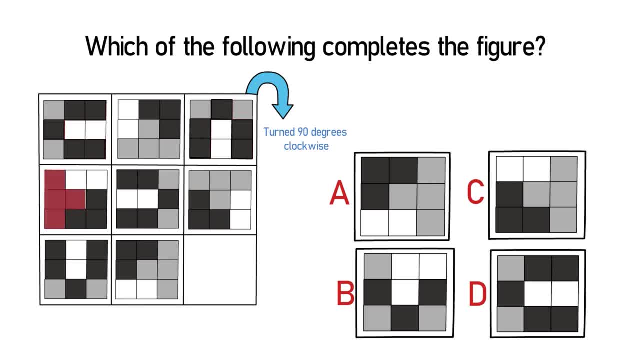 from the previous position. Let's go to the second row. In the second row you can recognize letter T. This letter shows up in the left column, But if we look in the middle row, in the right column, you see that the same letter T now is turned 90 degrees from the previous position. 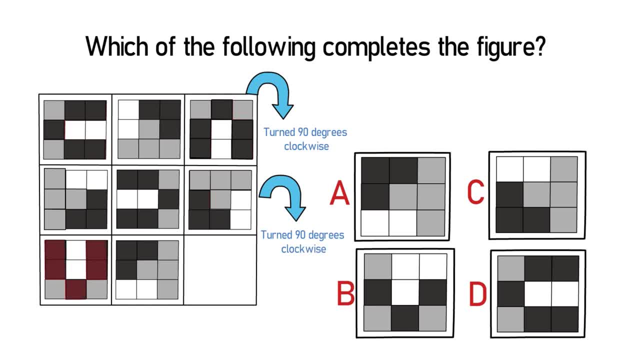 So now, if we follow the same logic, you can recognize letter V in the bottom left corner. According to the pattern that we've identified, this letter should be turned 90 degrees in the bottom right corner. So the correct answer here is choice D, Hopefully. 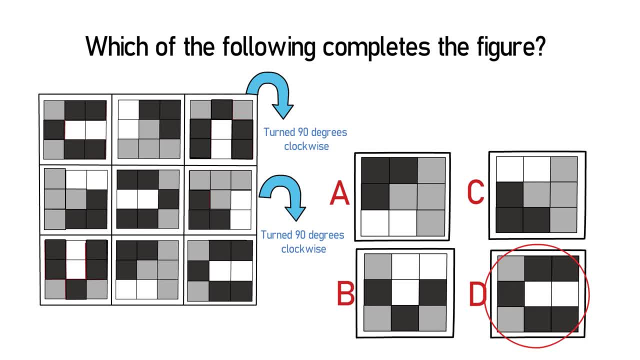 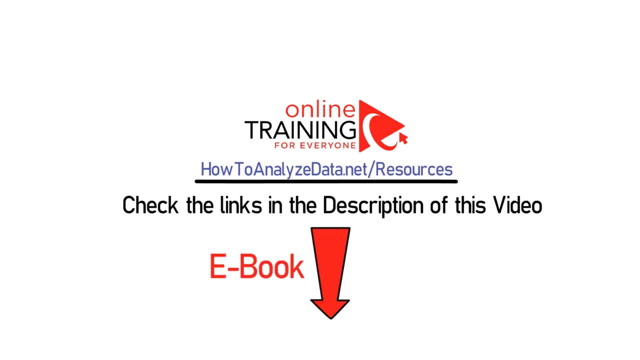 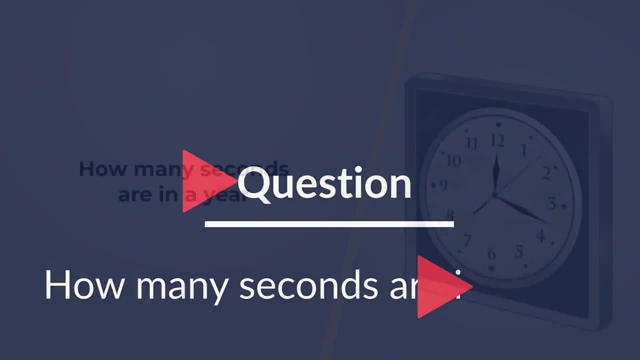 you've nailed this question and now know how to answer similar problems on the test. If you need to practice with more questions, please make sure to check out my e-book. in the description section of this video, I had this question being asked as part of a consulting job interview. 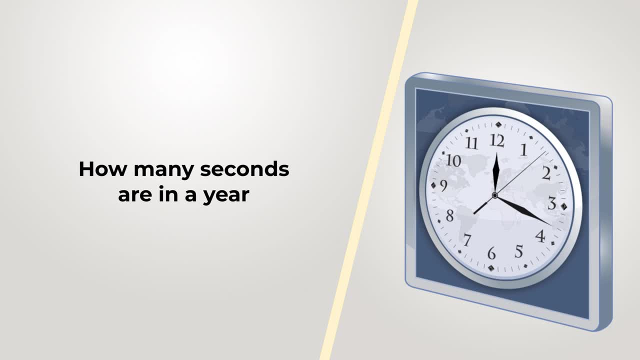 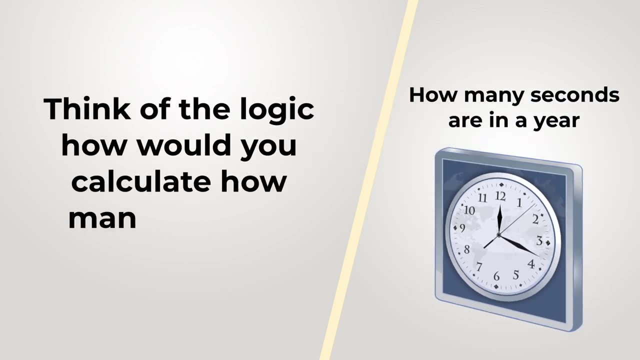 How many seconds are there in a year? Take a look at the picture. it might give you a hint. Do you think you know the answer? Think of the logic. how would you calculate how many seconds are there in a year? Or maybe there is an alternative. 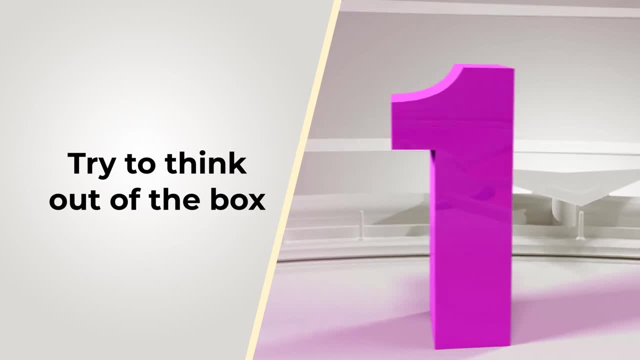 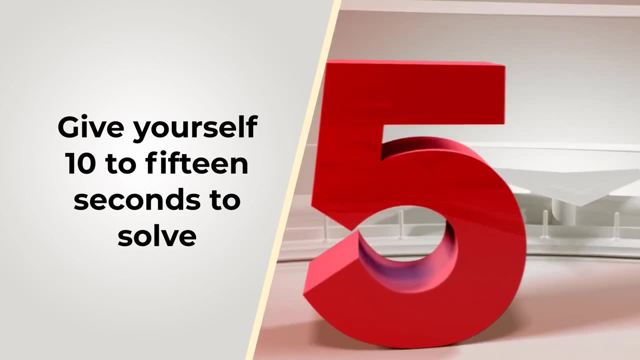 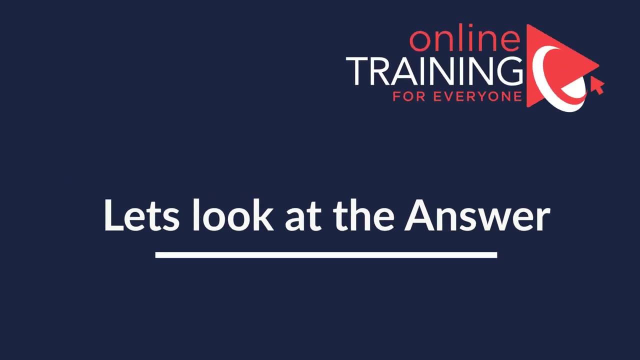 always try to think out of the box- this would be my hint to you- and give yourself 10 to 15 seconds. this is as much time as you might get answering these types of questions in the test. now let's continue and get to the correct solution together. obviously, this is a tricky question and 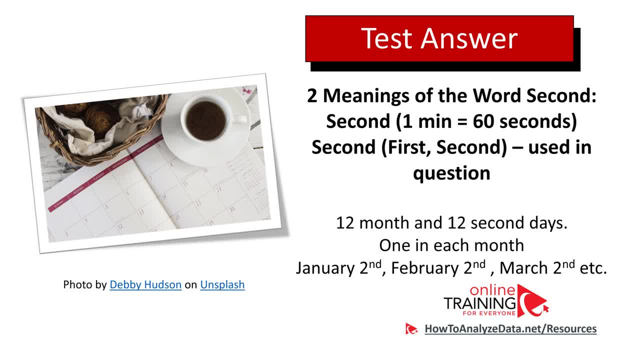 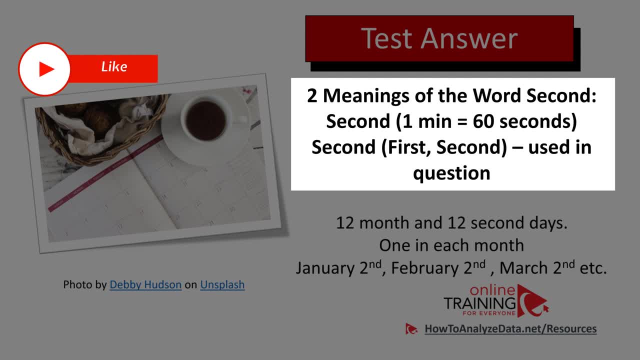 it challenges you in understanding of the word second. there are two meanings in the word second. one is second- for example, one minute has 60 seconds- but second one is second, where you have sequence of first and second and the second meaning of the second is used in this particular question. 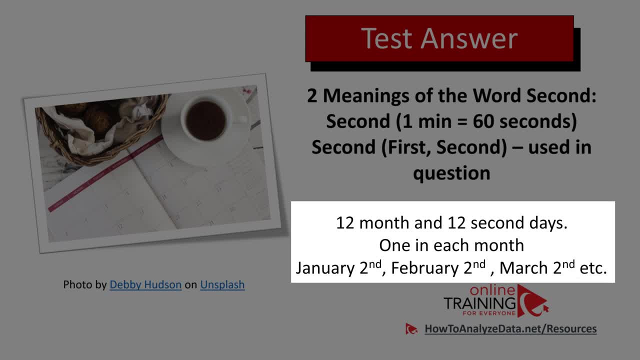 so, if we go back to the question, in the year there are 12 months and there are 12 second days, one second day in each month's: January 2nd, February 2nd, March 2nd and etc. hopefully you've nailed this question. it gives you some laughs and you know that you have a lot of questions. 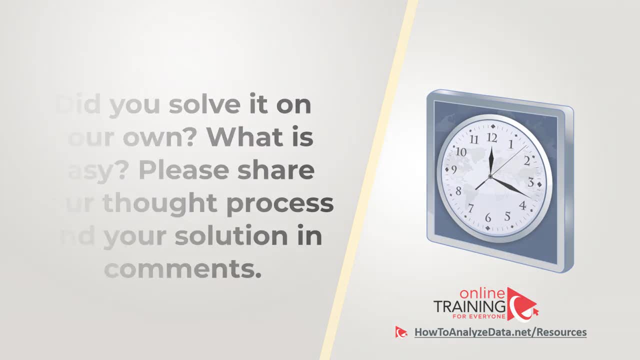 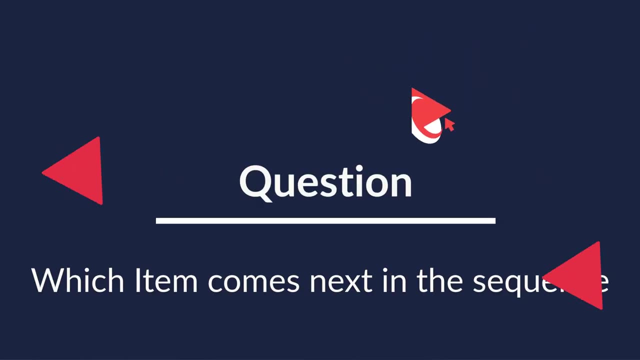 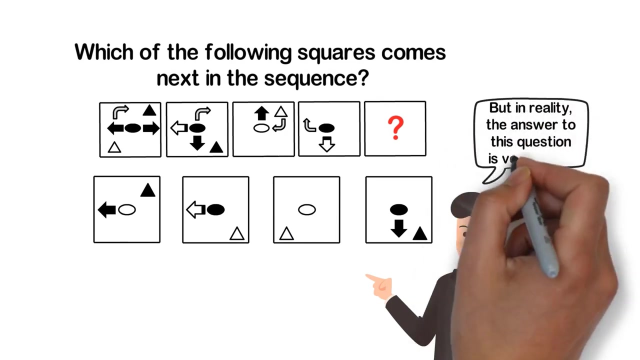 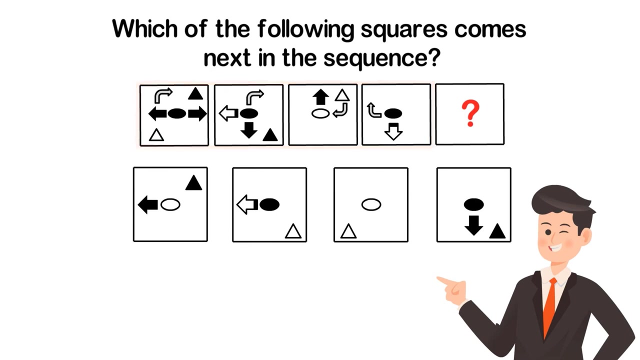 you now know how to answer similar problems in the test. here's the question that on the surface seems very, very hard to solve, but in reality the answer to this question is very simple. you're presented with five different squares. squares one through four have shapes inside and you need to determine the missing square five. you're presented with four. 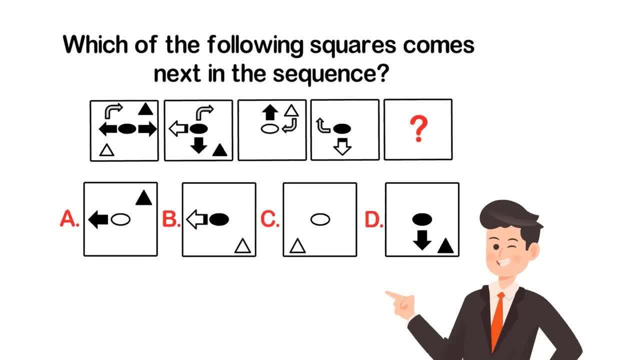 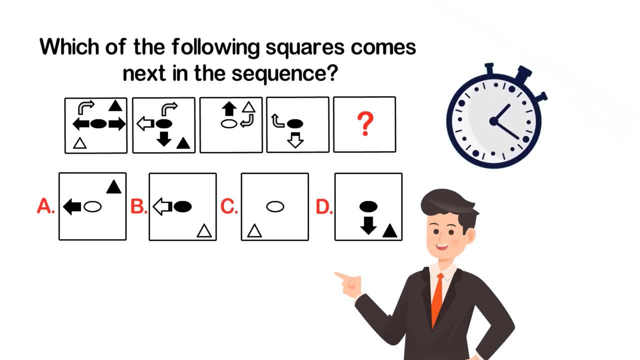 different choices: A, B, C and D. take a close look to see if you can come up with the correct answer. maybe give yourself five to ten seconds, or maybe longer- 10 to 20 seconds. this is about as much time as you'll get on the real test. did you figure out the answer? let's continue to see how we can solve. 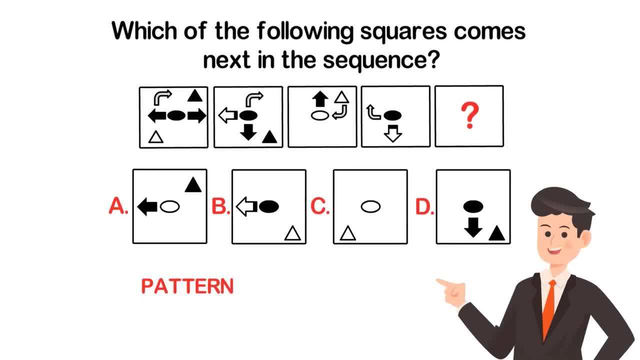 this challenge and get to the correct solution together. as I mentioned, test writers are trying to trick you and in this particular case, there is no pattern within the shape. it's all random. no matter how hard you try, you will not be able to determine any patterns among those small shapes. 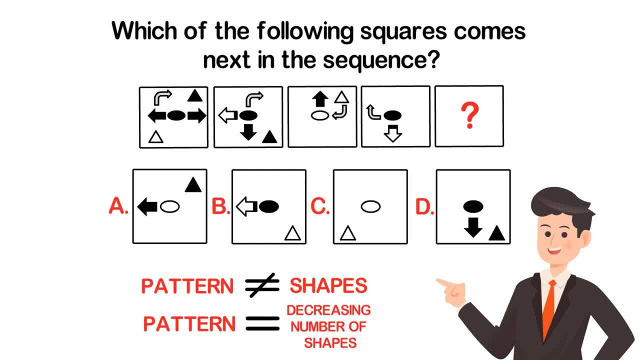 the pattern here is the decreasing number of shapes. if you look at the figure one, it has six shapes. if you look at the figure two, it has five, four, three. so the answer for the figure five, the number of inside shapes, should be two. so the correct answer here is choice C. hopefully you 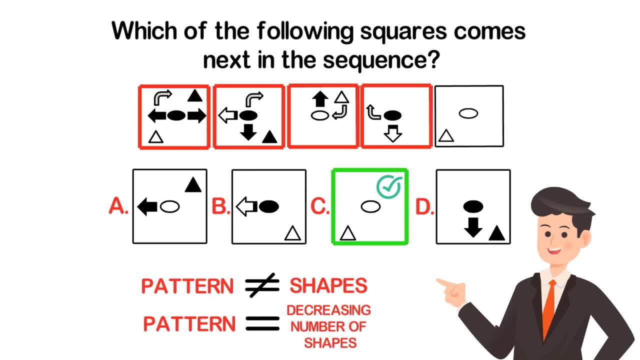 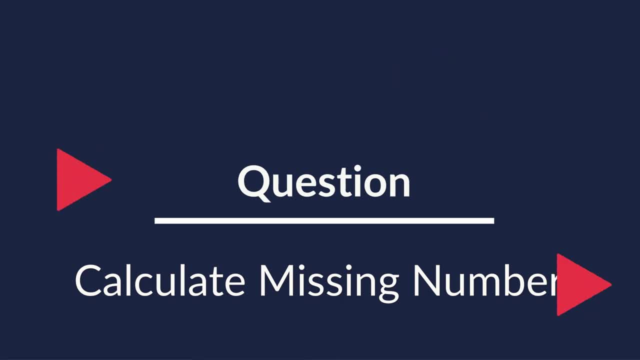 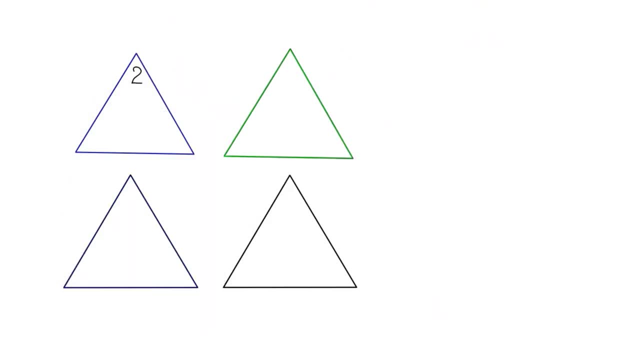 nailed this question and now know how to answer similar problems on the test. here's another puzzling question you might find difficult to solve. you are presented with four triangles. each triangle has a number in the corner and you need to calculate one of the missing numbers in the upper corner of the black triangle. 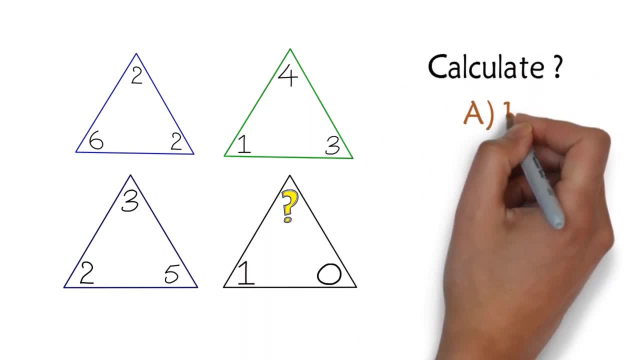 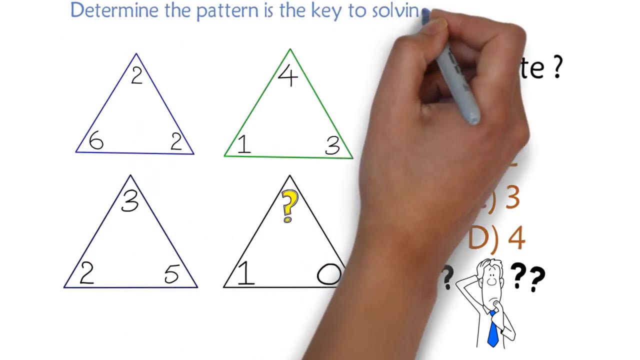 you have four different choices. you have choice A one, you have choice B two, you have choice C3 and you have choice D4. can you determine the answer? let's continue to see how we can solve this challenge together. determining the pattern is the key to solving. 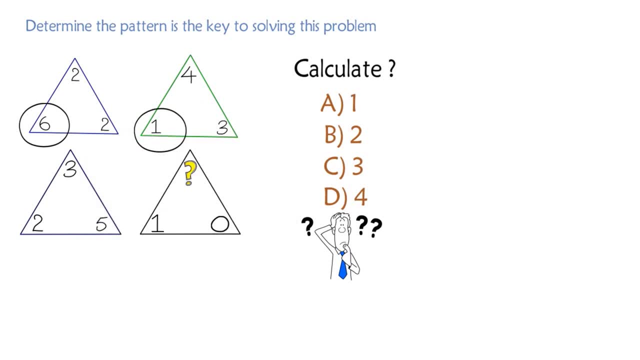 this challenge. for example, if you add up the numbers in the lower left corners, six plus one plus one plus two, in all triangles, you will get to the sum of ten. same thing happens when you add up the numbers in the bottom right corners of the same triangles: two plus three plus zero plus five. 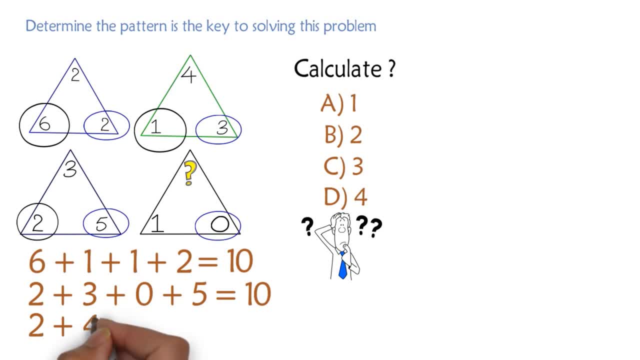 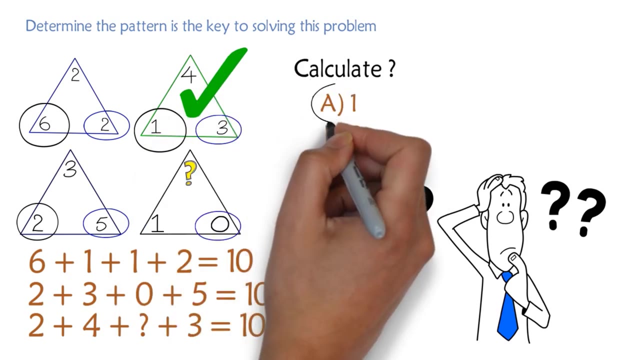 also equals ten, so same logic can be applied to the upper right corners of the triangles. as you can see, triangles are colored to confuse you, so you're only concentrated on the numbers inside of each triangles, but you're not looking across multiple triangles. the correct answer to this problem is choice A one, because this is the math. 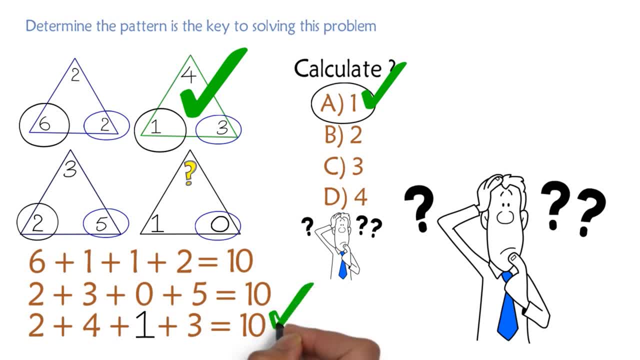 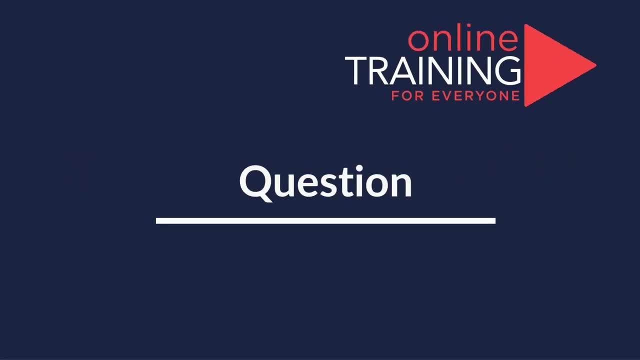 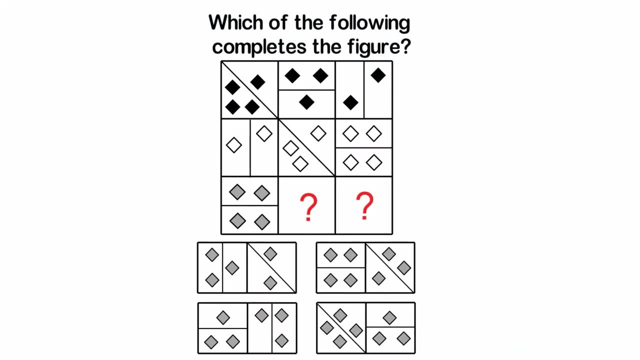 of getting into 10 with the missing number. hopefully, you've nailed this question and now know how to answer similar problems on the test. when you see a question like this, you might ask yourself how can it possibly be even more confusing? but the reality is that the answer to the question I'm about to show you is very simple. let's look. 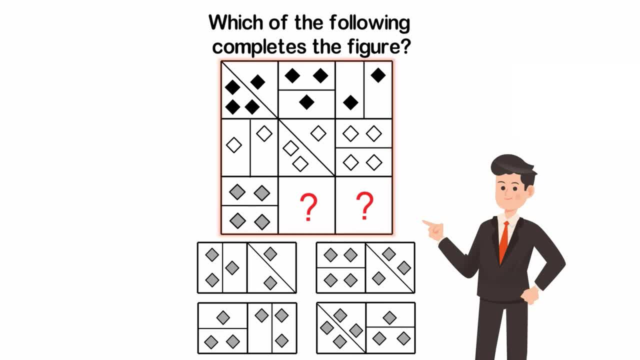 in more details. you're presented with the 3x3 Matrix. two of the shapes in the Matrix are missing. they are located in the bottom row and you have four possible choices for the answers: choices A, B, C and D. take a close look. the solution is. 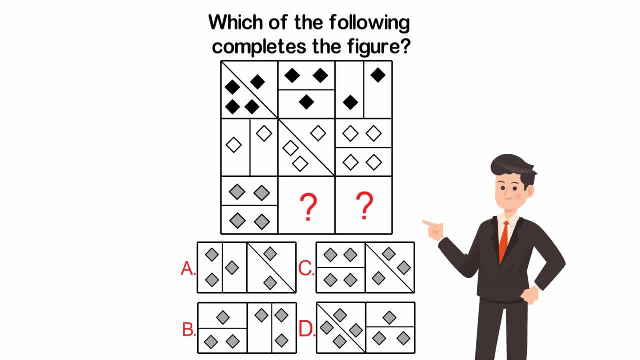 not obvious, but it is very simple. Give yourself 10 to 20 seconds, maybe go to 30 seconds by pausing this video to see if you can come up with the answer on your own. Are you ready? Let's continue. 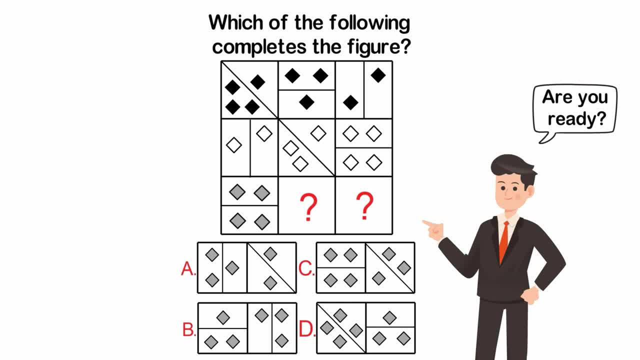 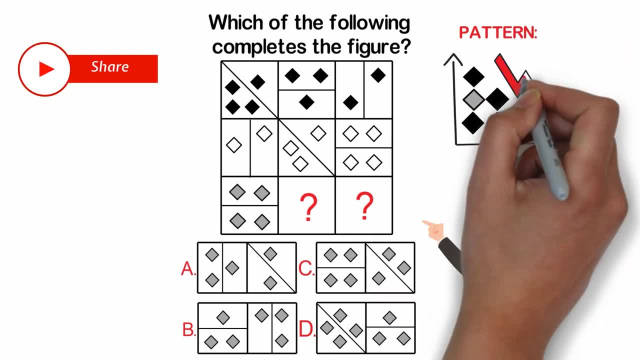 to see how we can get to the correct solution together. As I mentioned, the answer to this question is very simple. The pattern is represented in each row by decreasing number of diamonds. Let's look at the top row. You see that the top left square contains four black diamonds. 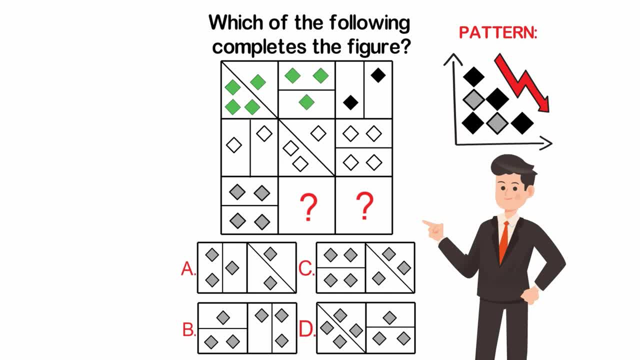 The middle square in the top row contains only three diamonds, And then the right square in the top row contains only two diamonds. In the second row the pattern reverses and it goes from right to left And you see the same pattern of the white diamonds: Four goes down to three and then goes. 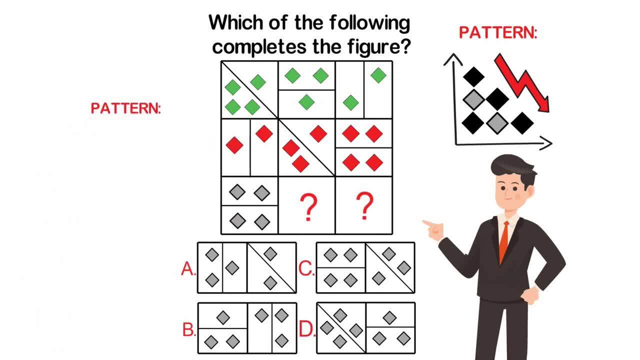 down to two. So in the bottom row we need to follow the same pattern. The pattern will be the number of diamonds decreasing from four to two among the gray diamonds. So the correct answer here is choice A. Hopefully you've nailed this question. 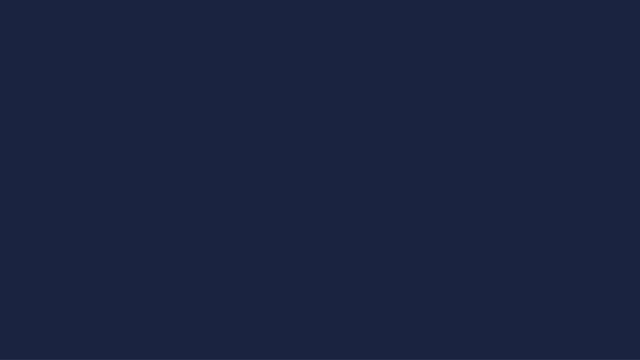 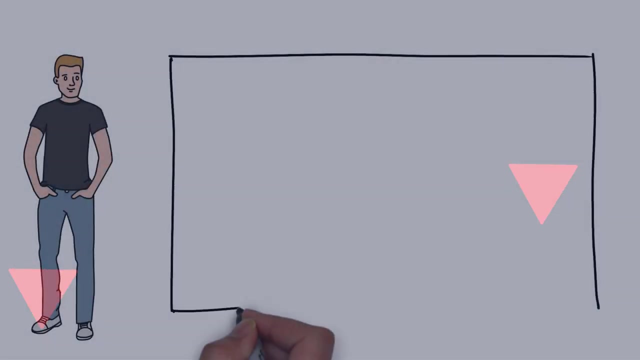 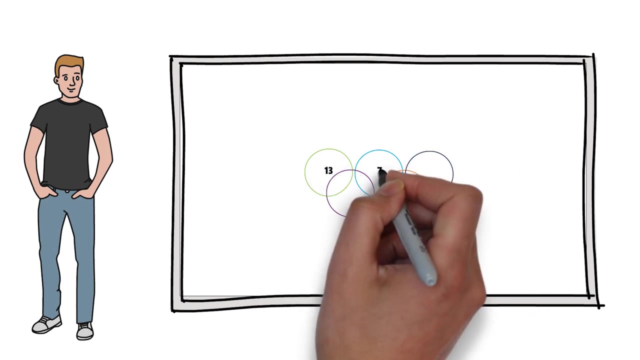 And now know how to answer similar problems in the test. This is one of my favorite questions because it is very frequently used in the test. You're presented with five crossing circles. All circles are of the different colors. There are numbers inside the circles as well as the numbers on the intersections of the circles. 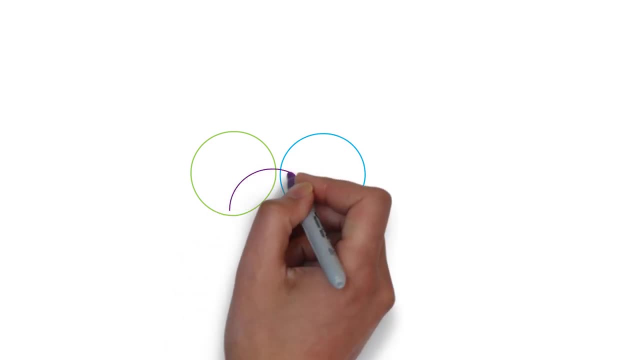 In this particular case, you're presented with five different circles, all of them different colors, And the numbers that you see on the screen are five different colors: 13,, 3, 4, 7, 5, 10,, 1, and 15.. There is also one number missing, which is highlighted with the 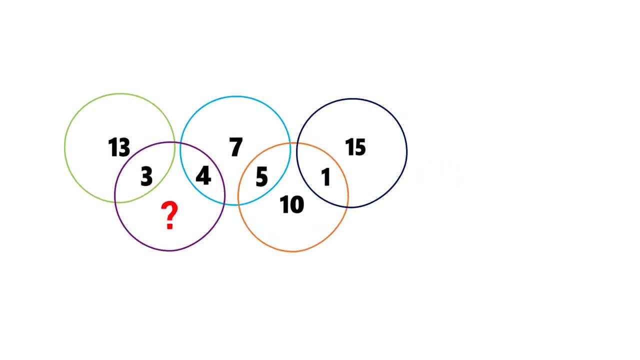 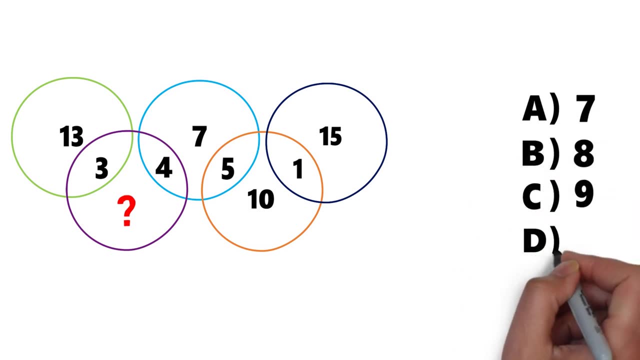 question mark. You need to calculate the missing number And the choices are choice A- 7,, choice B- 8,, choice C- 9, and choice D- 11.. Give yourself a few seconds, maybe 10 to 15 seconds. This is. 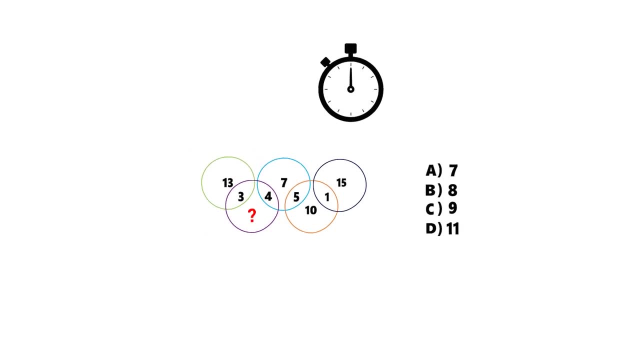 about as much time as you get on the typical test to calculate the answer. Do you see the solution? Let's continue to see how we can get to the correct solution and solve this challenge together. As you might have figured out by now, sum of each numbers in the circle adds up to 16.. For example, 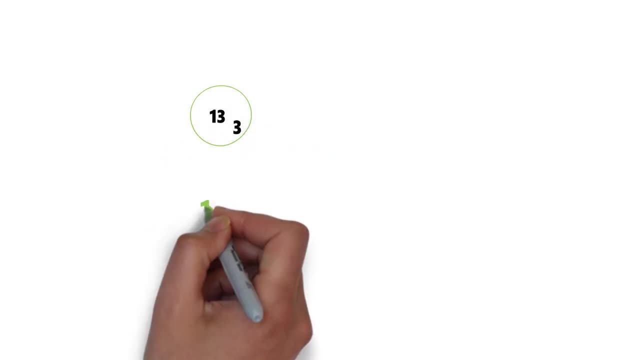 let's look at the green circle. We have numbers 13 and 3,, and 13 plus 3 equals 16.. In the blue circle, we have numbers 4 plus 7 plus 5, and all of them add up to 16.. In the black circle, 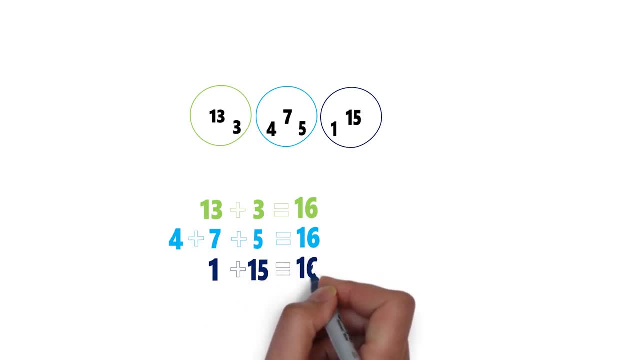 we have 1 and 15, also adds up to 16.. And in the orange circle we have 5 plus 1 plus 10, also equals 16.. So to calculate question mark, which is the missing number, we need to add 3 plus 4 plus question mark and make an equation. 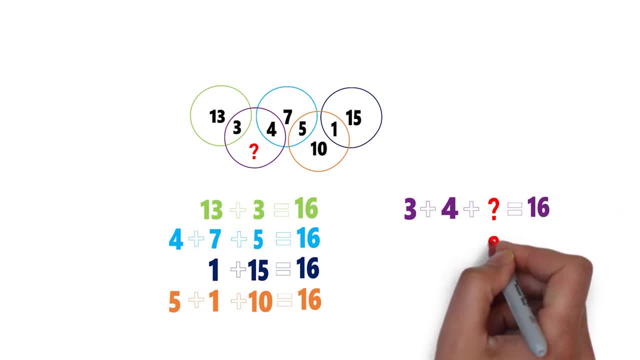 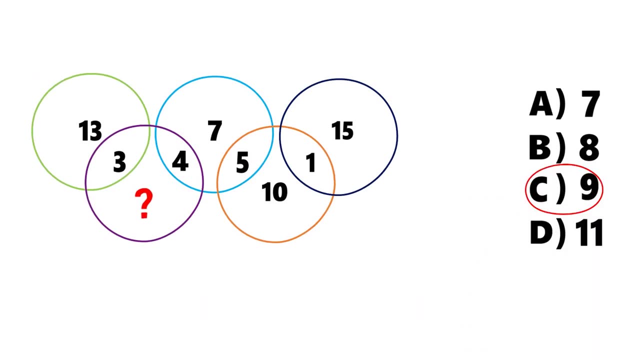 to make it equal 16.. After doing the calculation, you see that the question mark and the missing number equals 9.. So the correct choice here is choice C 9.. Hopefully you've nailed this question and now know how to answer similar problems on the test. 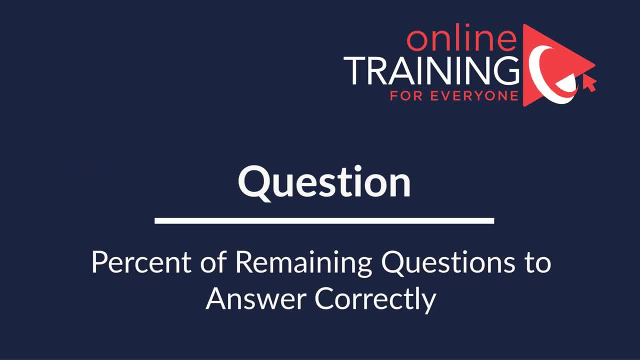 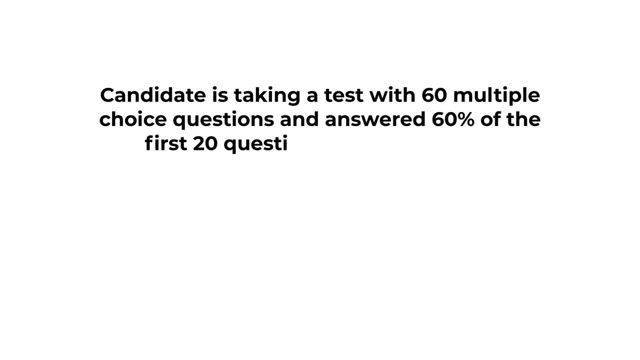 Here is one of the frequently used questions to test your understanding of the percentages Candidate is taking a test. so imagine yourself with 60 multiple choice questions and answered 60% of the first 20 questions correctly so far. So what percent of the remaining questions? 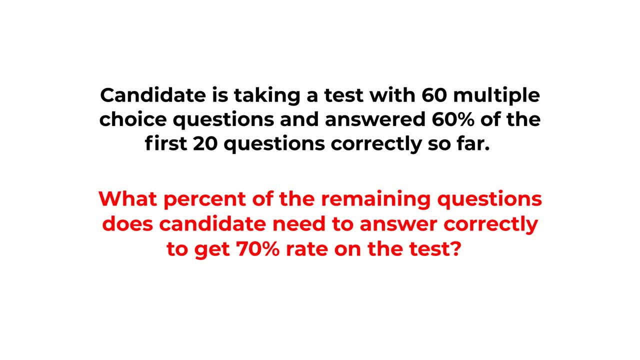 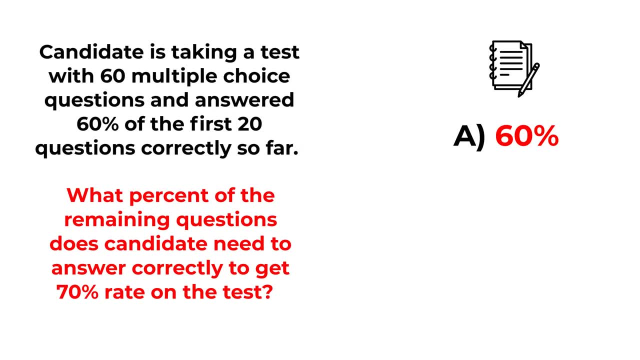 does candidate need to answer correctly to get 70% rate on the test. You're presented with four different choices: Choice A, which is the most common question and which is the most common question. Choice B- 60%. Choice B- 65%. Choice C- 70% And choice D- 75%. Do you see the answer? 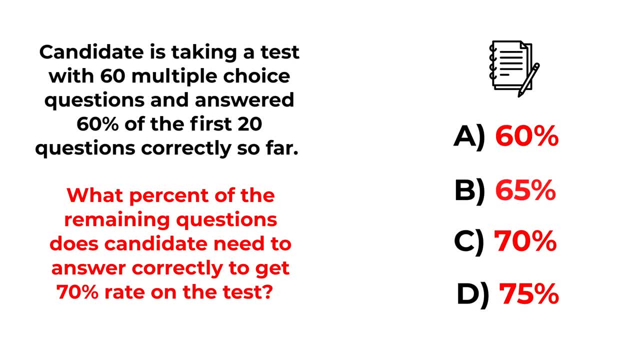 Take a close look and possibly get yourself a piece of paper or use Microsoft Excel to do the calculations. Or maybe you can do all the calculations in your head. That would be amazing. Give yourself 15 to 20 seconds. This particular question might require a lot of steps, So give. 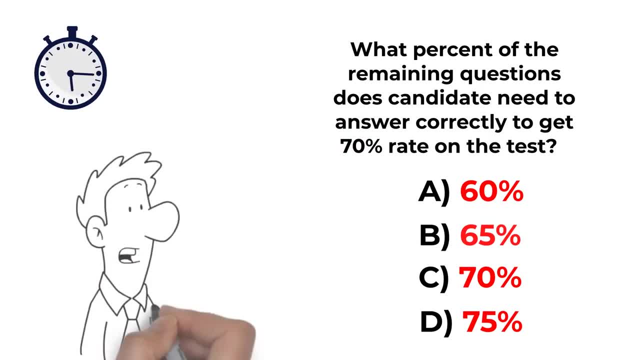 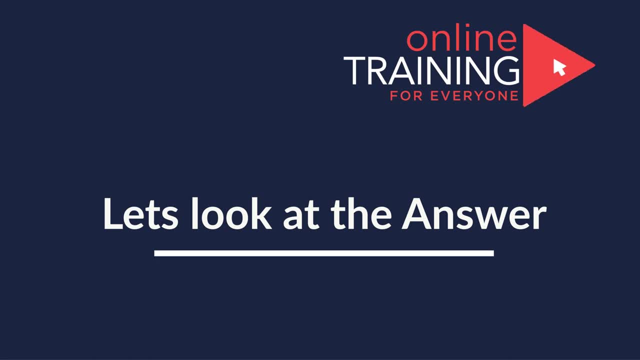 yourself some time and try to solve it. Ready or not, I'm going to move forward and reveal the correct answer, as well as the solution. As I already mentioned, this is a multi-tiered question and it requires you to do multiple 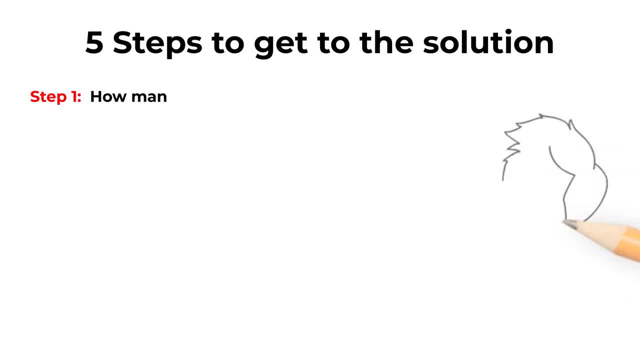 calculations to get to the correct answer. So the first calculation we would need to do is how many questions have already been answered correctly by the candidate, And the answer is calculated by multiplying 20 questions by 60%. So the answer is 12 questions. 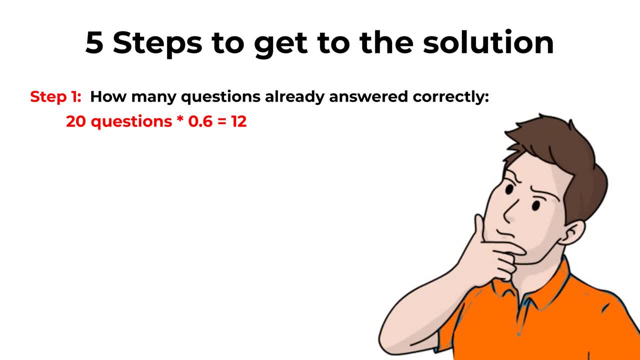 have already been answered correctly so far by the candidate. In the next phase we need to determine how many remaining questions need to be answered correctly to pass the test at 70% rate. So if there are 60 questions total on the test and we need to pass, 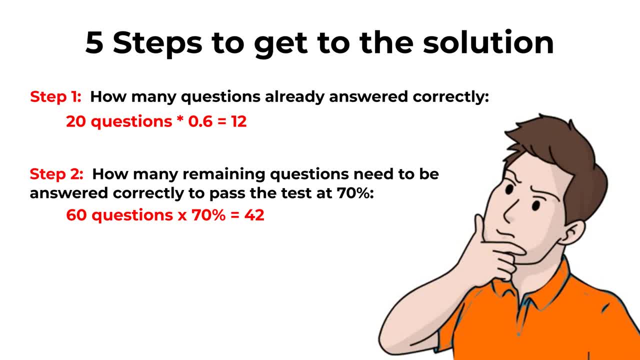 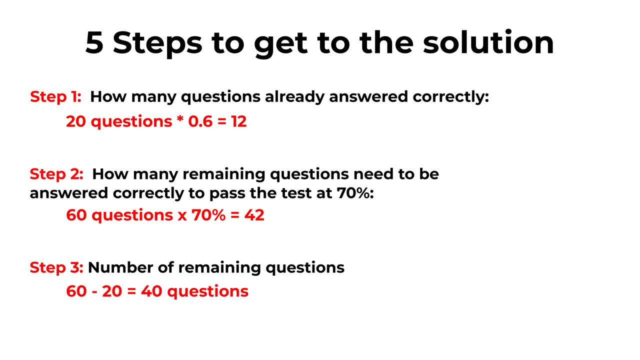 it at 70% rate, we will get to 42 questions that need to be answered correctly to get a passing rate of 70%. In the next phase we need to calculate how many remaining questions remain on the test. To do this, we need to subtract 20 from 60. And it tells us that we need to calculate. 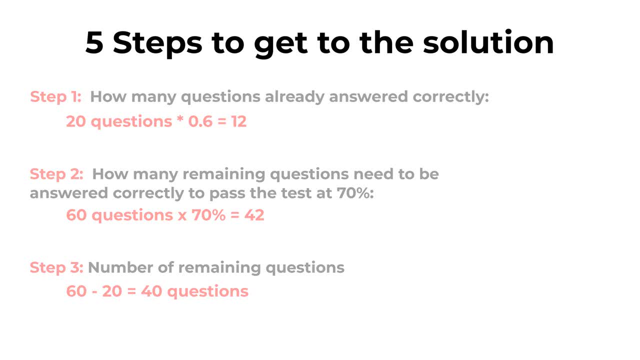 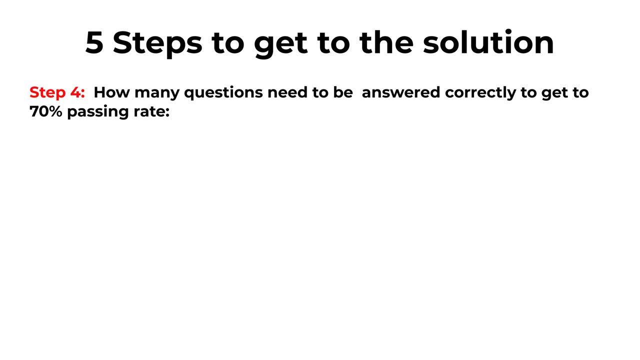 that 40 questions are still remaining. Now how many questions need to be answered correctly out of remaining questions to still get to 70% passing rate? To calculate this, we need to subtract 12, which is the number of questions we already answered correctly out of first 20. 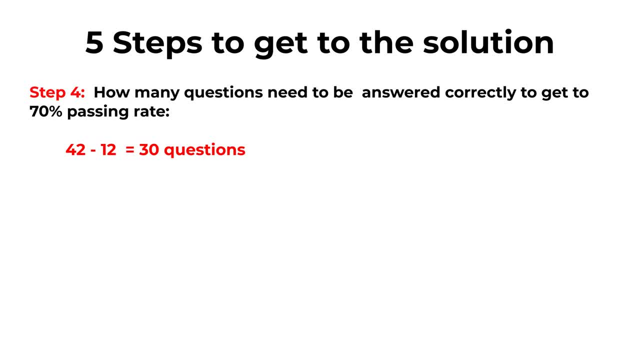 questions answered from 42. And 42 minus 12 equals 30, which means that out of remaining 40 questions, 30 questions need to be answered correctly to get to the 70% passing rate. So the last calculation we need to do is to calculate what is the percentage of. 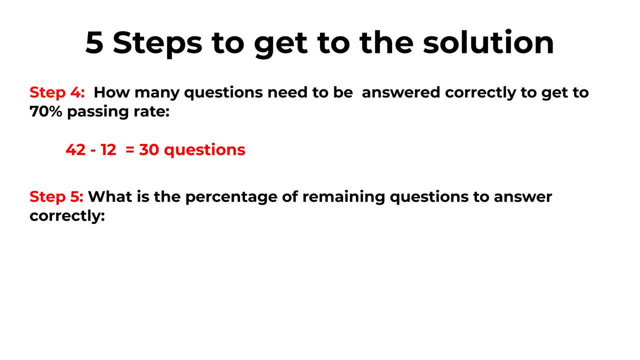 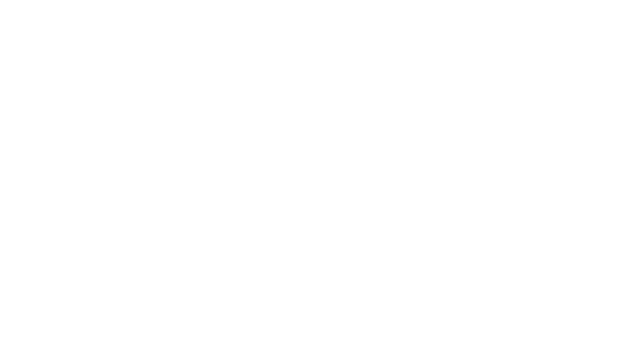 remaining questions we need to answer correctly. To do this, we need to divide 30 by 40 and multiply it by 100%, which is an equivalent of 0.75 multiplied by 100%, And the correct answer is choice D, 75%. Do you know the better way to solve this challenge? Please share your thoughts. 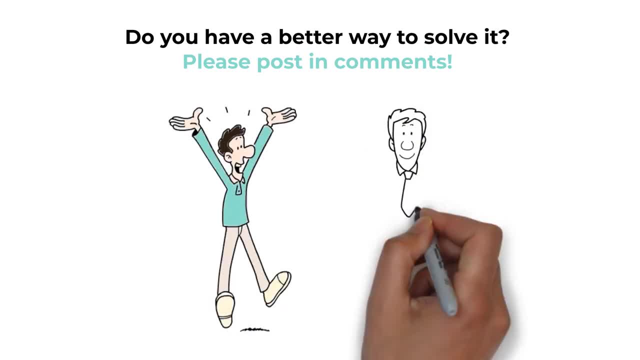 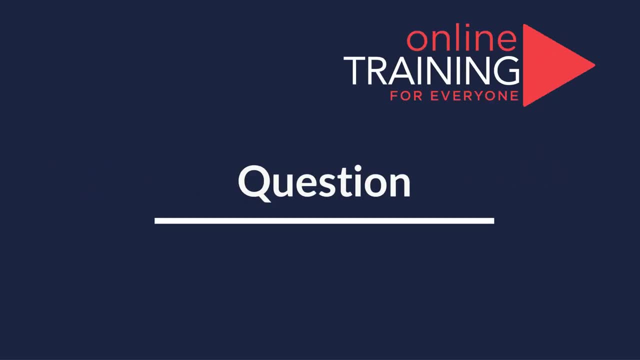 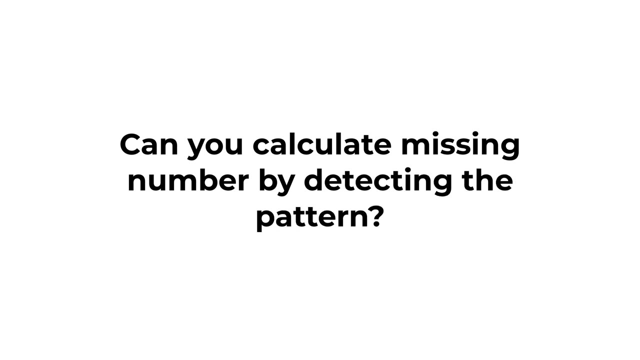 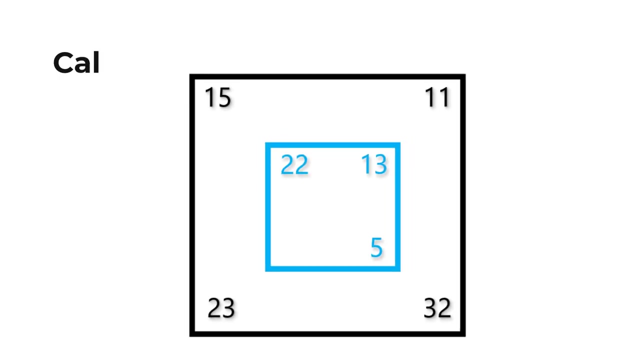 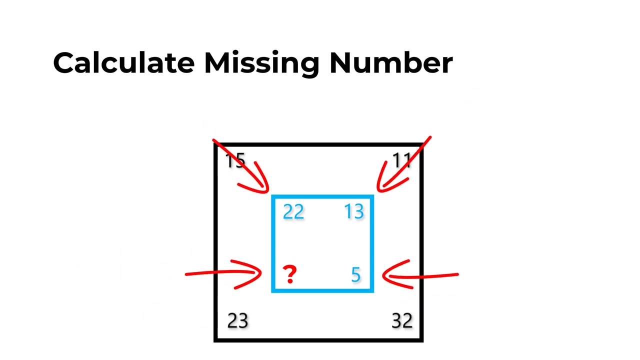 in the comment section of this video, And I hope that you never forget to like and subscribe to our channel. Thank you very much for watching and see you in the next video. Thank you very much for watching and see you in the next video. 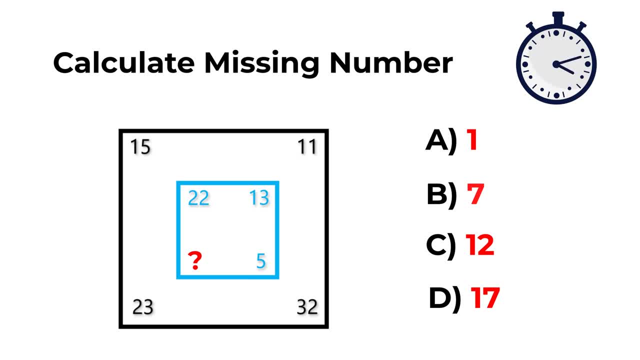 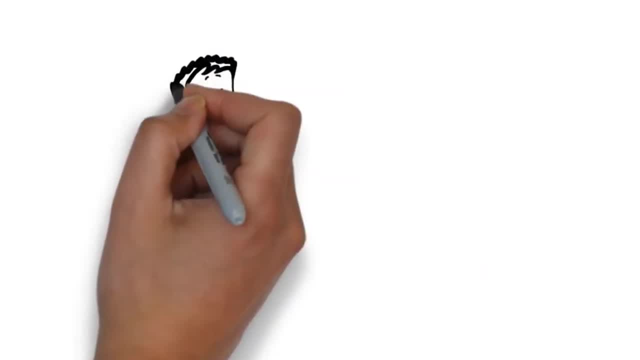 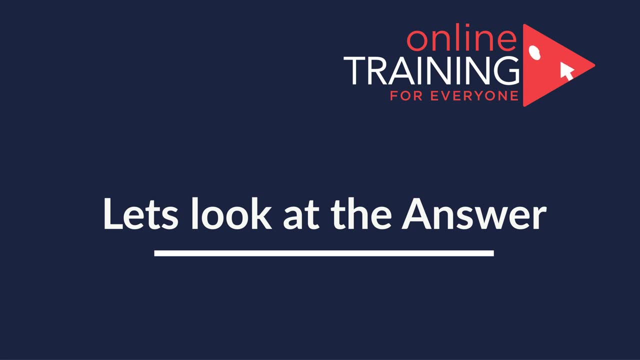 20 seconds. Possibly pause this video to see if you can come up with the answer. Do you see the pattern? Did you calculate the answer? Let's continue to see how we can get to the correct solution together. As you might have guessed, the pattern here is that the difference between 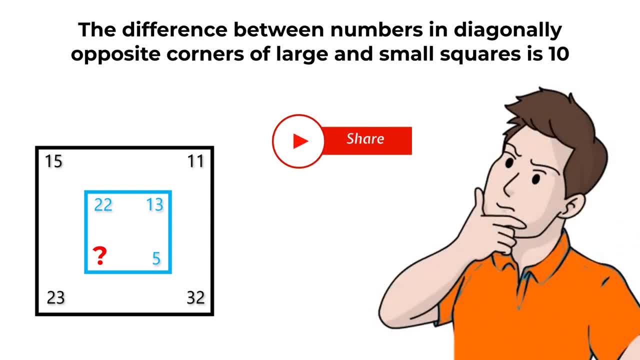 numbers in diagonally opposite corners of the larger and smaller squares is 10.. For example, at the upper left corner, the difference between 15 and 5 is 10.. If we look at the bottom right corner, the difference between 32 and 22 is 10.. And the lower left corner. the difference between 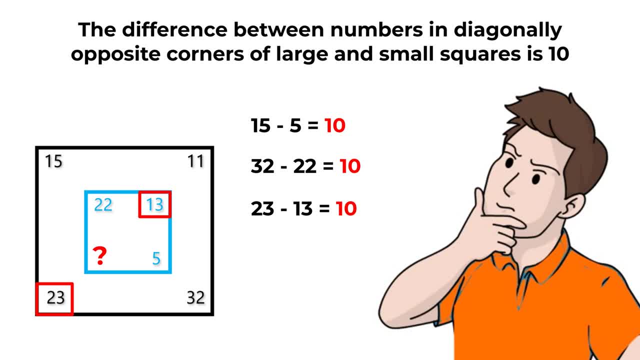 23, and 13 is 10 as well. So to calculate the missing number, we need to calculate the difference between 11 and 10.. And the difference is 1.. So the correct answer here is choice A, 1. Hopefully. 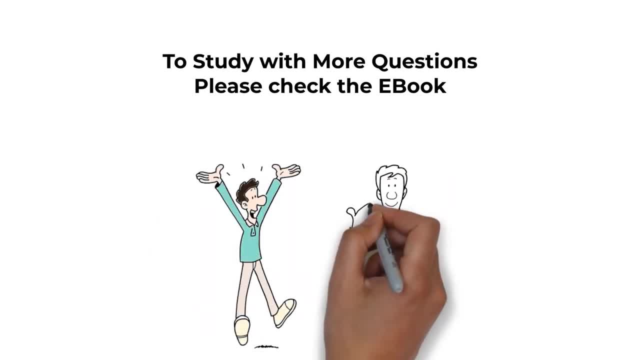 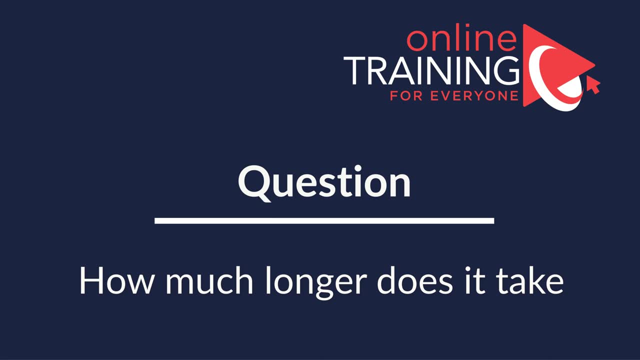 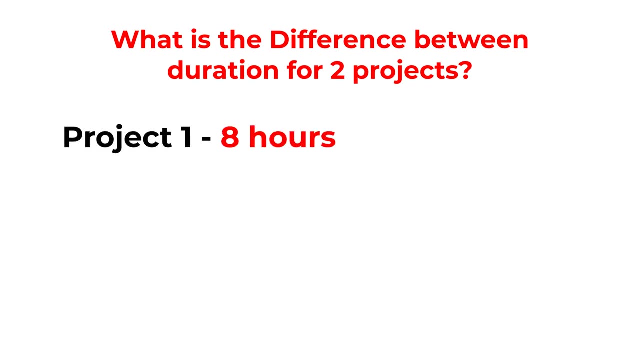 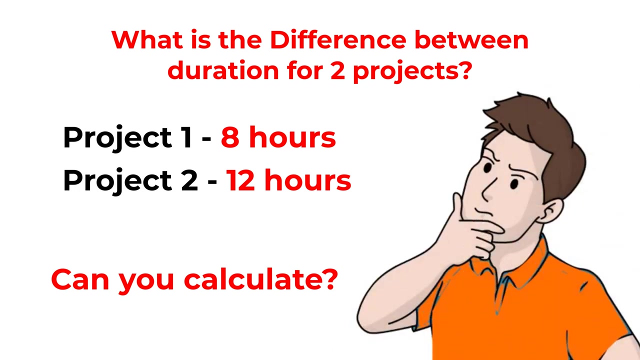 you now know how to answer similar problems on the test. Here is an interesting question which tests your understanding of percentage differences. You are presented with two projects, project 1 and project 2. And you need to calculate the difference between completion time for those two projects. It takes 8 hours to complete project 1.. 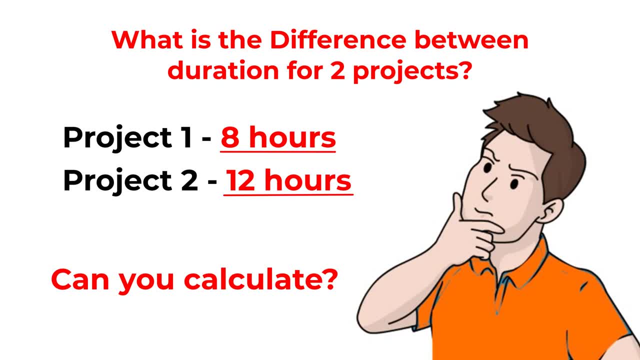 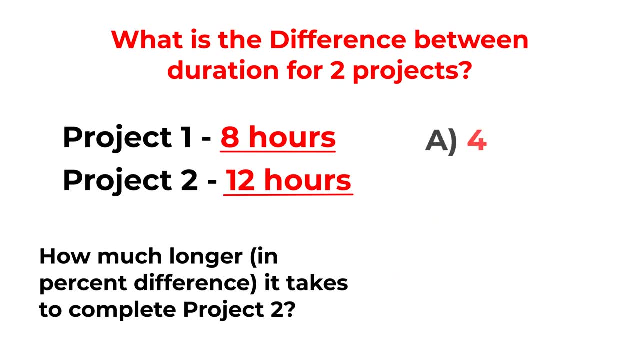 And it takes 12 hours to complete project 2.. So how much longer it takes to complete project 2?? You have four different choices: Choice A 4%, Choice B 50%, Choice C- 100%, And then choice D. 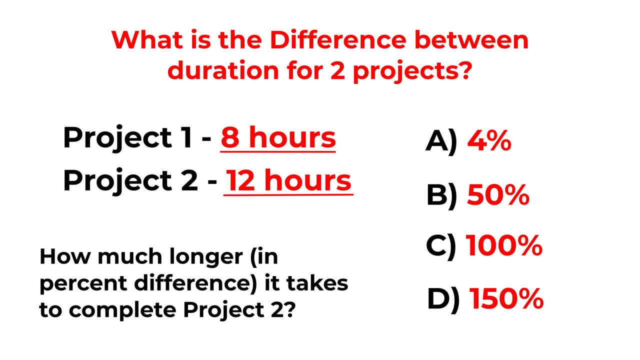 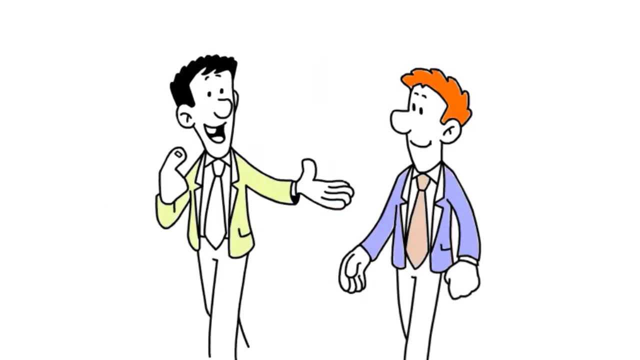 150%. Do you see the answer? Give yourself 10 to 15 seconds to see if you can do mental math and calculate the percentage differences. The answer might be a little trickier than you think. Are you ready? Let's continue to see how we can get to the correct solution together. 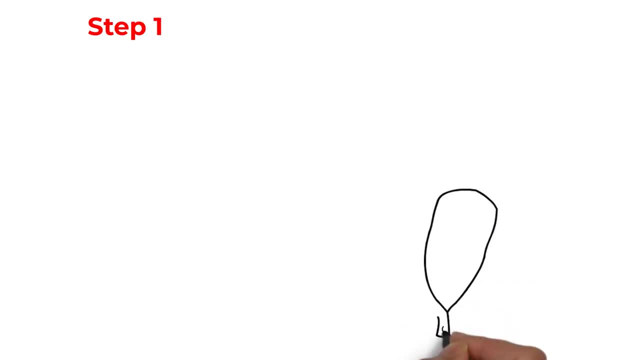 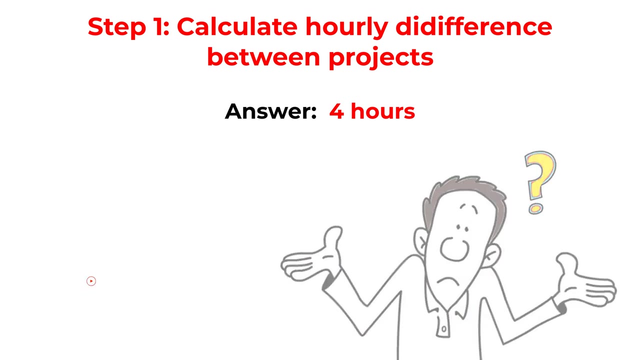 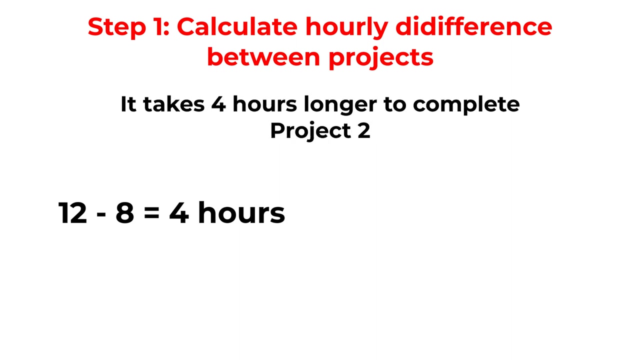 To get to the correct answer, we first need to understand the difference in hours between the two projects. The difference is 4 hours And it is calculated by subtracting 8 from 12.. 12 minus 8 equals 4.. And that is the difference between project 1 and project 2 hours. 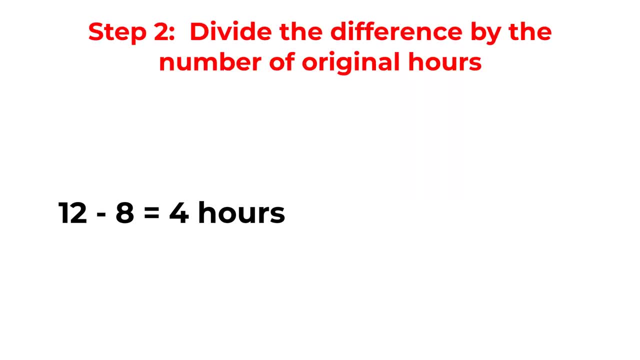 In the second step we need to divide the difference by the number of original hours, And the original hours would be project 1 hours. 4 divided by 8 is 0.5. And then we need to multiply 0.5 by 100%. So the correct answer here is choice B: 50% increase. 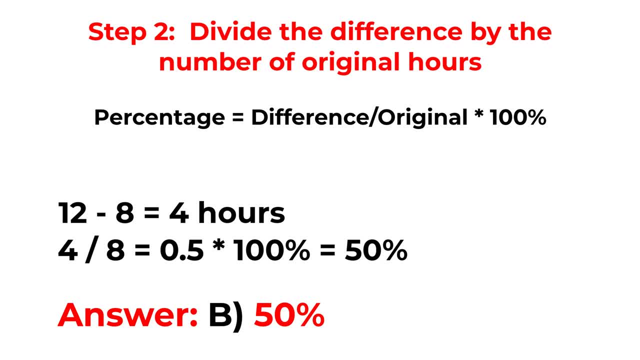 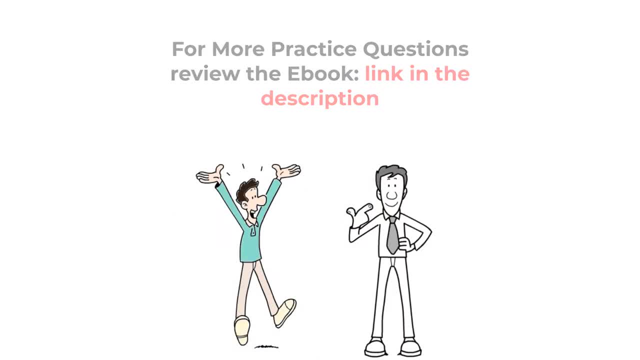 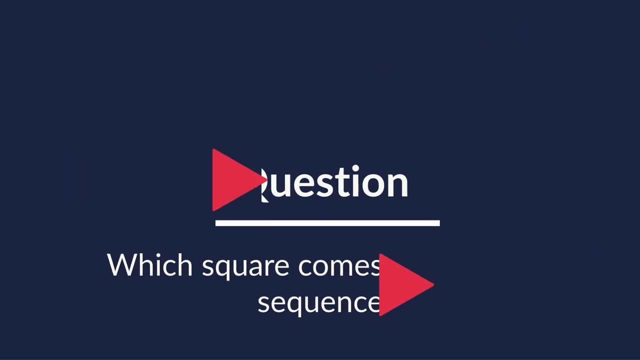 Hopefully you've nailed this question and now know how to answer similar problems on the test. It is guaranteed that you will get questions like this almost on any test. You are presented with different shapes And you need to identify the missing shape in this sequence You are presented. 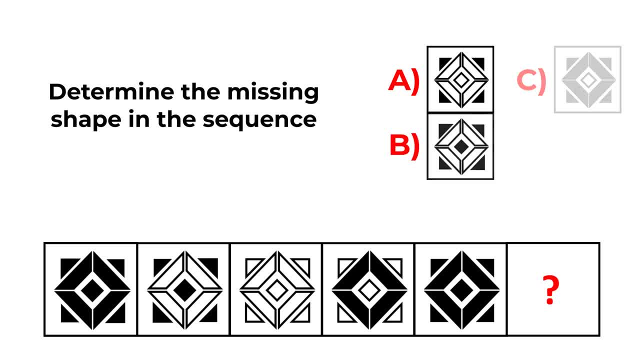 with four different choices: Choices A, B, C and D. Obviously, you need to look and identify the pattern. Do you see the pattern? Let's continue to see how we can get to the correct solution and solve this challenge together. Let's continue to see how we can get to the correct solution and solve this challenge together. 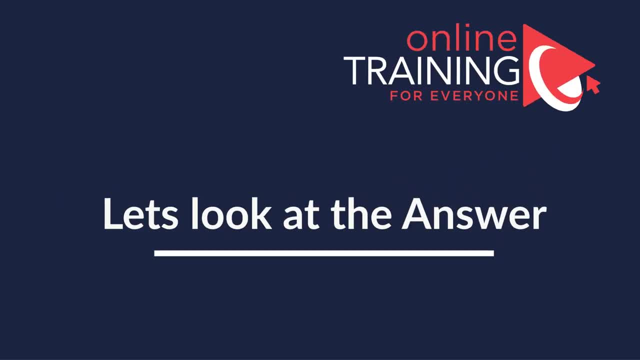 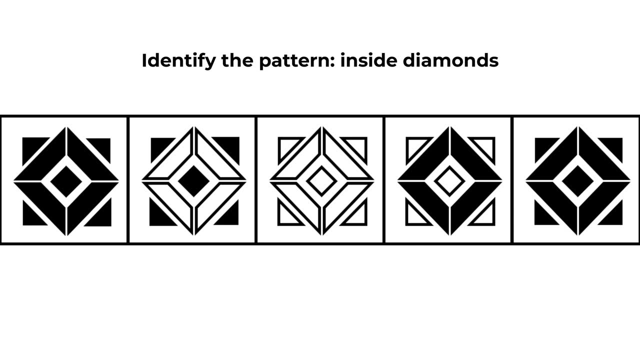 Let me first explain you the different shapes we see in the picture. Let's start with the inside diamond. You see that inside small diamond changes the colors. We have two black inside diamonds, then two white inside diamonds and then inside diamond in the shape 5 is also black, Do you see? 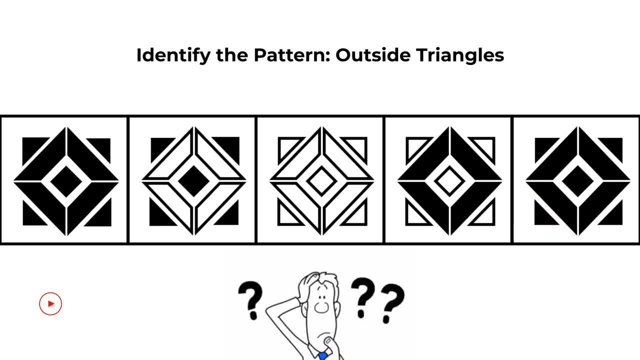 the pattern. Now there is also a pattern of outside triangles. You see that outside triangles in the shapes 1 and 2 are black, in the shapes 3 and 4 are white and in the shape 5 are black. Does it ring a bell? Doesn't give you a pattern? And then the third. 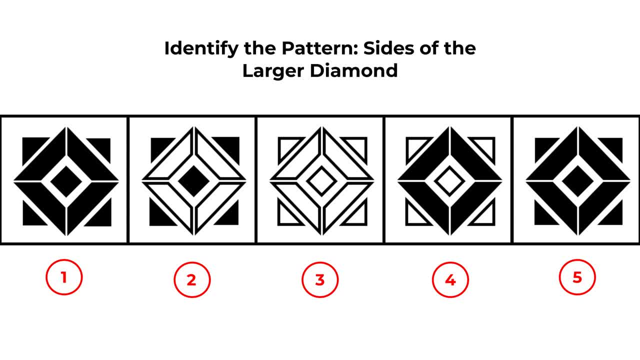 pattern are the sides of the larger diamond. If you look closely, you see that the sides of the larger diamonds in the first shape are black. then we have two white shapes and then two blacks again. Let's recap: Shape 2 is the first shape in the pattern. Shape 3 is the second shape in the pattern. 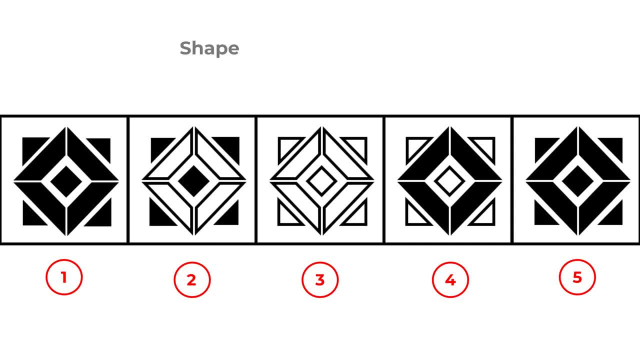 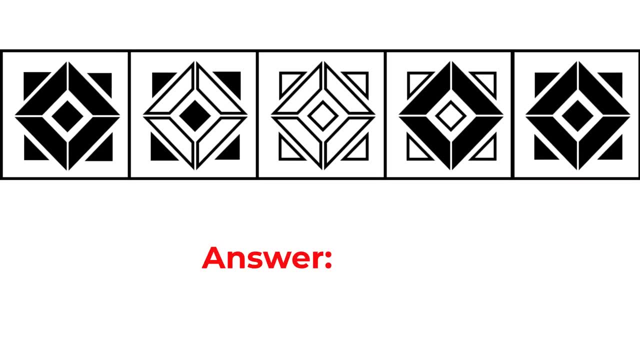 Shape 4 is the third shape in the pattern, And then shape 5 is the fourth and last step in the pattern. If you look closely at the shape 1 in the picture, you see that this represents the left shape in the pattern. So the correct choice here for shape 6 would be to select the first shape in the pattern. 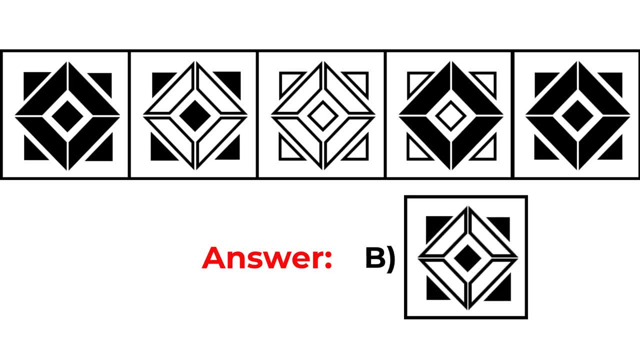 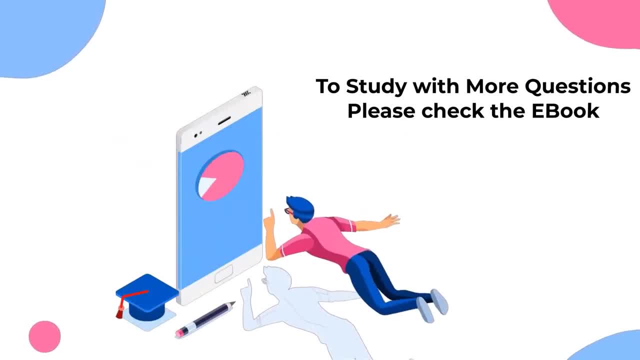 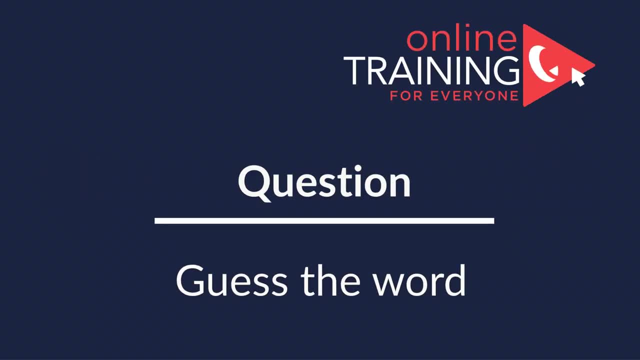 which the matching answer for the choice B. So the correct answer here is choice B. Hopefully you've nailed this question and now know how to answer similar problems on the test A lot of times. Okay, imagine presented with the question in the test that will try to determine your knowledge of English words. 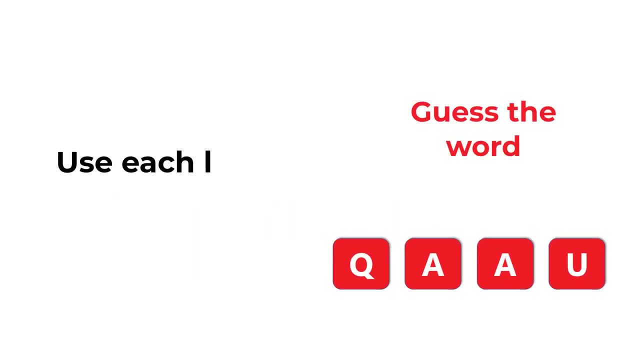 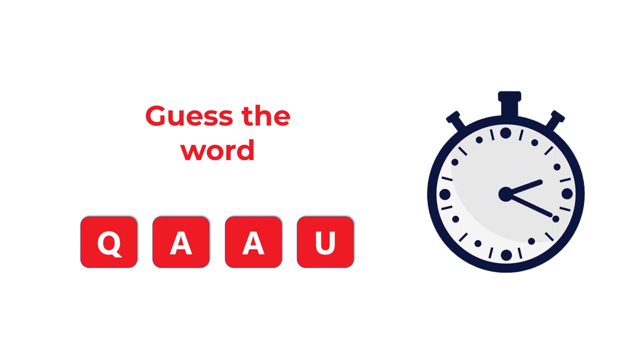 as well as how quickly you can extract these words from your memory. In this particular case, we are looking at four letters- Q, A, A and U- and you need to guess the word by combining these letters. Do you see the word? Give yourself 5 to 10 seconds to see if you can come up with the 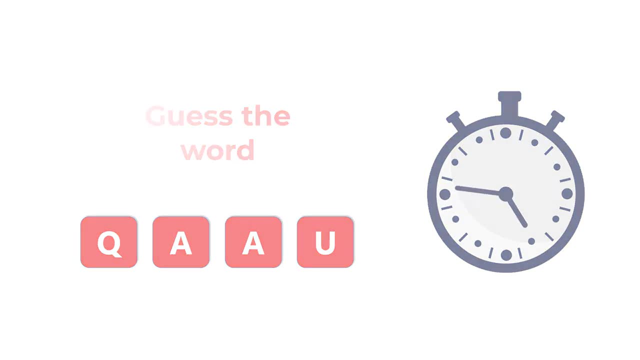 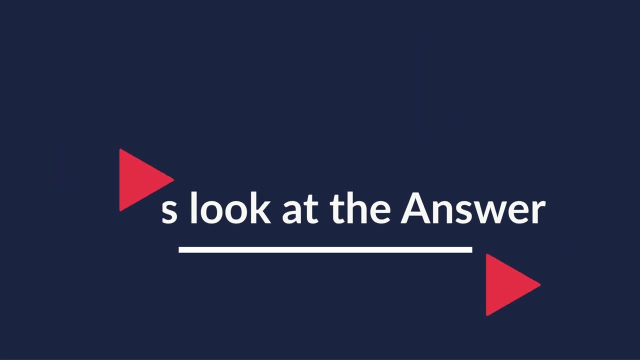 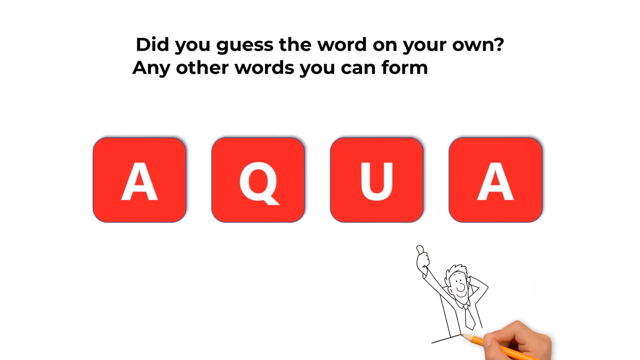 answer. Let's continue to see how we can get the correct answer together. As you might have figured out, the correct answer here is the word aqua. The spelling of the final word is A-Q-U-A, and you can get to the correct answer by rearranging the letters on the screen. 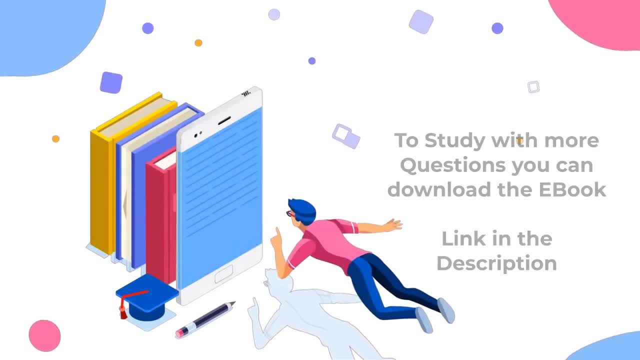 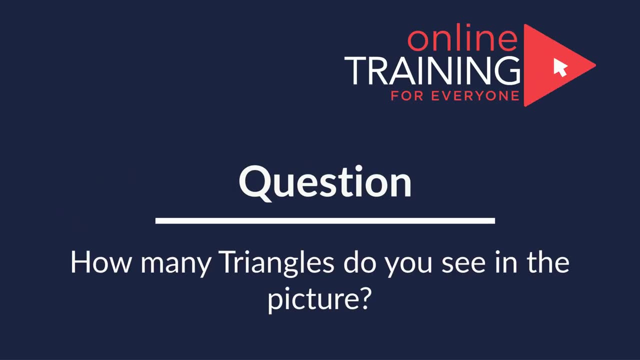 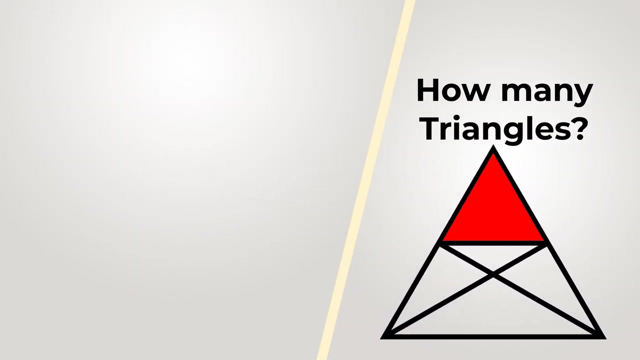 Hopefully you've nailed this question and now know how to answer similar problems in the test. This is one of my favorite questions and there is a very high chance that you will get it. Let's get started on the assessment test. How many triangles do you see? You are presented. 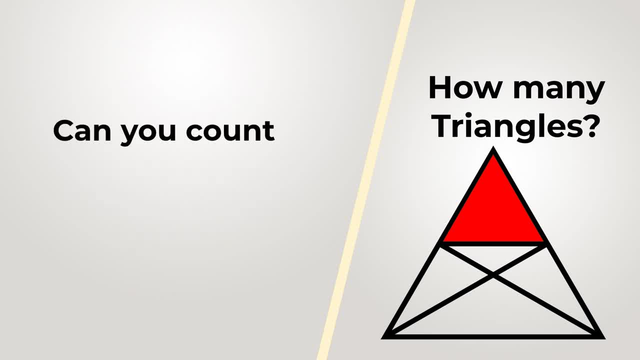 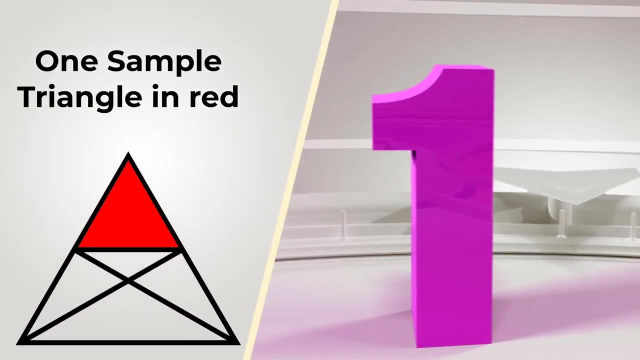 with the shape on the left, There are large triangles and there are also lines inside of these large triangles. You have four different choices: Choice A: 9 triangles. Choice B, 12. Choice C: 17. And choice D: 24. One triangle is highlighted in red, but there are a lot of other. 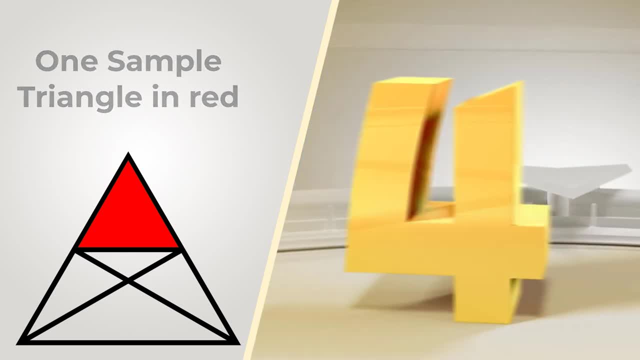 triangles. Do you think you know the answer? Give yourself a few seconds. I would recommend 10 to 15 seconds. Do you think you know the answer? Give yourself a few seconds. I would recommend 10 to 15 seconds. Do you think you know the answer? Give yourself a few seconds. I would recommend 10 to 15. 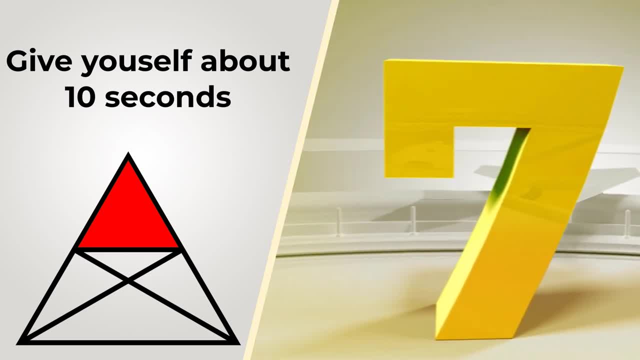 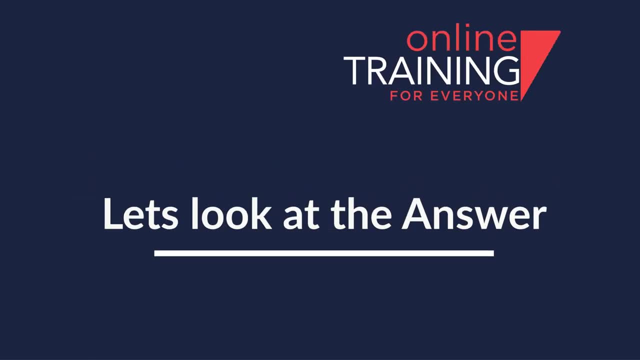 seconds. Do you think you know the answer? Give yourself a few seconds. This is about as much time as you will get in the real test. You can pause this video to give yourself some time to figure out the answer. I am going to continue and reveal the correct solution so we can get to the answer. 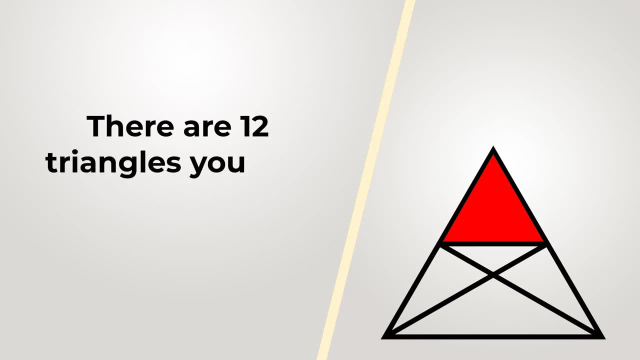 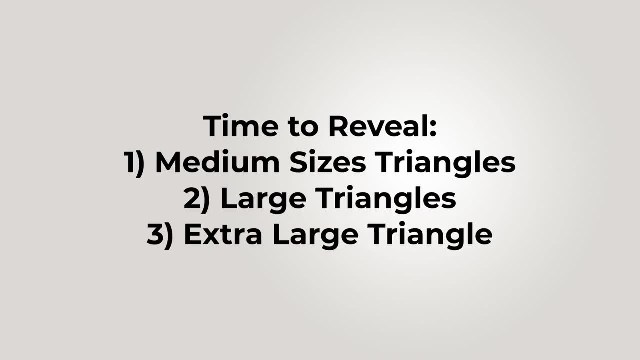 together. I counted 12 triangles in this picture. Is this what you got too? Let me show them all for you. I'll start with the smaller triangles and then go to the medium-sized ones and then go to the large ones. One, two, three, four, five, six, seven, eight, nine, ten, eleven, twelve, twelve. 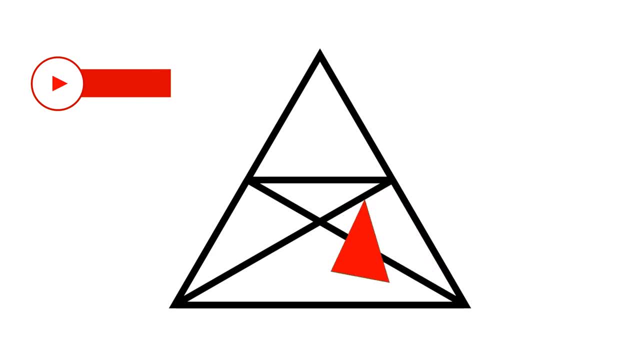 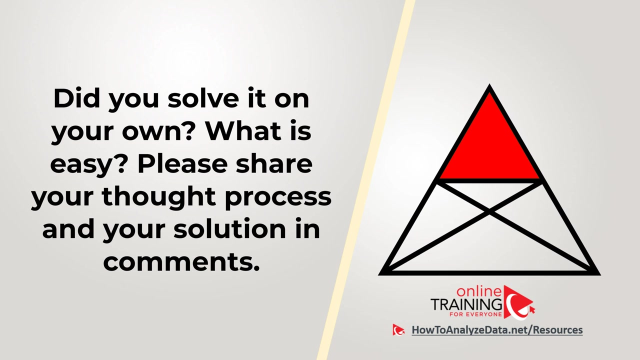 one, two, three, four, five, six, seven, eight, nine, ten, eleven, twelve. Did you come up with the different answer? Please share your thought process in the comment section of this video, so we can all learn from your perspective. Hopefully you nailed this question and got to the 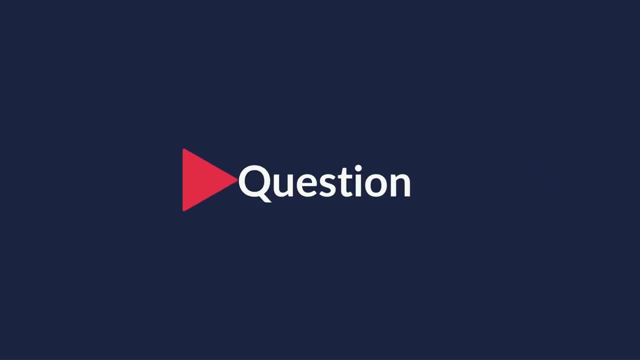 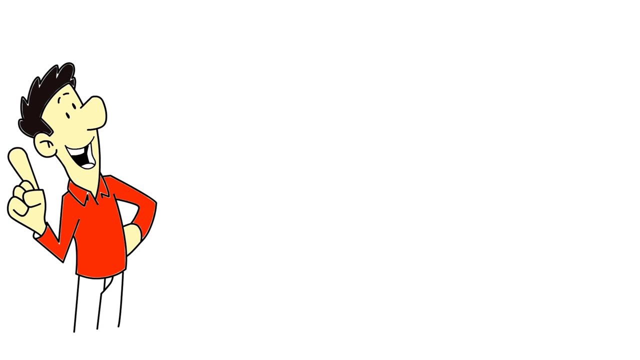 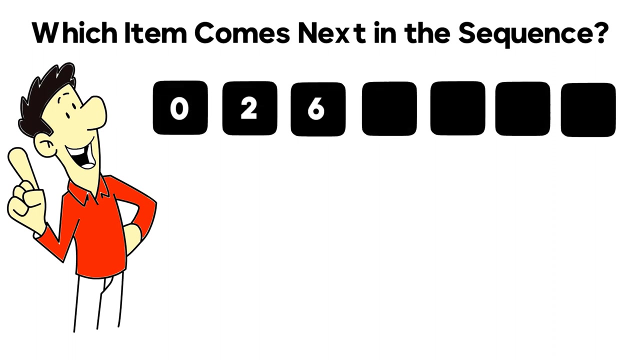 correct answer on your own. Very frequently on the test you might be asked to detect the pattern. In this question we are being asked which item comes next in the sequence And we are presented with the sequence of items. Six items in the sequence are visible: Zero, two, six, twelve. 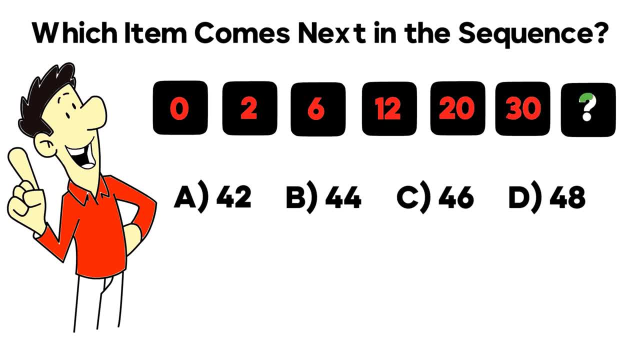 twenty and thirty, And the next item is missing And you are being asked to select one of the four following choices: Choice A- 42.. Choice B- 44.. Choice C- 46. And choice D- 48.. Do you see the answer? 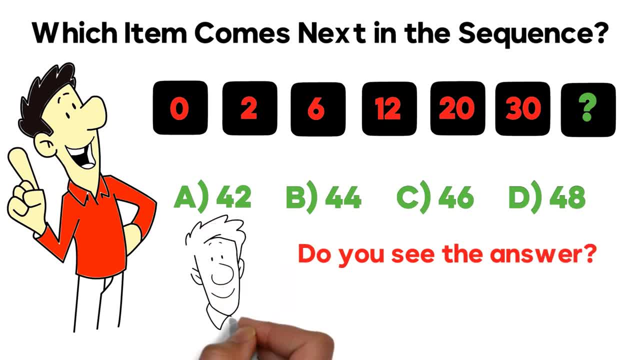 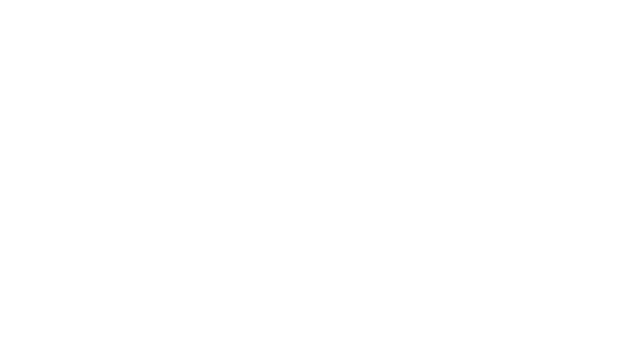 It may or may not be obvious, depending upon your skills of detecting the pattern, Like it or not. we are going to continue and I'll share with you the answer. So who's going to answer first? As with any type of question, 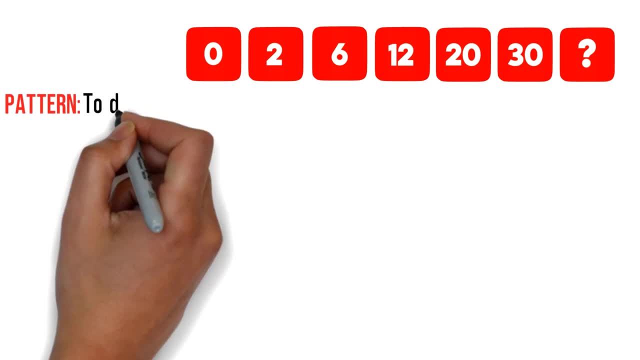 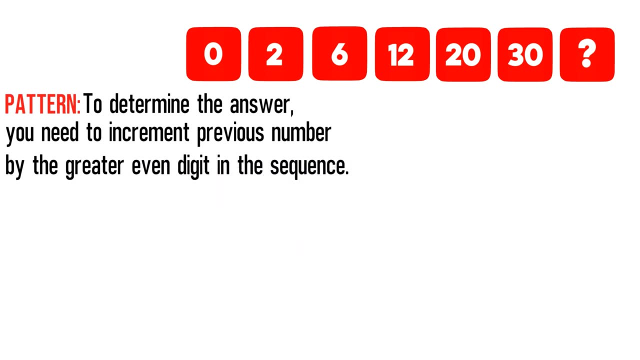 the key is to determine the pattern, To determine the answer. in this particular case, you need to increment previous number by the greater event digit in the sequence. As with any type of question, the key is to determine the pattern, To determine the answer. 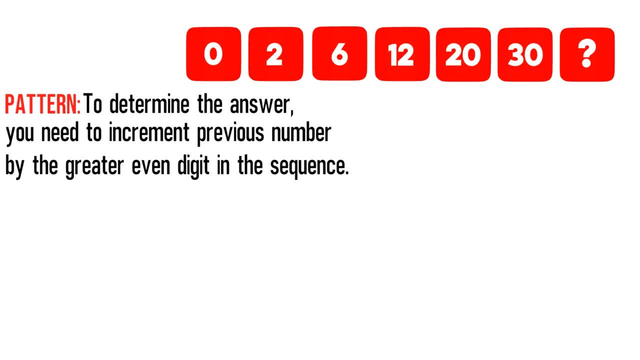 to this particular case, you need to increment previous number by the greater event digit in the sequence. You can even come up with the formula, And in our case, the formula to determine the next number would be current number plus two multiplied by current position. 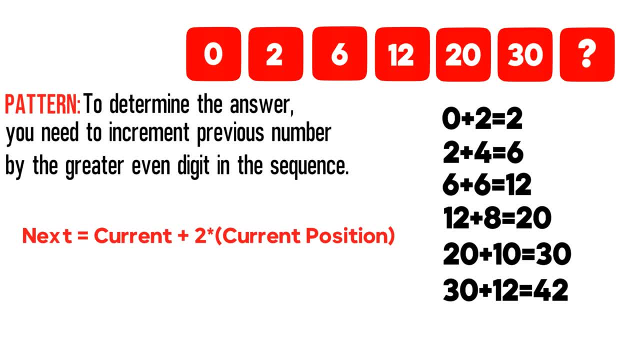 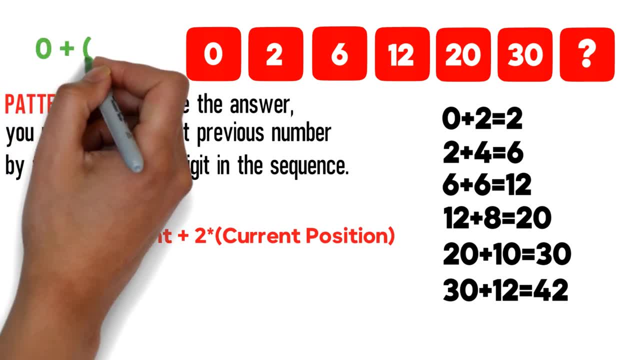 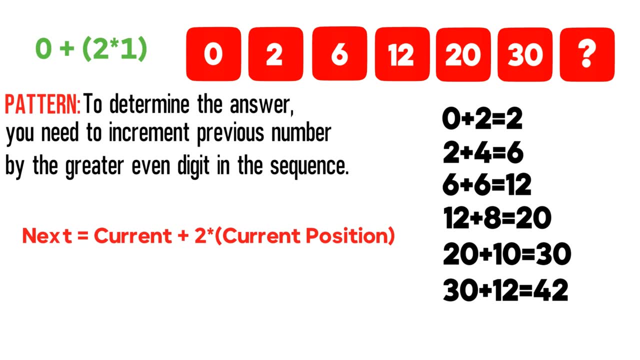 So let's see how it works. For example, let's take the number zero. This is the first number in the sequence. To determine the next number in the sequence, we need to add the previous number, which is 0, and then 2 multiplied by 1, because number 0 has the first position in the sequence. 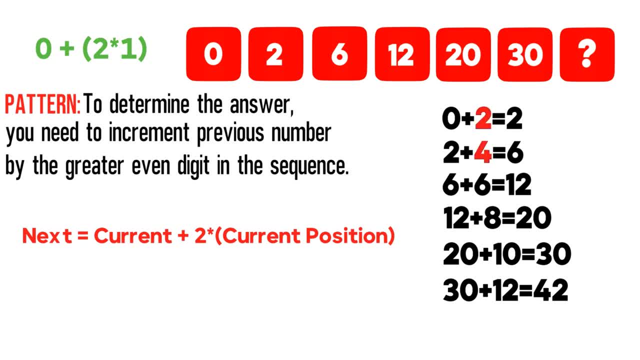 Instead of using the formula, you can also use the next even number and add it to the previous number. The even numbers are 2,, 4,, 6, and you can increment them down the list, So you can add 2 to 0,. the next one would be 4,. 2 plus 4 equals 6,. the next number would be 6,. 6 plus 6 is 12,. 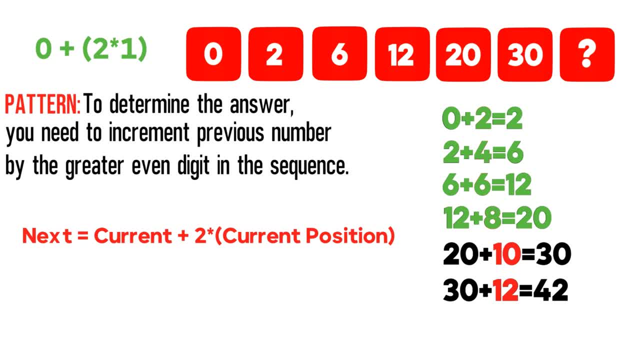 the next number would be 8, and 12 plus 8 equals 20.. The number after that would be 10,, so 20 plus 10 would be 30,, and the number after that would be 12, and 30 plus 12 equals 42.. 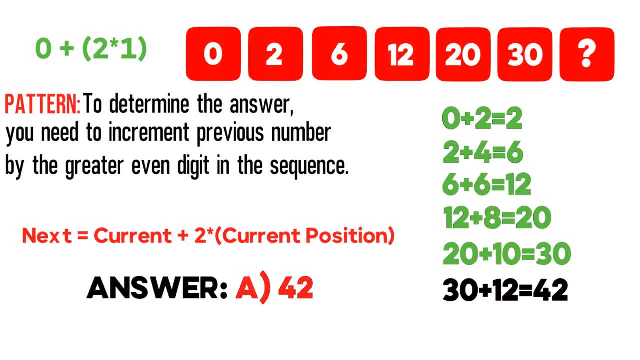 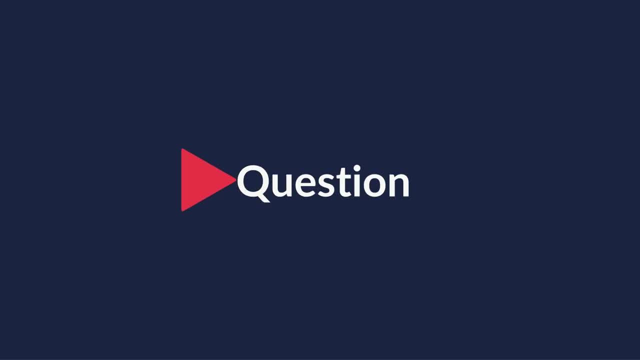 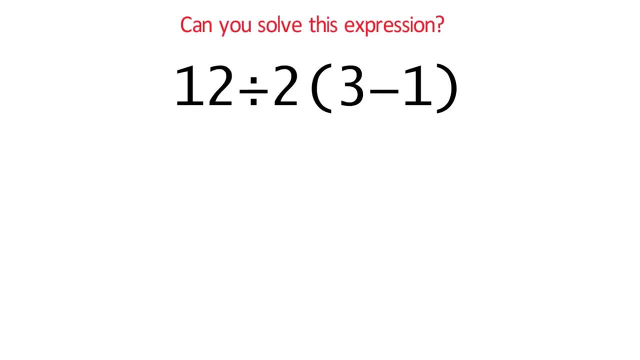 The correct choice here is choice A 42.. Hopefully you've nailed this question and now know how to answer similar problems on the test. Here's the interesting question, which is easy to understand but at the same time you will have a lot of fun solving it. You need to calculate this simple expression: 12 divided by 2. 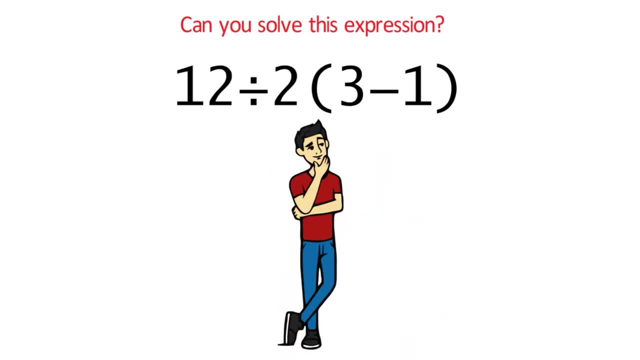 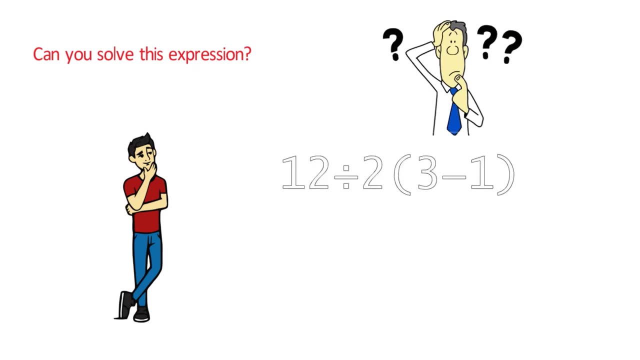 and then multiplied on the value in parentheses, which is 3 minus 1.. Take a look closely and see if you can come up with the answer. There are three operations here: division, multiplication and subtraction. All you need to do is to write the answer in the following order: 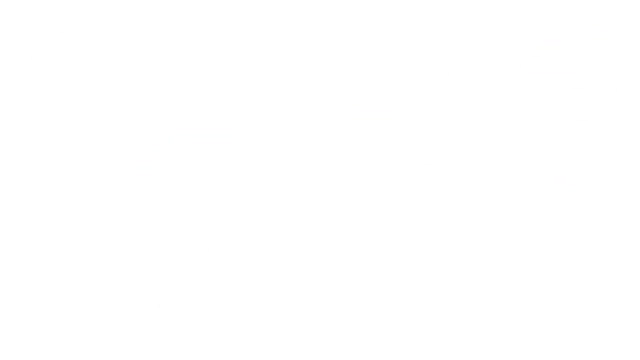 to determine is which one to do first, second and third. do you think you know the answer? let's continue and get it solved together. the order of operations in math tells us that the first expression we need to solve is in parentheses. we first need to calculate 3 minus 1 and obviously, 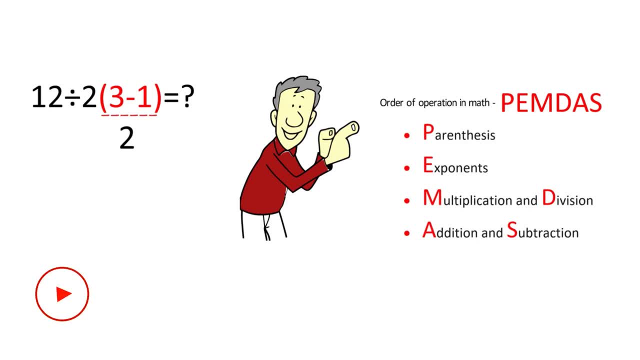 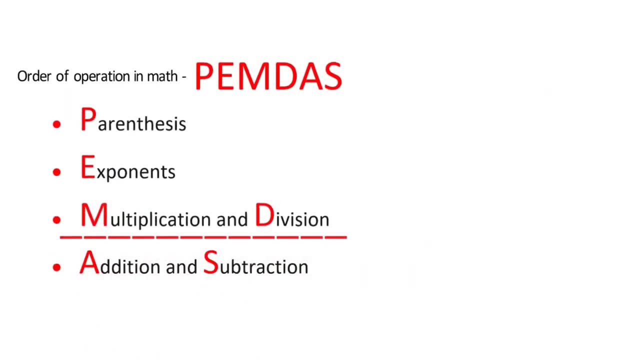 the answer is 2. the big question is: what do we do next? the order pemdes tells us that we need to do multiplication and division. but what order doesn't mention is that we need to do it from left to right. and, what's interesting, the acronym itself is a little bit confusing, because it shows: 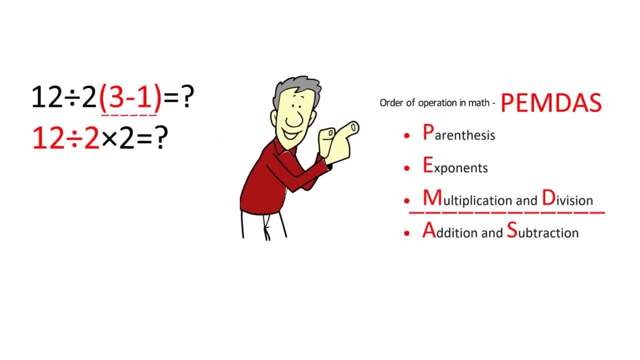 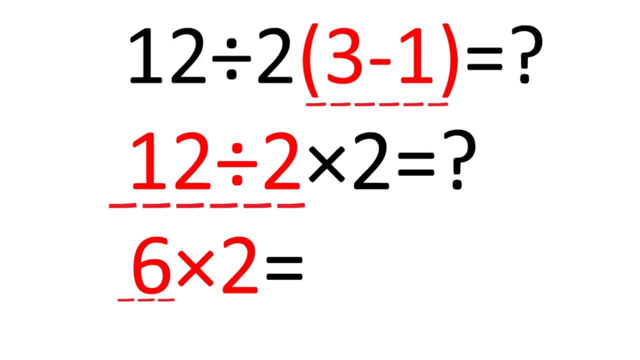 multiplication first and then division. but in our case we need to do division first and divide 12 by 2 and then do multiplication. once we divide 12 by 2, we get to 6 and the final expression we need to solve would be 6 multiplied by 2. so the correct answer here is 12.. 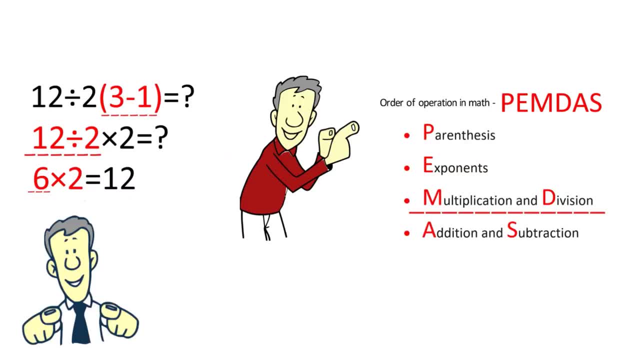 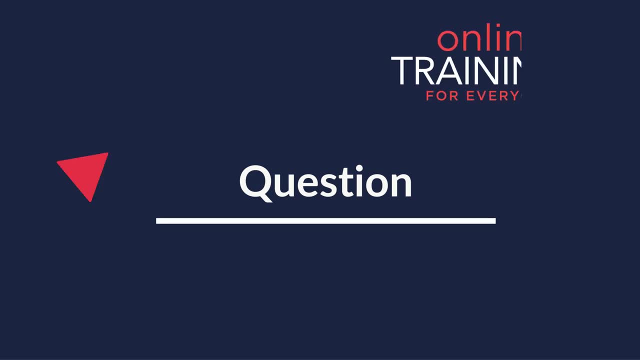 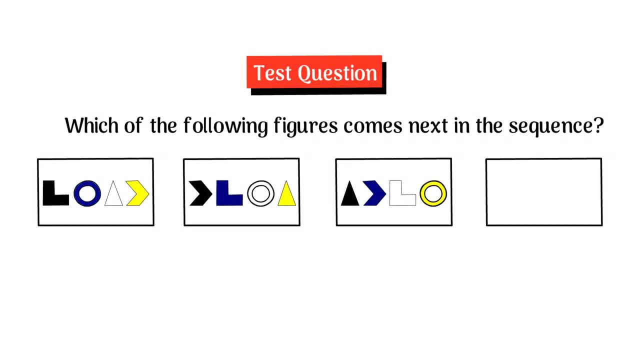 solve this challenge on your own. was it easy for you? please share your thought process and your solution in the comment section of this video. here is a very cool question that you frequently see. on the test, you are presented with four rectangles. in each one of these rectangles, 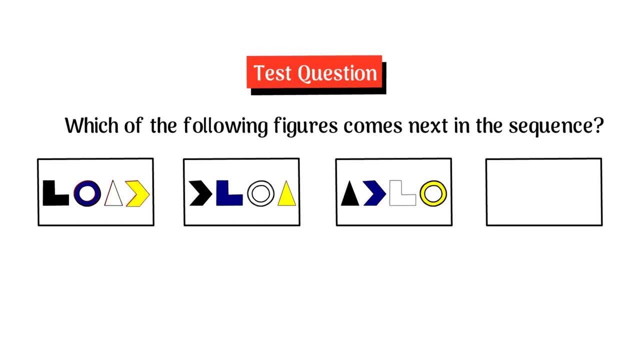 there are different shapes. each shape is of the different color. three rectangles have shapes present and force rectangle on the right has all the shapes missing. you have four different choices to identify the missing item in the sequence: choices a, b, c and d. do you think you can come up with the answer? give yourself some time. you can pause this video to see. 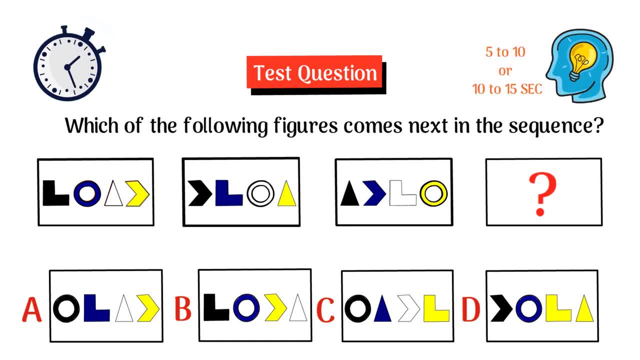 if you can identify the pattern, give yourself 5 to 10, maybe 10 to 15 seconds. this is about as much time as you will get in the real test. did you figure out the solution? let's continue to see how we can get to the correct solution together. in most types of problems there are. 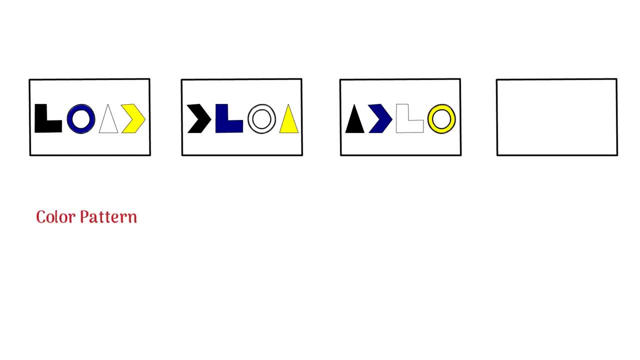 typically multiple patterns per line of this problem. there are multiple patterns per line of the pattern present. For example, let's look at the color pattern. If you look closely, you see that the first shape inside the rectangle is always black. second shape is always purple. third shape is: 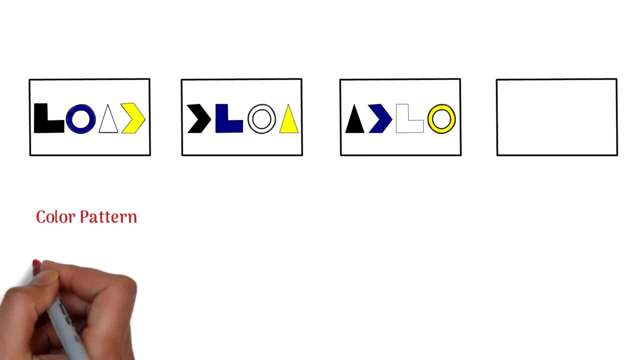 always white and the rightmost shape is always yellow. Second pattern that you can see if you look closely is the pattern of rotating shapes. You can see that the rightmost shape in the previous rectangle always becomes the leftmost shape in the next rectangle. For example, the yellow arrow. 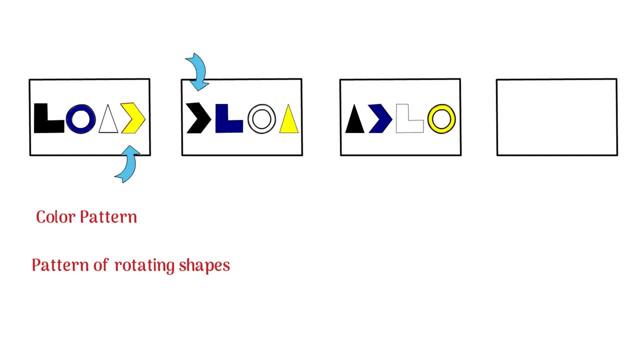 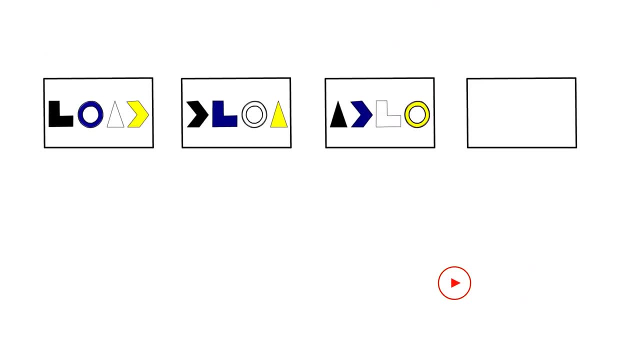 from the first rectangle becomes the black arrow in the second rectangle. If you are able to identify at least one of these patterns, you will be able to solve this problem. Let's look at each of the answers and try to exclude the incorrect answers. For example, choice A does match the 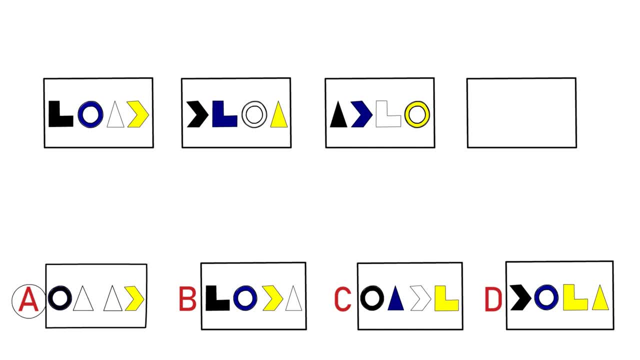 color pattern, but if you look closely, the next shape after the circle should be triangle and not the L shape as it is currently presented in the choice A. Choice B can be excluded because it doesn't match the color pattern. As you can see, the yellow shape and white shape should be swapped to match the color pattern. 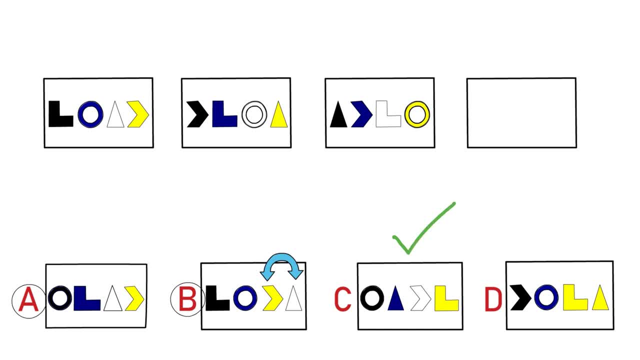 Choice C is the correct answer. It does meet requirements for both patterns And choice D does not match the color pattern. Two rightmost shapes are yellow. Hopefully you've nailed this question and now know how to answer similar problems on the test, But in case you need more questions like 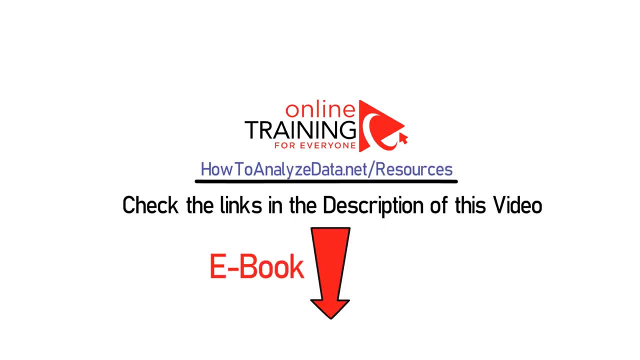 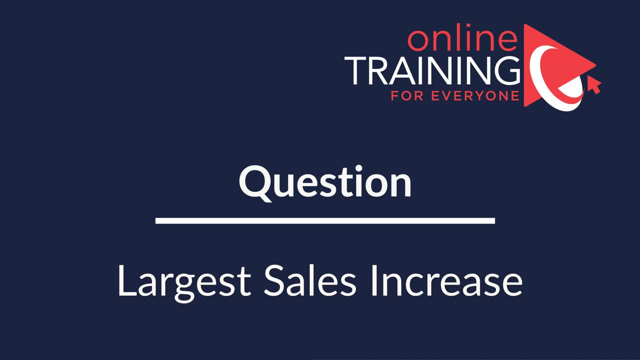 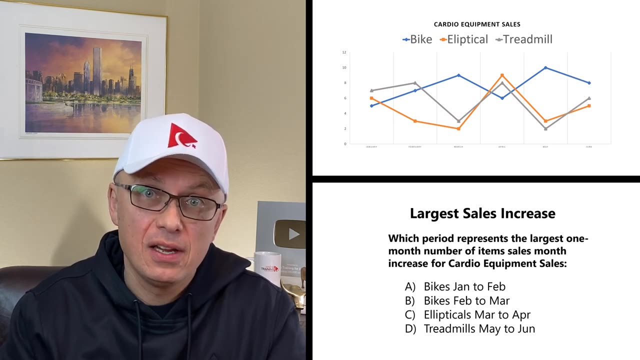 this. please make sure to check out my ebook. in the description section of this video, A lot of times you might get a question which asks you to determine the sales increase. You're typically presented with the graph which shows lines that represent different sales. In our case, 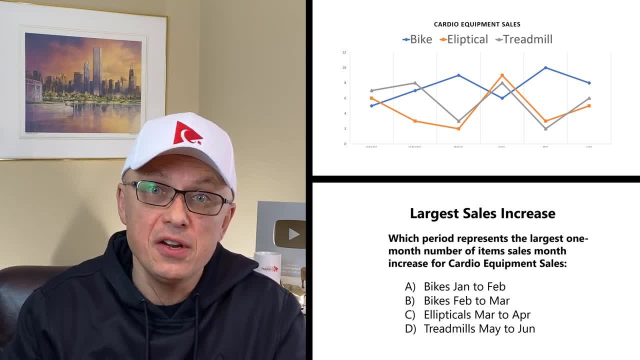 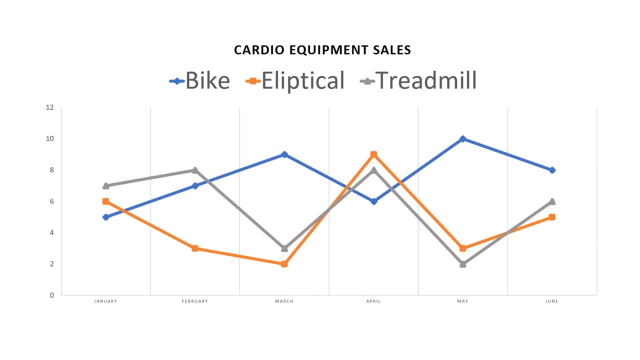 we are represented with the chart that shows sales of cardio equipment from January to June: sales of bikes represented by the blue line, sales of elliptical represented by the orange line and sales of treadmills are represented by the gray line. The question is how many sales? 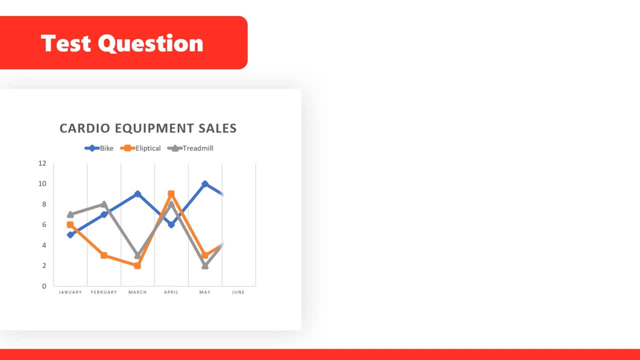 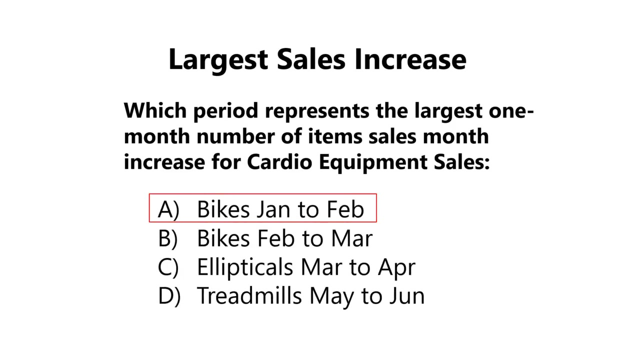 do you need to determine the largest sales increase. Specifically, you need to determine which period represents the largest one month's number of item sales increase. for cardio equipment sales, You have four different choices. Choice A: bikes from January to February. Choice B: 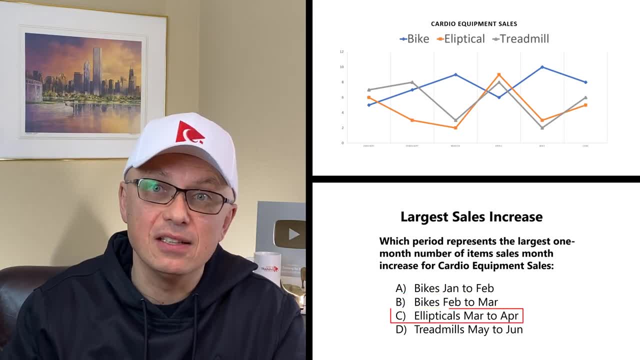 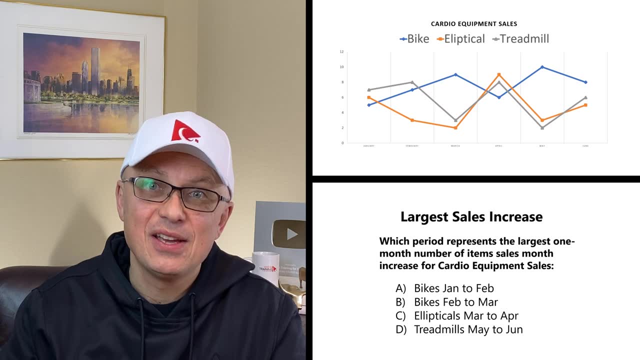 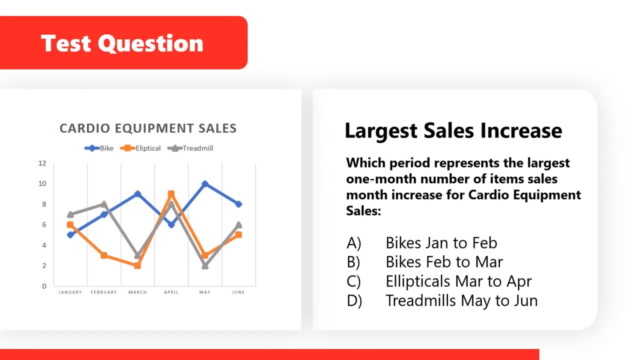 bikes from February to March, Choice C ellipticals- March to April And choice D treadmill made to June. Do you see the answer? You may need to look closely to determine the correct answer for this question. Give yourself 5 to 10 seconds to see if you can come up with the right solution. Are you ready? 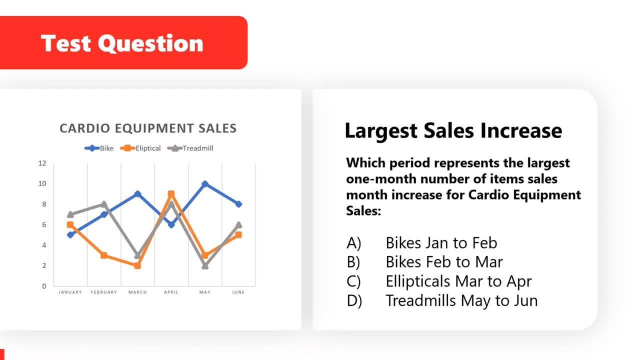 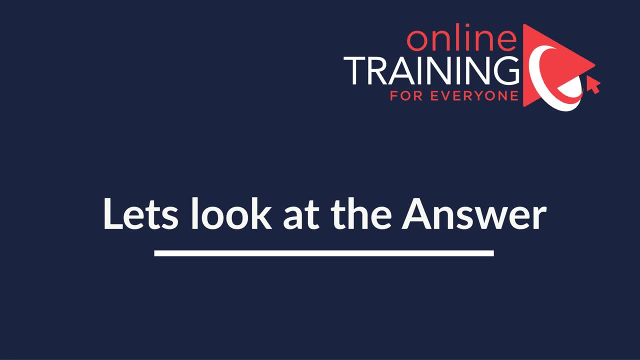 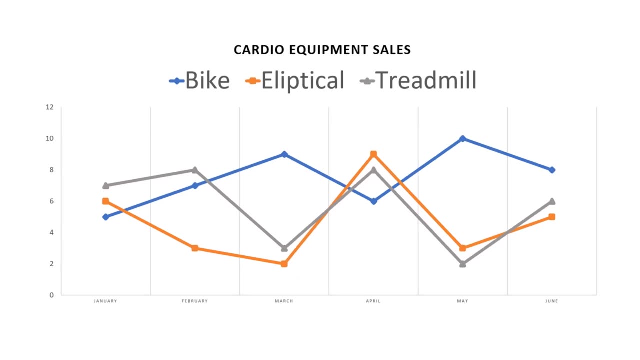 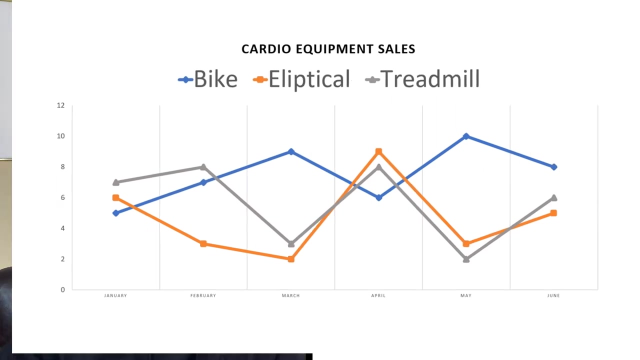 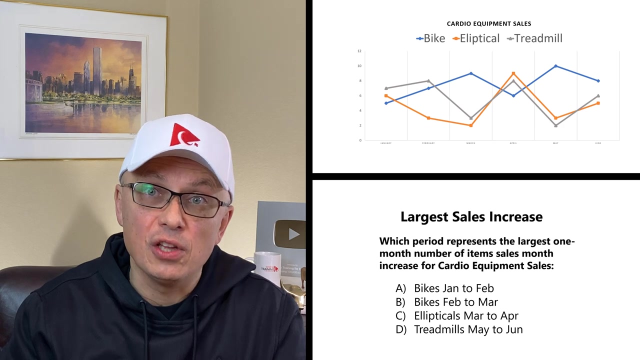 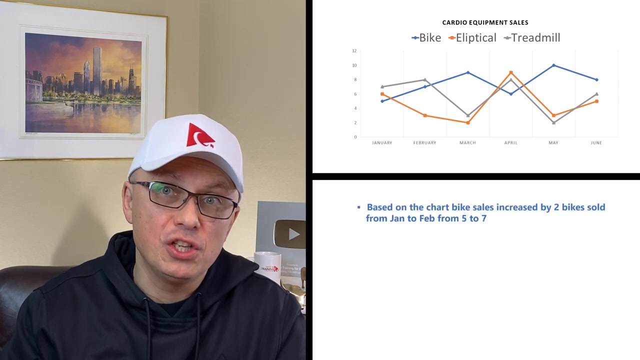 We're going to move forward and cover the answer for this problem and get to the solution together. To answer this question, we need to look at the graph closely. For each data point on this chart, we need to determine the actual value fore, اTER, cada parameter. And we need to determine the actual value. And once we have all the numbers, we need to answer that question by looking at the differences for equipment sales from months to months. Specifically, in this case, you need to evaluate four different choices that are represented by answers A through D. let's do it together, Based: on the chart. Bike Sales increased by 2 from January to February and the increase was from 5 to 7 items sold. Bike Sales also increased by 46.8 items sold by 12.6 items and the increase came from 49.5 items. gauche: 1 item: less than 25 items sold. 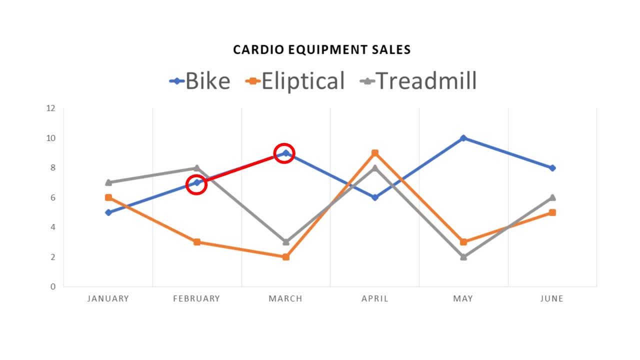 increased by two from seven to nine between February and March. elliptical sales, on the other hand, increased by seven from March to April, jumping from two to nine, and treadmill sales increased by four. between me and you went up from two to six. so the correct answer here is choice C: elliptical sales. 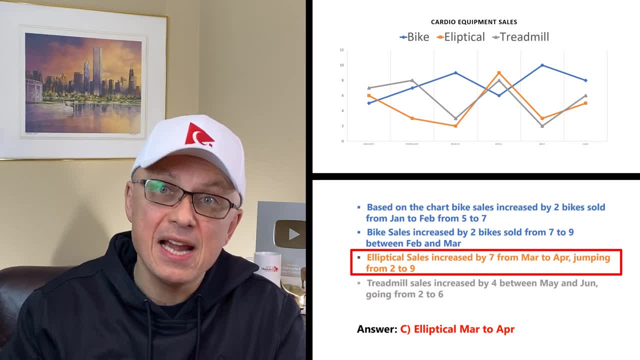 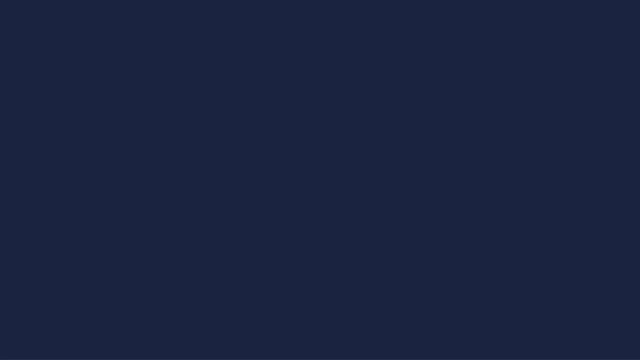 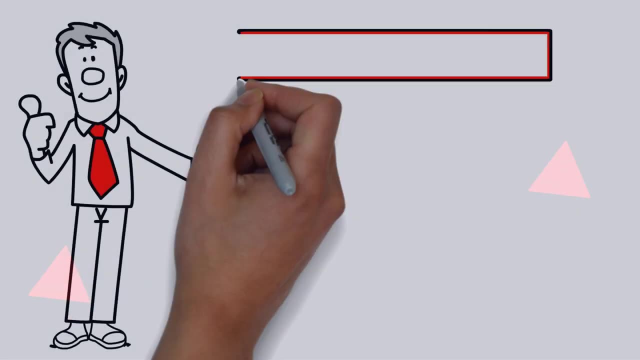 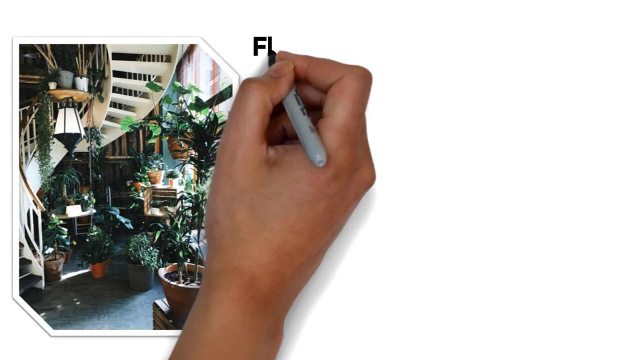 from March to April because jump was by seven from two to nine. hopefully it nailed this question and now know how to answer similar problems on the test. I am very excited to present you with simple but at the same time very tricky question which tests your math skills as well as attention to details. florist has 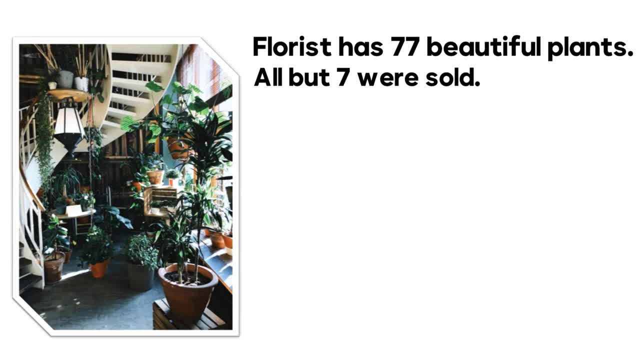 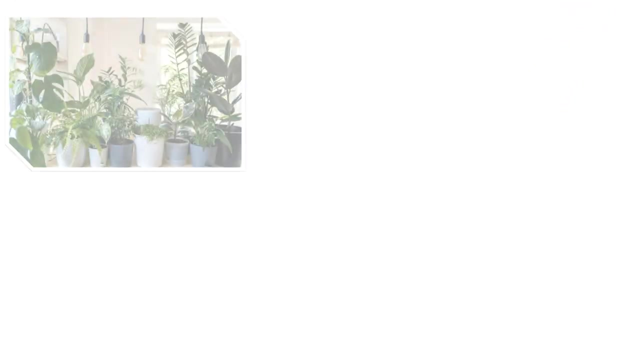 seventy seven beautiful plants- all but seven- were sold. how many plants are left? you have four different choices: choice a: seven, choice B: 77, choice C: 70 and choice D: 84. do you think you know the answer? let's continue to see how we can get to the correct solution together. the answer to this: 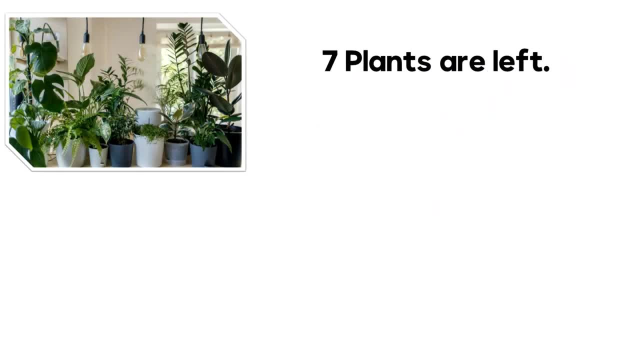 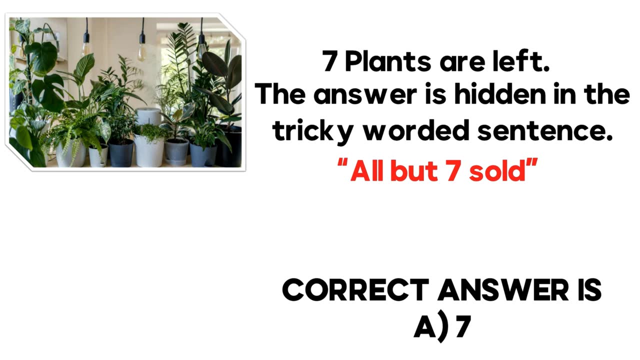 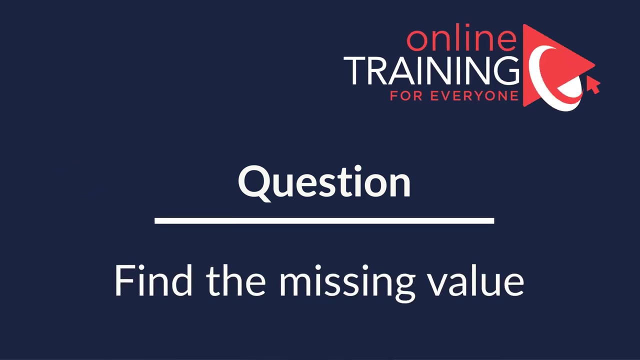 question is very simple: seven plants are left. the answer is hidden in the tricky worded sentence: all but seven were sold, so the correct answer here is choice a: seven. hopefully you've read this question correctly, understood it very well and solved it on your own. you're going to love this problem because it is so confusing you're. 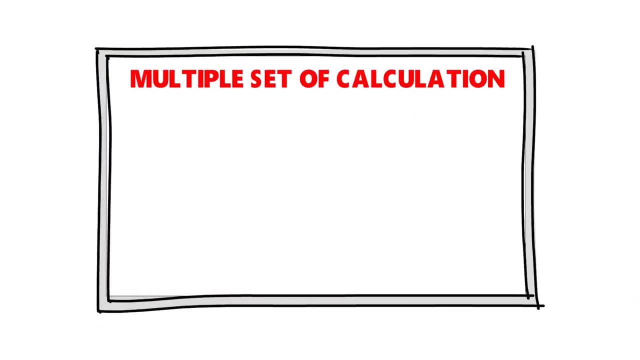 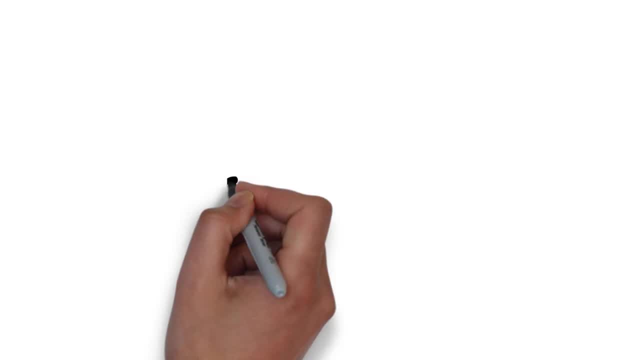 presented with multiple set of calculations. in our case, we have two full calculations and one calculation is missing. the final value, the first calculation is 22 multiplied by 22 equals 16.. second calculation is: 33 multiplied by 33 equals 36. and then the 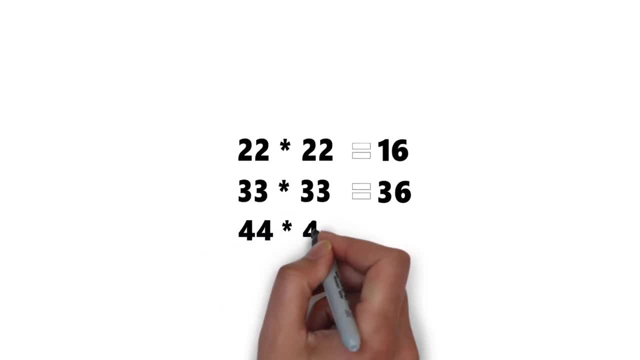 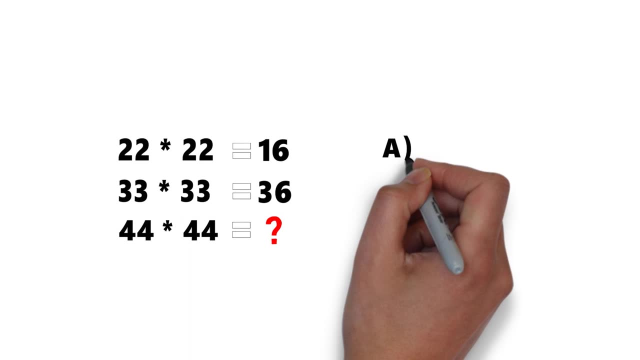 last calculation is 44 multiplied by 44 equals question mark, and you need to calculate question mark. you have four different choices: choice a 52, choice b 56, choice C, 60 and choose D, 64. do you see the answer? it's not obvious. so give yourself 52, two 3NP, molecular mattered time as number, often spelled with an Amazon矢 Nam. NOW YOU READ THIS PIEсь formula for a question mark: is文-von livingbrush useres have a her. they give out simple choice rather than a final answer or answer f seeking images. if I only add a million this time, you know the answer for question marks. do you understand that? see the thấy. 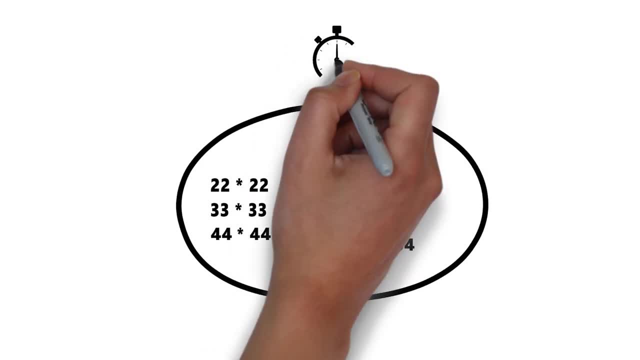 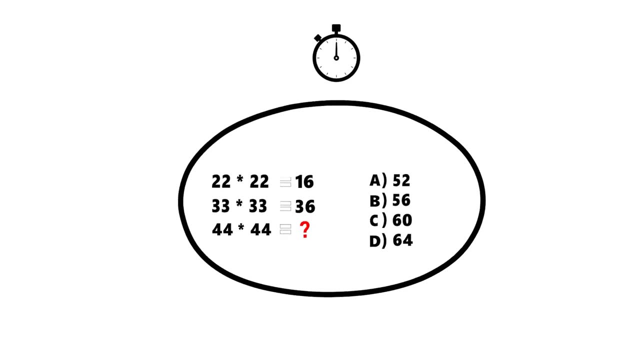 5 to 10 seconds, maybe 10 to 20 seconds, to see if you can come up with the solution, Ready or not. I am going to reveal the answer and we are going to get to the correct solution together. Typically to solve these types of problems, you need to identify the pattern. 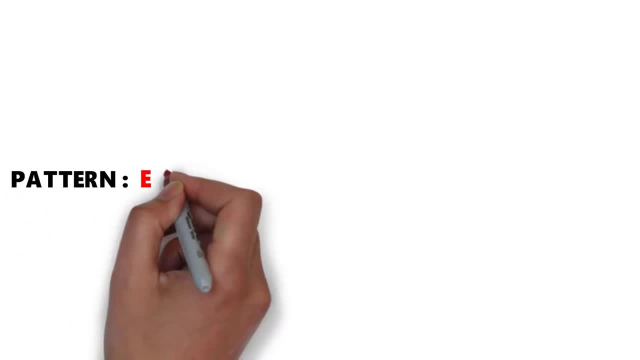 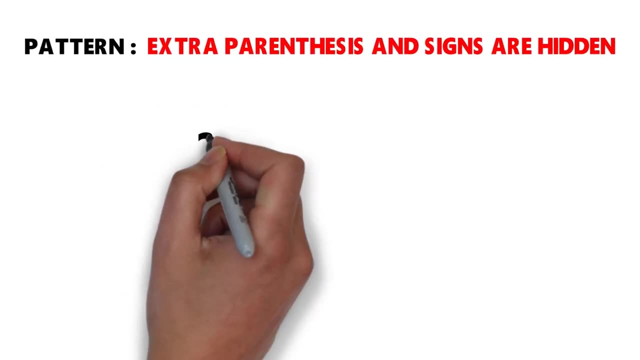 And in this particular case, the pattern is that the sign and parentheses are hidden in between digits and are not presented on the screen. Let's look at the first two examples: 22 multiplied by 22 equals 16.. It is not obvious because it doesn't go along with the rules of conventional 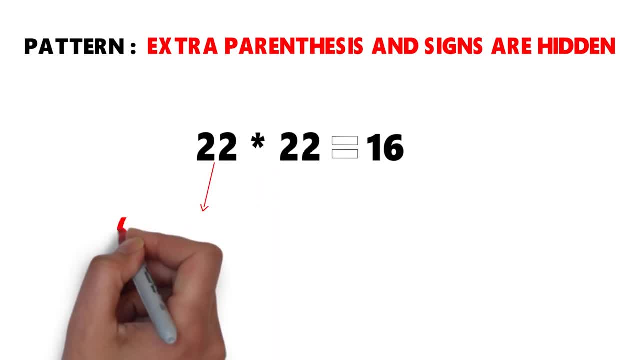 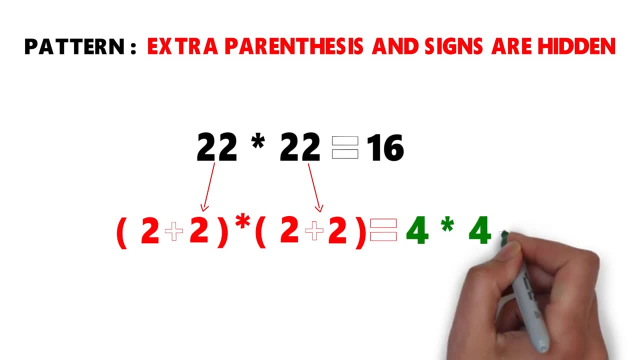 math. But if you add parentheses and in parentheses add 2 plus 2, multiplied another set in parentheses, 2 plus 2, you will be multiplying 4 by 4 and the result would be equal 16.. Same thing with 3 by 3.. 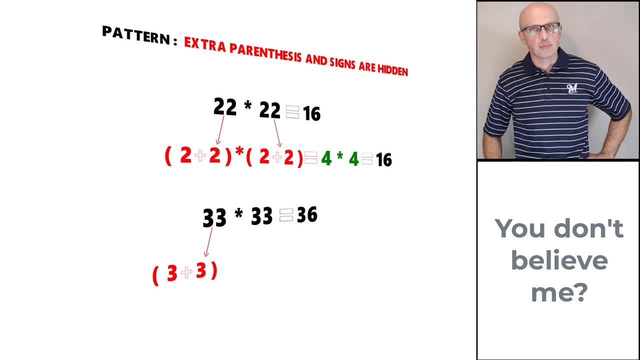 If you add in parentheses 3 plus 3 multiplied by another set in parentheses 3 plus 3, you will be multiplying 6 plus 6 and the result would be equal 16.. If you add in parentheses 3 plus 3 multiplied by another set in parentheses: